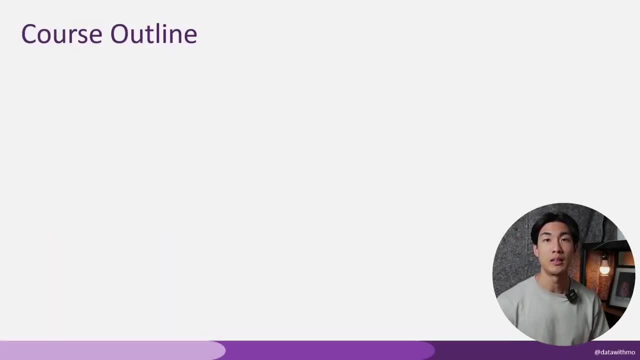 Okay, so first of all I created a simple course outline here so we can go through what exactly you'll be learning. So in the first two sections, in the databases, queries, tables and case sections- we're going to go through some theoretical knowledge first, 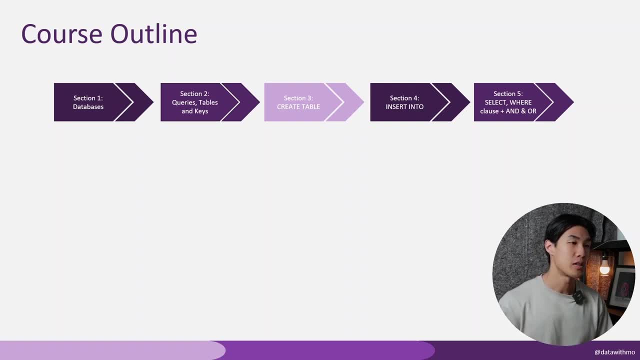 and then we move on to the hands-on bit. So in section three we'll create some tables, then in section four we're going to insert into these tables, Then in section five we're going to move on to some basic select statements. 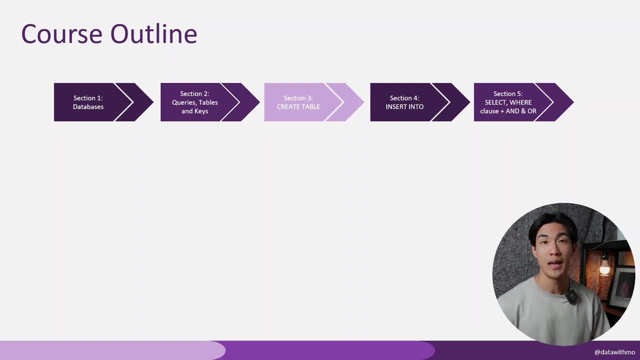 and we're also going to explore some where clauses with and and or. Now, moving on into section six, we're going to use the in, not in is no and between operators, And then in section seven, we move on to order by limit distinct. 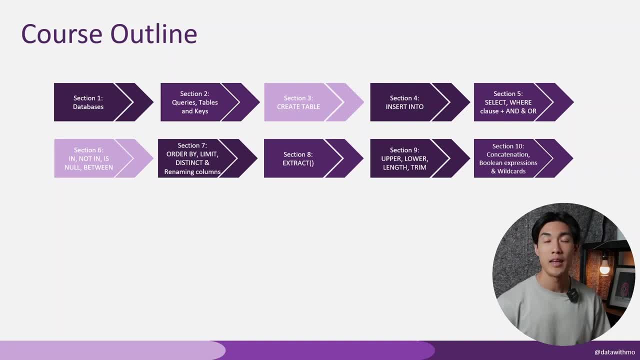 and we're also going to rename some columns. Then, in section eight, we're going to use the extract function to extract date information from the date columns, Of course, and then in section nine, we're going to move on to string manipulation. 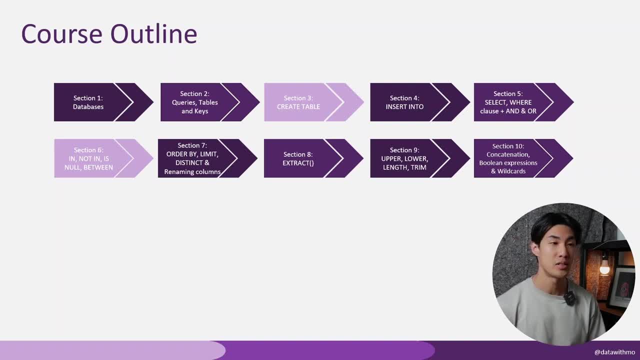 So we'll use the upper, lower, length and trim functions. Then, in section 10, we're going to use concatenation Boolean expressions and we're also going to introduce wildcards. So then, moving on to section 11, continuing on the theme of string manipulation, 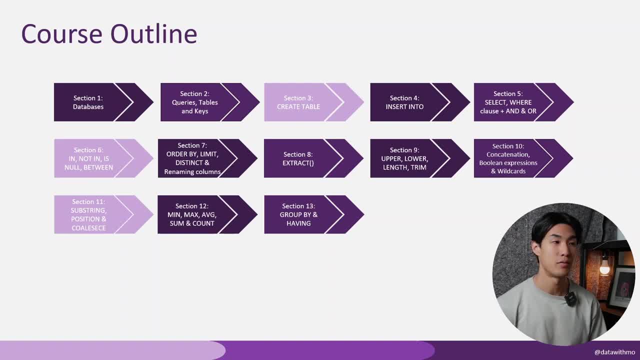 we're going to use the substring, position and coalesce functions And then we're going to to move on to some numerical functions, so we'll use the min, the max, the average, the sum and the count. Now, in section 13, we're going to use a group by and a special where statement the having. 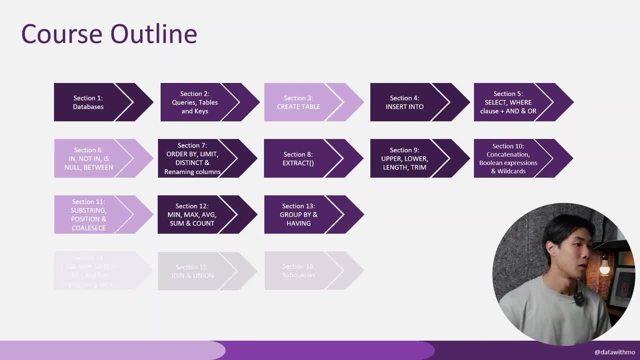 that you must use when you use group by. Now, moving on to section 14, we're going to use case statements and we're also going to combine case statements with the group by, and we're also going to use these case statements for transposing our data. Then, moving on to section 15, we're going to 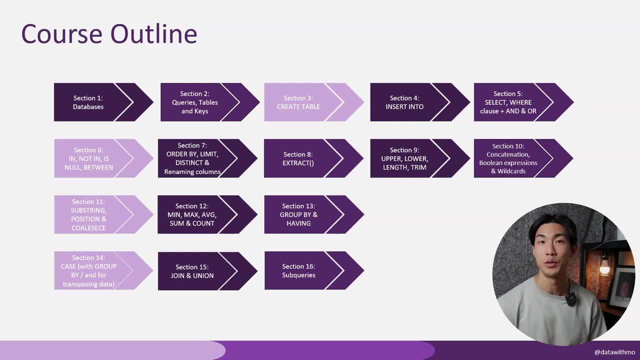 start working with multiple tables, using joins and unions, and then finally, in section 16, we're going to move on to something a little bit more complicated in the form of subqueries. So first of all, let's see what databases are, what a database management system is, 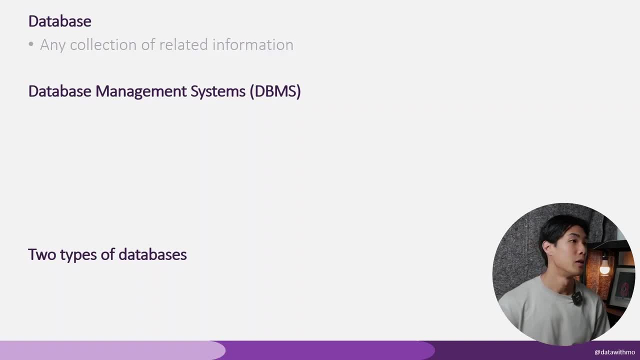 and what the two main types of databases are. So when you think of a database, just think of any collection of related information, and a database management system is essentially just a software application or software program that can help you create and maintain these databases. Now, crude is going to be. 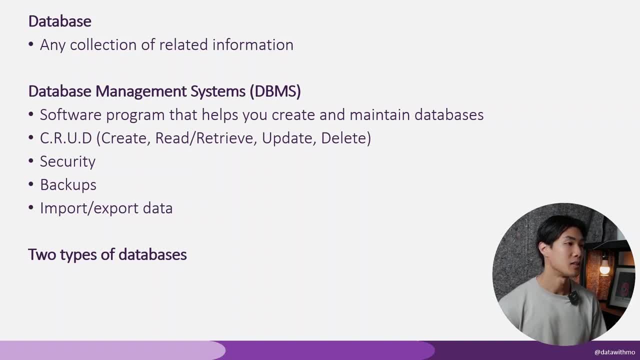 a very popular acronym that you may hear and it stands for create, read or retrieve, update and delete the main operations of a database, But obviously these databases can help you with security, backups, importing and exporting data as well. The two main types of databases are relational databases and non-relational databases. 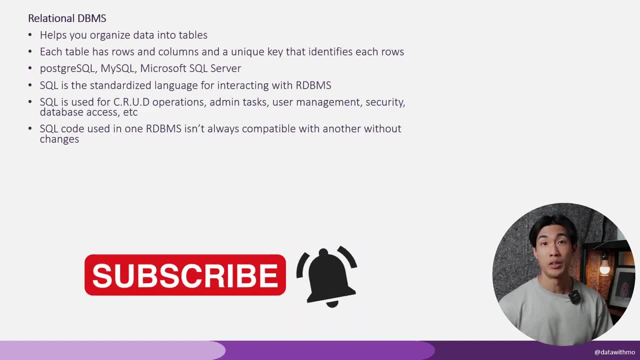 So first I'm going to cover relational database management systems, which is what this tutorial is on. So these can help you organize data into tables. Each table has rows and columns, pretty much like a spreadsheet. So some popular ones would be postgres, sql, which is what I'll cover in this tutorial. 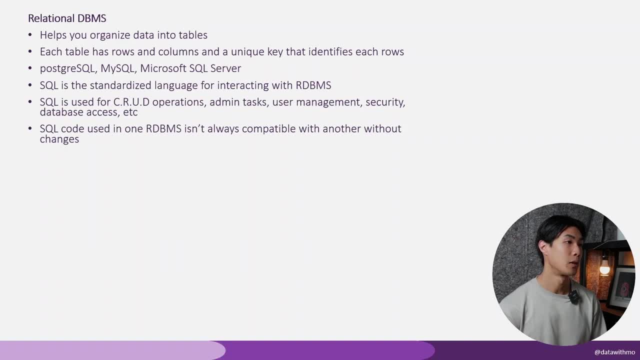 or mysql or microsoft sql server. Now sql is the standardized language for interacting with relational databases. So sql is used for all database management systems, or rdbms, and it stands for structured query language. sql is used for crude operations: admin tasks, backups, security, user management. 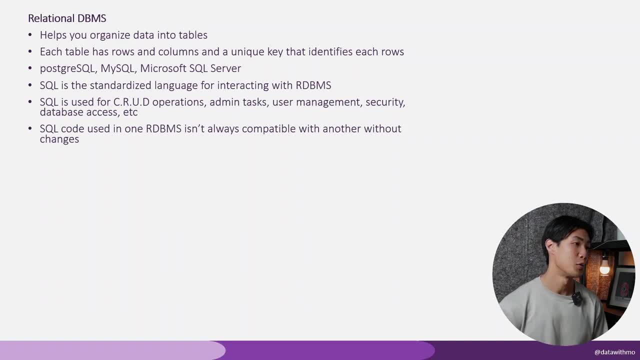 database access, so on and so forth. So sql code used in one rdbms may not always be transferable to another one, but given that they're so similar- say, for example, if you can code in postgres sql, you'll be able to code in mysql as well. 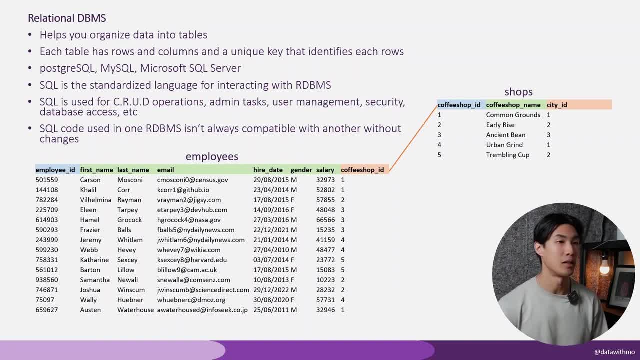 Let's quickly look at two tables here. I have the employees table on the left and then the shops table on the right. You can see that within the employees table we have the employee id column, which is the unique identifier. So if I look at the first row here, employee id 501 559, this employee id uniquely identifies. 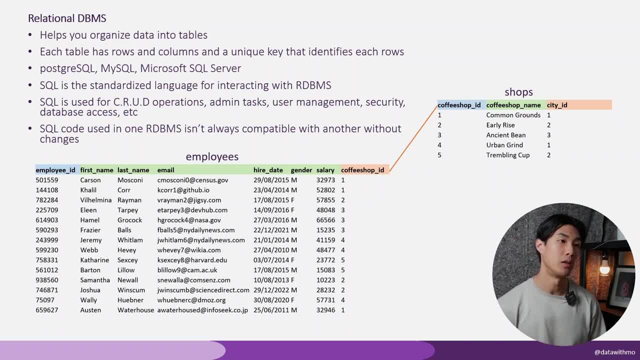 Carson Mosconi. If I look at the shops table on the right, you can see that the coffee shop id is the unique identifier. So if I look at coffee shop id 1, this is going to uniquely identify the coffee shop with the coffee shop name common grounds. 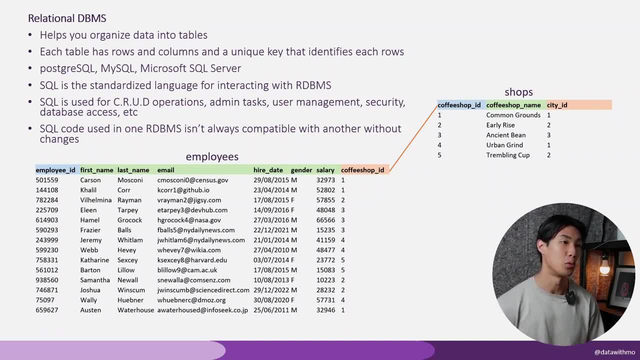 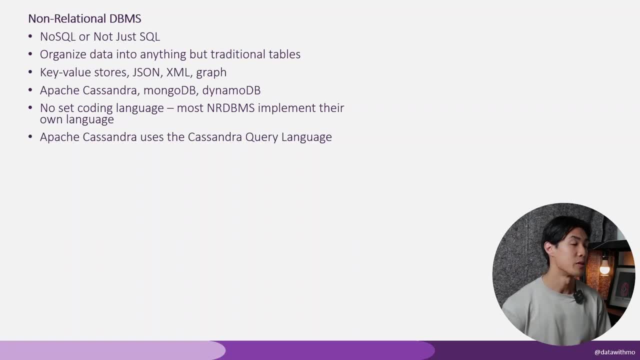 Now you can see that both of these tables are organized into rows and columns, much like a spreadsheet. So, moving on to non-relational database management systems, which stand for no sql or not just sql, You can organize data into anything but traditional tables, so think. 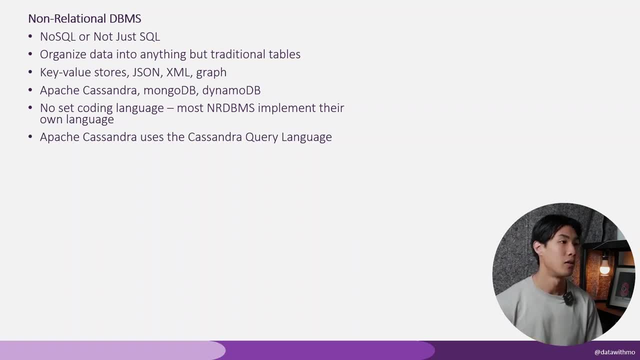 of key value stores json's, xml's graph. Some popular ones would be a Apache Cassandra, MongoDB or DynamoDB. There is no set coding language, so most non-relational database management systems they implement their own language. Apache Cassandra, for example, uses 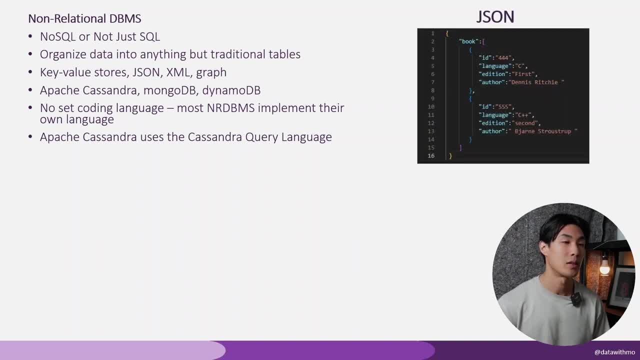 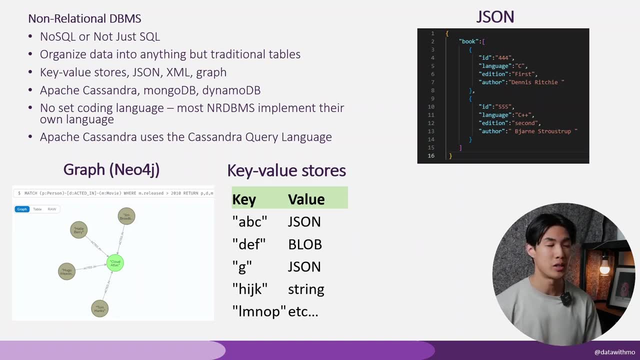 the Cassandra query language. So let's quickly look at some examples. you see a json file here, and then we have a graph database on the left- it's actually a Neo4j database, which is quite popular- and then we see some key value stores as well. So let's move on to queries. 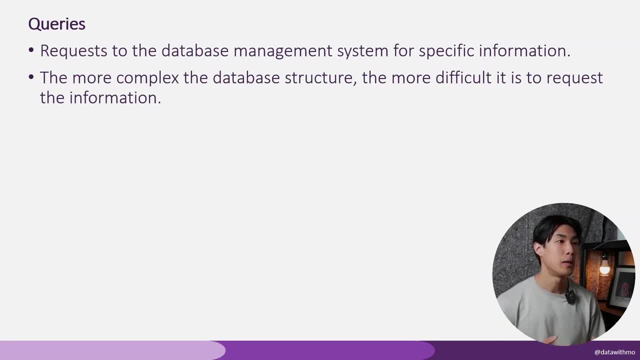 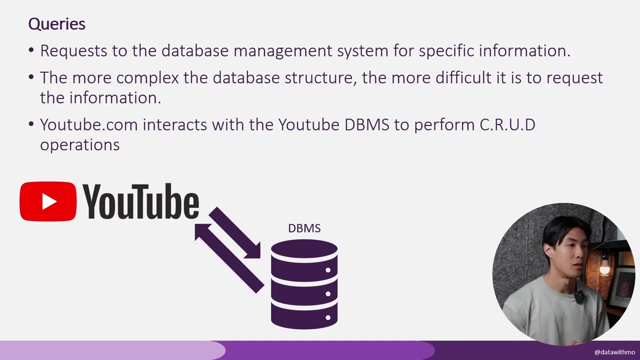 And queries are essentially just requests made to the database management system for specific information that you want to retrieve. So the more complex the database structure, the more difficult it is to request this information. So I created a very simple illustration here of a youtube database management system. Now, clearly I don't work at youtube and the formula is much more. 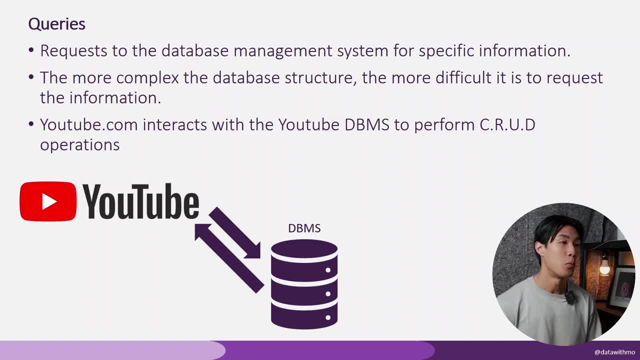 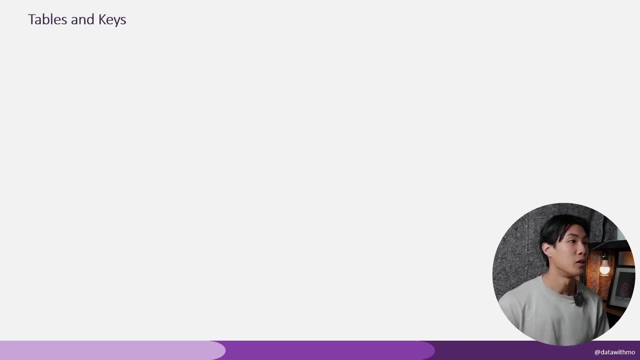 complicated than this, but at its very core. when you interact with youtubecom, youtubecom then in turn interacts with the youtube database management system to perform crude operations. and it's that simple at its core, obviously. So let's move on to tables and keys. So, like I, 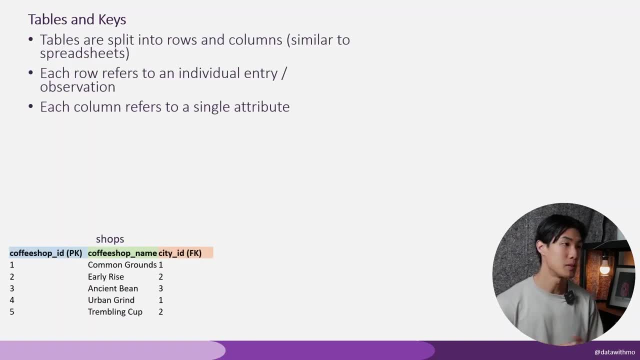 mentioned before, tables are split into rows and columns. Each row refers to an individual entry, a single observation, and then each column refers to a single attribute. So if we look at the shops table here on the bottom left, you can see that the coffee shop id column is a single. 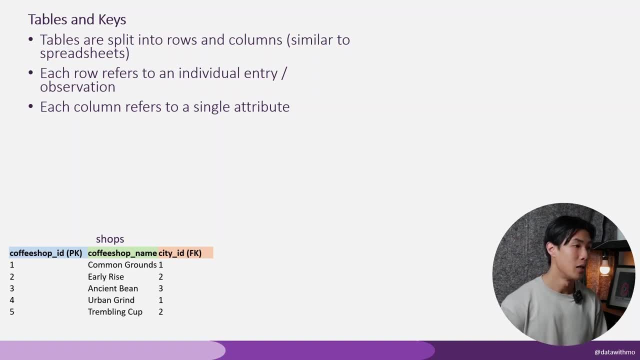 attribute and obviously it'll refer to the coffee shop id. You can see that the table is organized into rows and columns. so the first row would contain coffee shop id 1, coffee shop name, common grounds and city id 1.. Now these tables must have a primary key, so this is a special column. 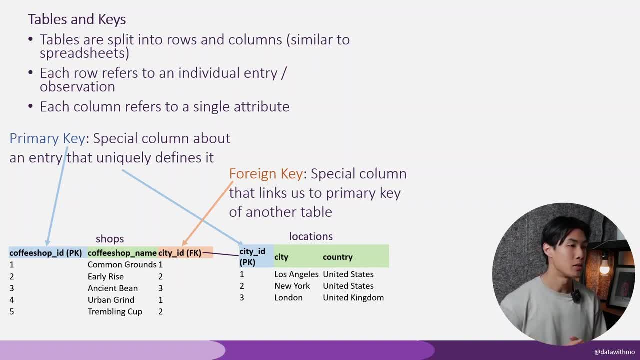 about an entry that uniquely identifies it. So if we look at the shops table, this special column is going to be the coffee shop id, which will uniquely identify each row within this table, and then the locations table on the right, the city id will be the primary key which will 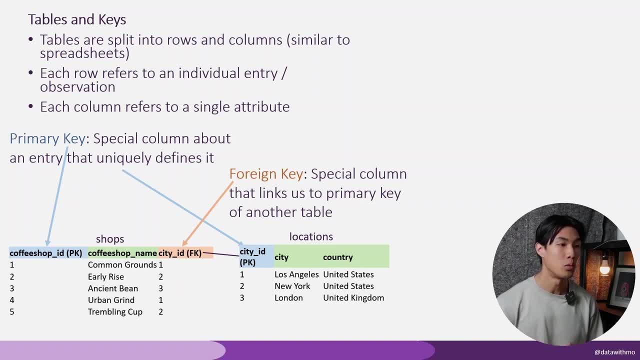 uniquely identify each row. So city id 1 will uniquely identify the city of Los Angeles in the united states and city id 2 will uniquely identify the city of new york, also in the united states. Now tables may have foreign keys, so this is not a must. Foreign key is a special column. 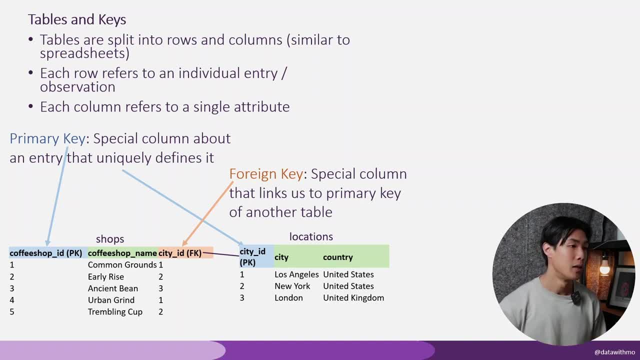 that can link you to the primary key of another table. So if we look at the city id column in the shops table, this is a foreign key because it links us to the primary key of the locations table. So city id foreign key in the shops table links us to the 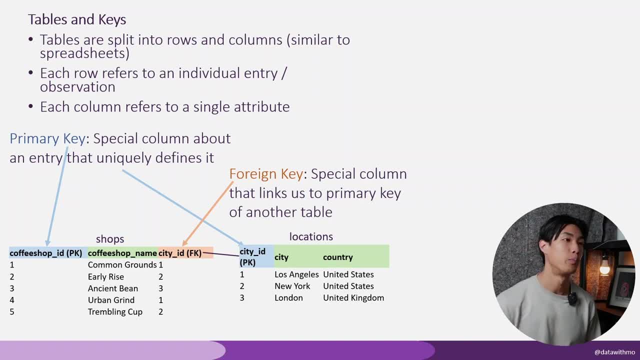 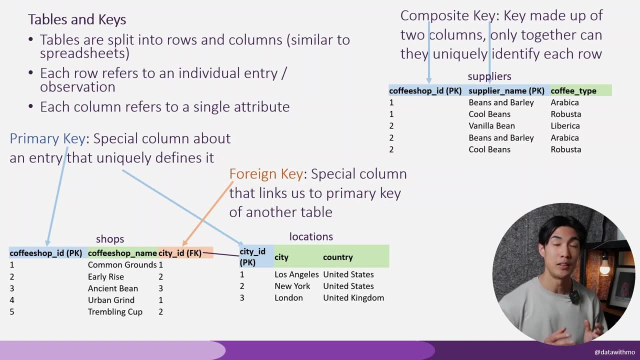 city id, primary key in the locations table. Now, tables may sometimes also have composite keys, so these are keys made up of two columns and only together can they uniquely identify each row. So let's quickly have a look at the suppliers table. on the top right You can see that the coffee shop id and the supplier name. 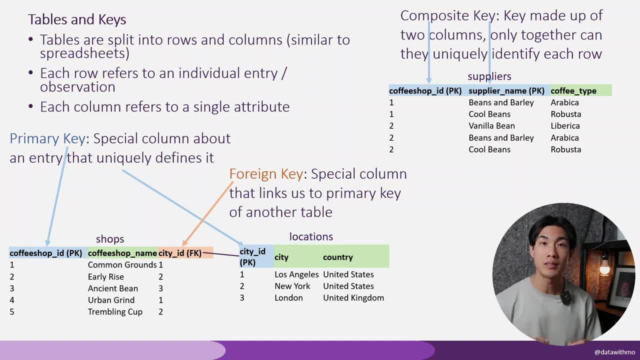 they make up the primary key together, because only together can they uniquely identify each row. We need to know which coffee shop the supplier supplies into and obviously we need to know which supplier is actually the coffee type supplier. So if we look at the supplier name, 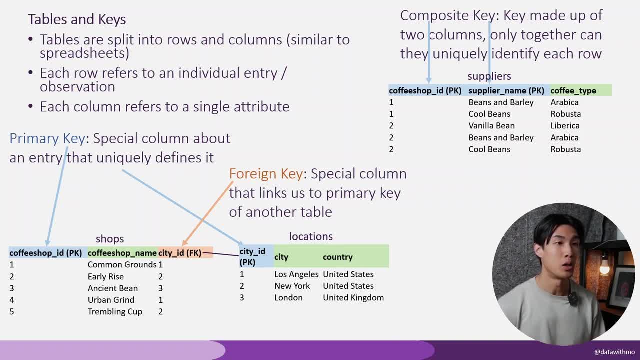 column only there's two entries for beans and barley. If we didn't have the coffee shop id column, we would have no clue who supplies the product, but we would have no clue which store the supplier actually supplies this product to, and that is exactly why we need a composite key here. 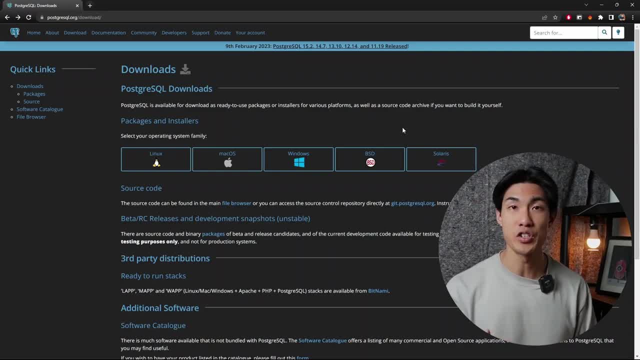 All right. so now I'll show you how you can easily install the pgadmin tool, which will be a PostgreSQL tool, on windows. So the download link is in the description below. so it's just this postgreSQLorg download link and make sure you obviously choose windows because you want to. 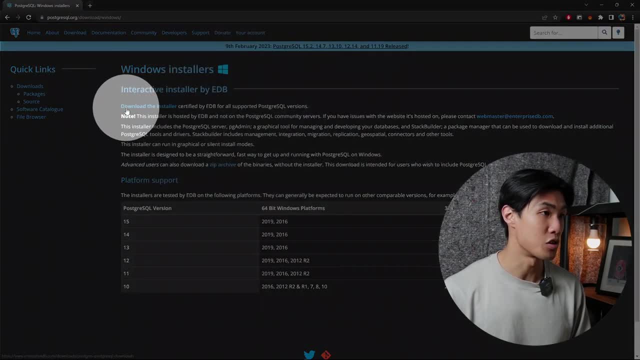 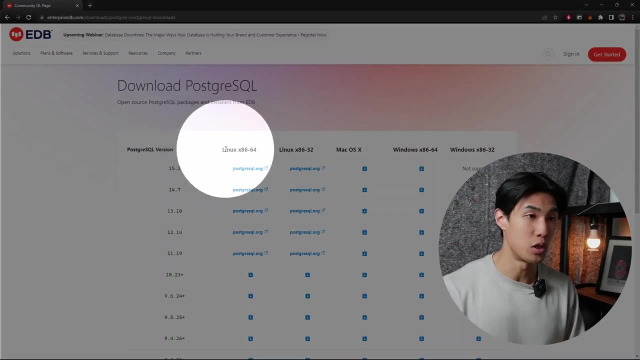 install it on windows and then from here you can easily install the pgadmin tool. and then you can here: the easiest way is just to click on download the installer. so once you do that, it'll take you to this page where you can choose between various environments. so what you want to do is you want? 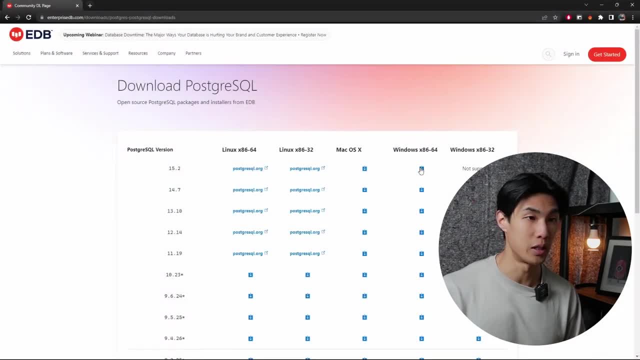 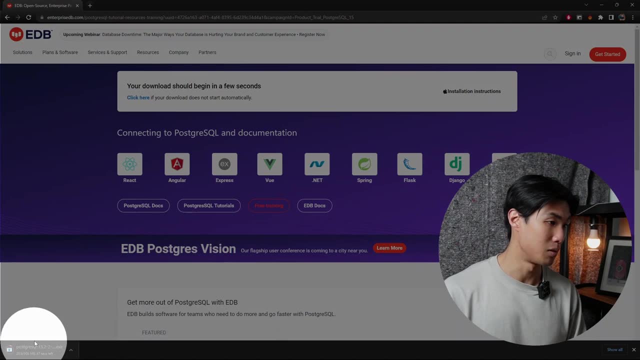 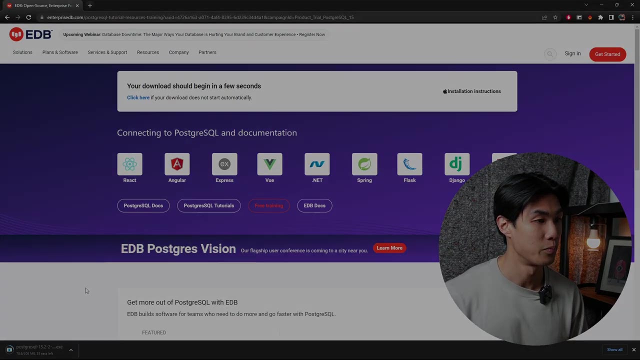 to choose the windows x86 64 operating system here and then click the download button. so your download should start now. so you can see that mine is actually in the bottom left here. so overall it's 305 megabytes, so i am just going to wait for the download to finish. okay, so once your download, 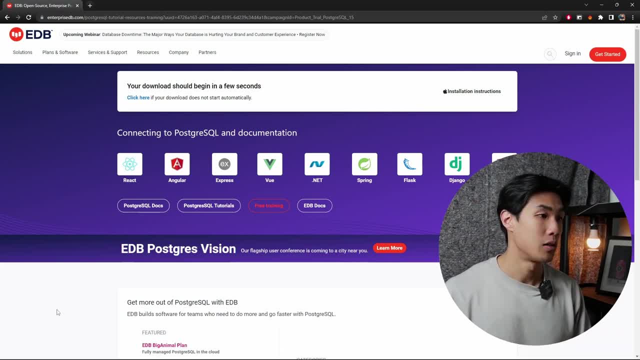 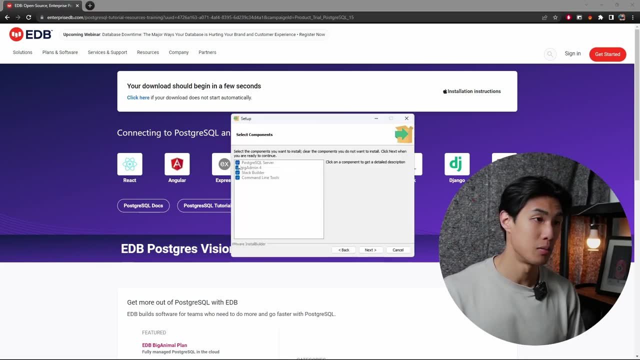 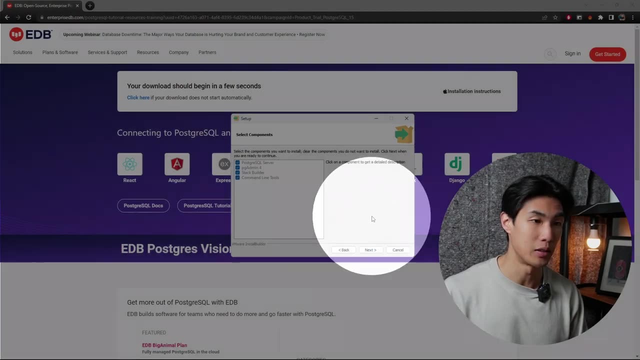 is done. make sure you just click the installer here and then let's start installing the postgres sql tool and then, when you're in the setup wizard, just hit next. make sure you install all of these so we'll have the postgres sql server right here. pgadmin4, stack builder and command line tools. 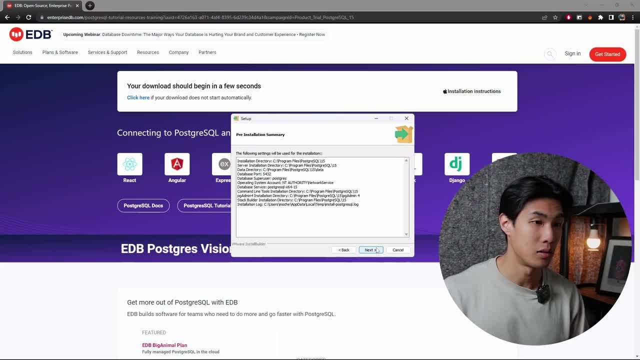 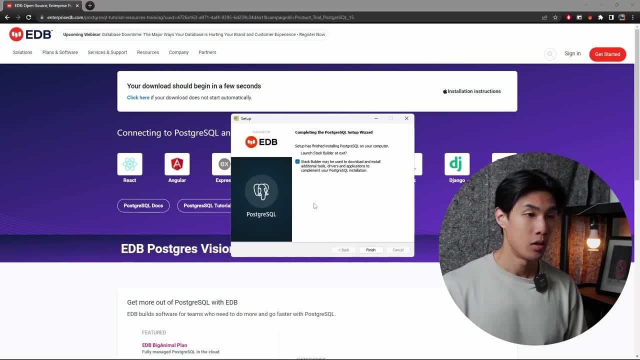 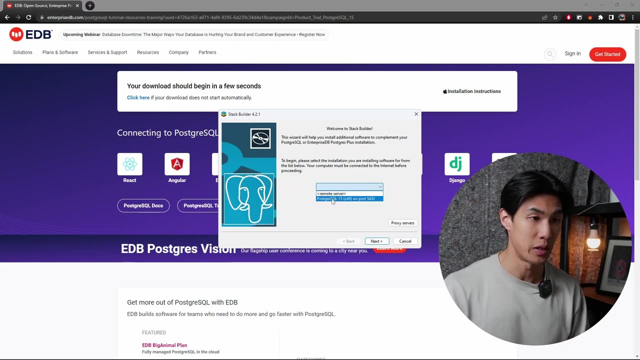 and then hit next, next, next, um, yep, next, everything is default. hit next, okay, so that's it. make sure you just hit next, hit finish at the end and then for the servers, just choose the one that comes by default. so this is going to be on port 5432. hit next and then from the application list: um, we need, i think yeah. 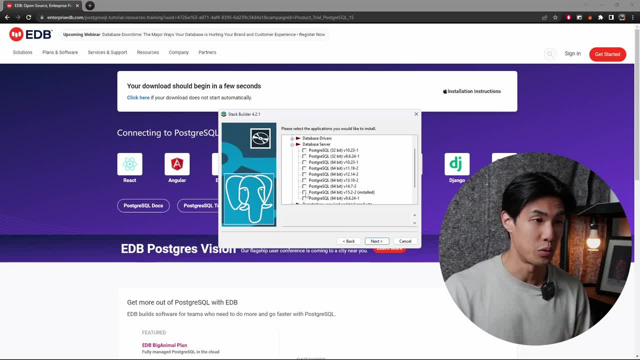 we do need to select something, so i think i'm just going to select the one that's already installed. so this one, hit next, hit next and then skip the installation, hit next and then finish, and now you have your pgadmin tool installed. so now, if i go into the 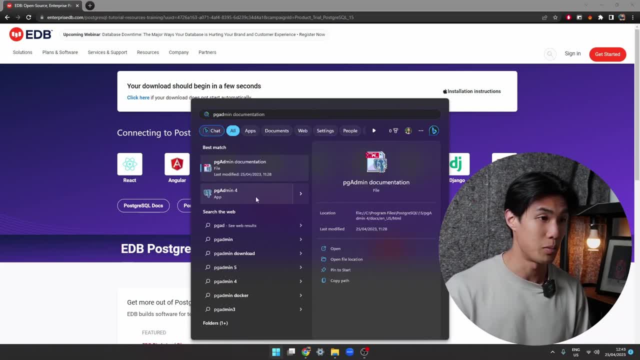 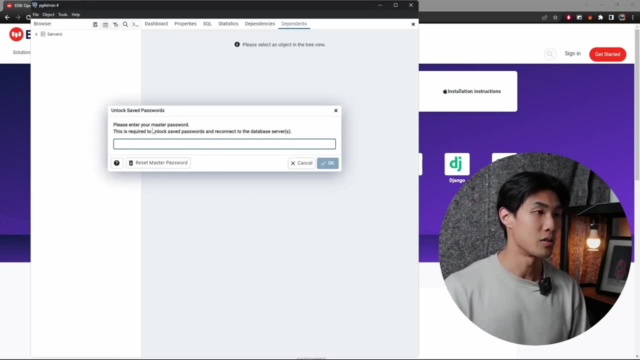 start menu and i type in pgadmin. you see here that i have the pgadmin tool right here, so you can just click on it and then it'll start up. so once it's started up for the first time you will have to provide a master password. obviously, just go with something that you'll remember. and then the moment. 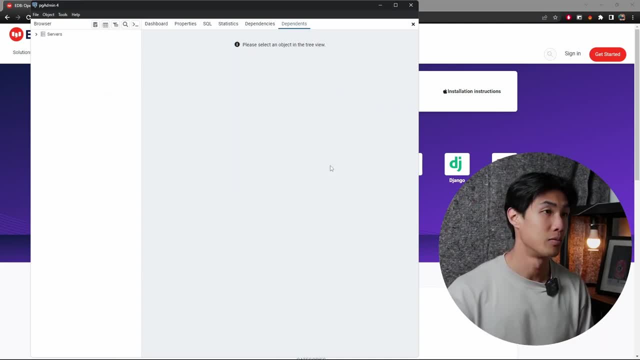 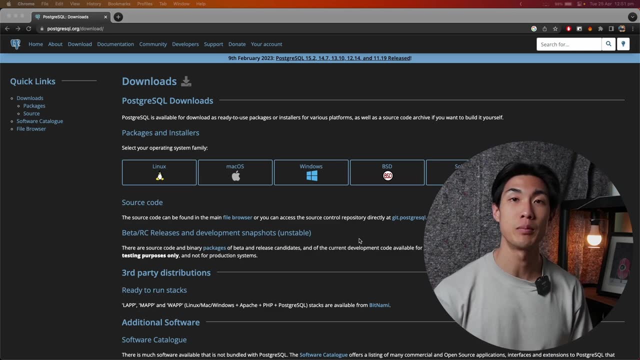 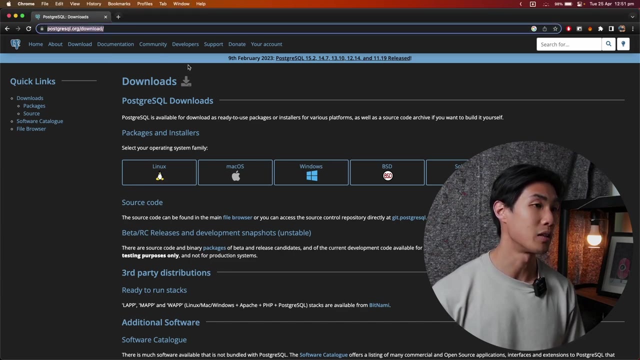 you hit ok, you have everything set up, so that's it okay. so now i am going to show you how you can easily install the pgadmin tool, which will be your tool if you have a mac. so just make sure that you go to this website here. link is in the description. 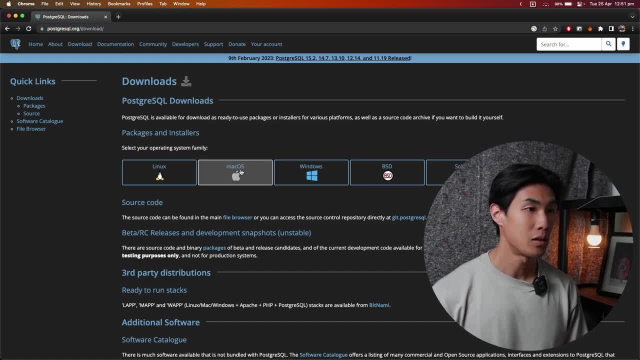 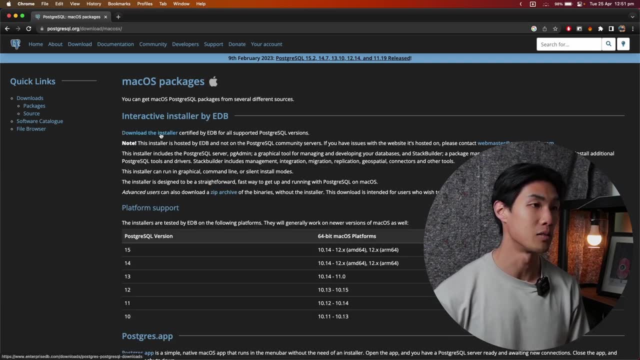 below. so postgresqlorg download and then obviously after that make sure just to click on mac os, and then the easiest way to install this one is to go to download the installer at the top left here and then click on it and then you get taken to this page and then make. 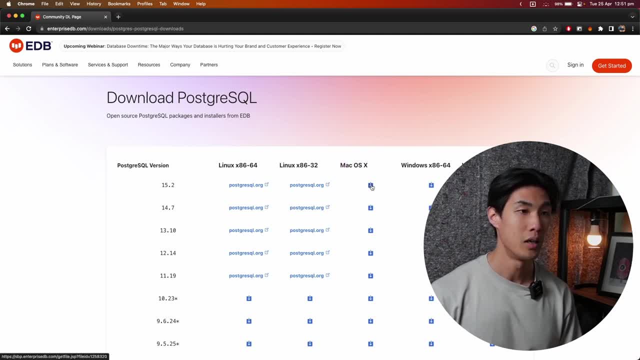 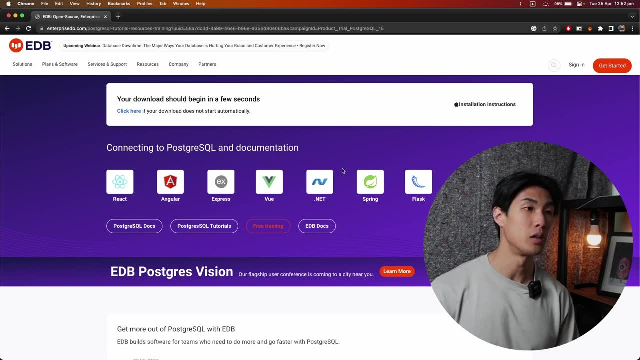 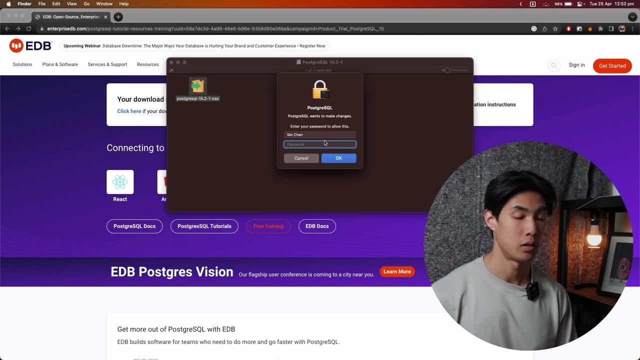 sure, obviously you select the mac os installer, hit the download button and then wait for the download to finish, all right. so once your download is done, make sure you click on the installation file and then click on this installation file, double click on it, hit open and then obviously just type in your system. 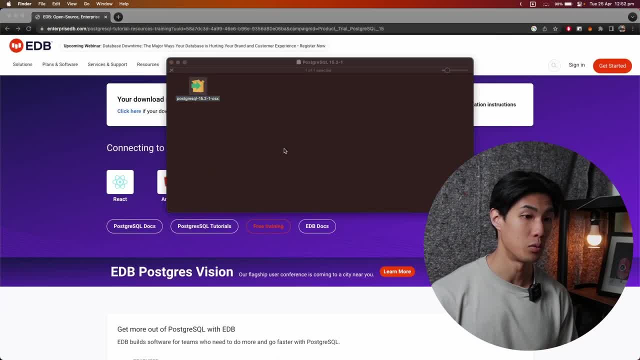 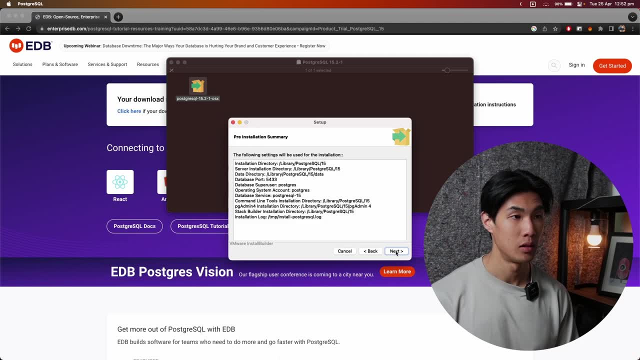 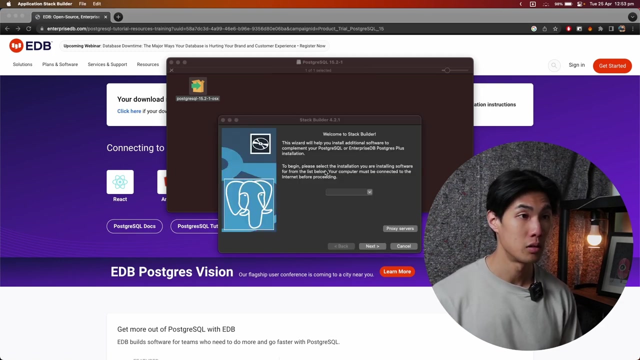 password, and then you can just install whatever you have. so let the installer begin: hit next, hit next, hit next again, next, again, next, again, next, and then sit back and wait for the installation to come in complete. okay, so once your installation is done, hit finish, type in your password again and then 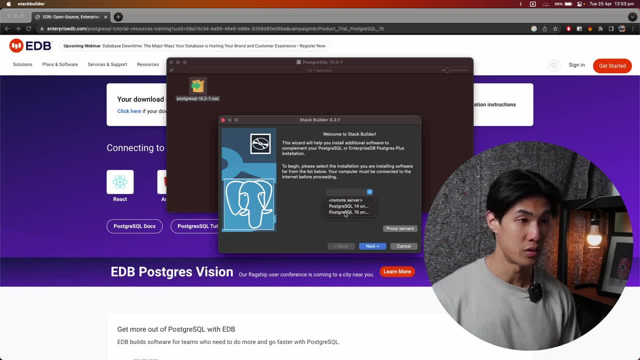 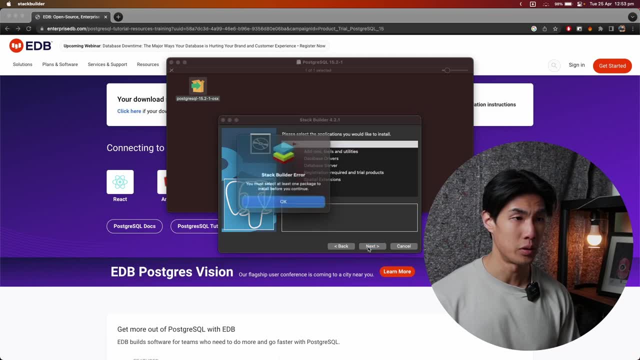 from here. just make sure you choose the whatever server you get given. so i'll go with postgresql 15, because it's the latest, hit next. and then i think we need to install something. yes, okay, so let me just select the server that i just chose from here. so 15.2, hit next, hit next. again, nice. 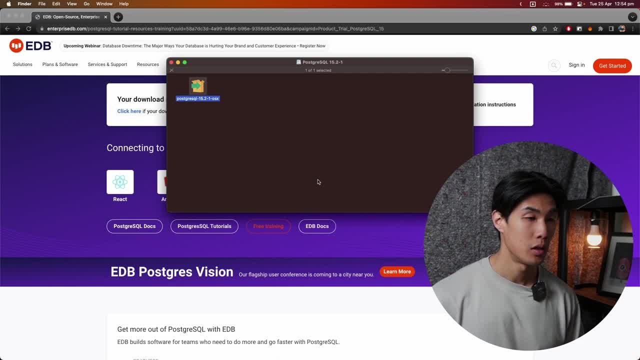 that. skip installation, hit next, hit, finish and then that's it. now you have the pg admin tool. so if i just search for it, you can see that i have it here. we can open it up, okay, so when you start it for the first time, you will have to enter a master password. obviously, just go for something. 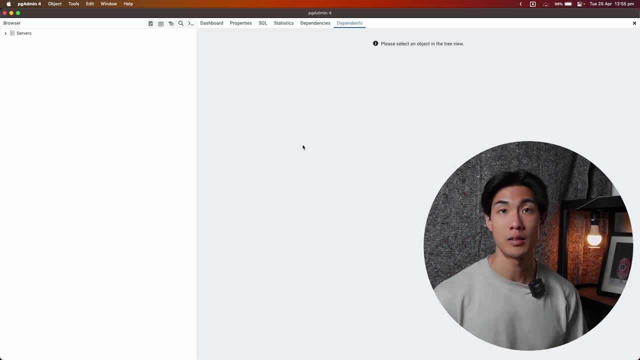 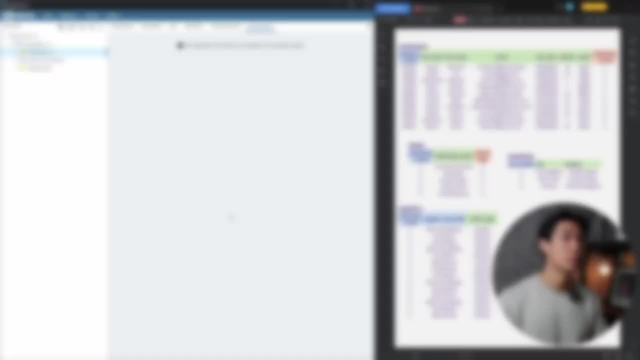 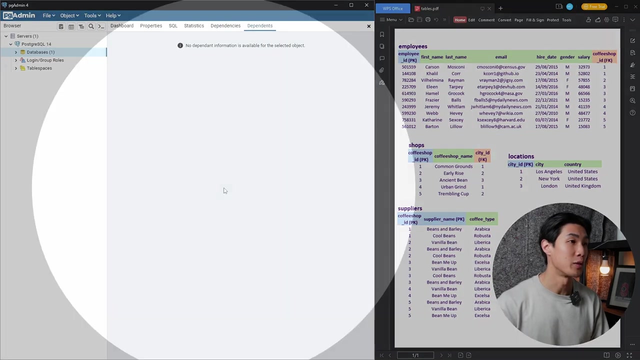 that you don't forget, so you can reuse it. and then that's it. you've installed pg admin tool, the postgresql tool which you will be using in this tutorial on your Mac. okay, so now that we have everything installed, let's jump into the exercise. and first of all, you can see that I have pg admin. 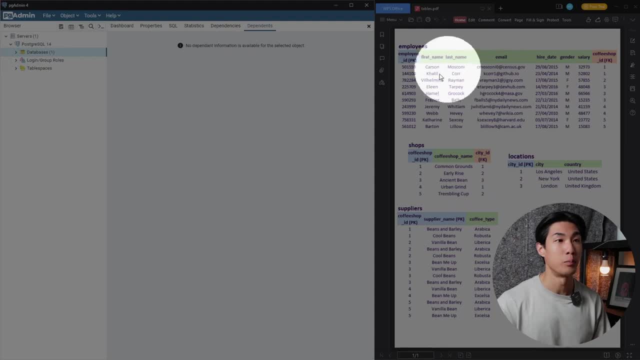 so the postgresql tool open on the left here and I'm going to have the tables open on the right, just so you can see what kind of data we're working with. so just to go through the tables, we have the employees table, at the top, we have the shops table, the locations table and then we also 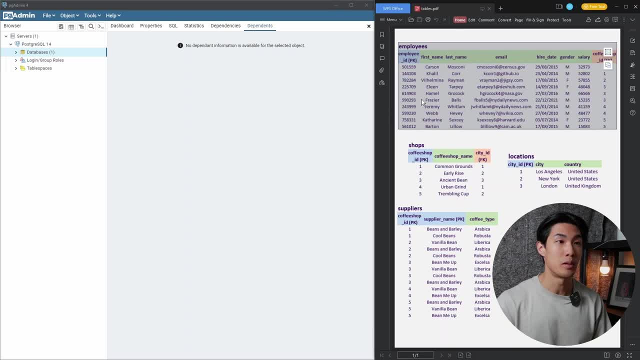 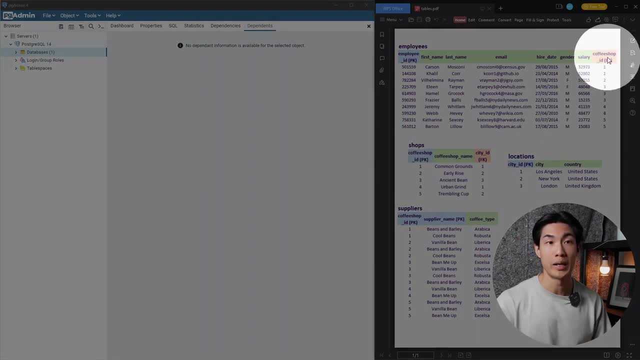 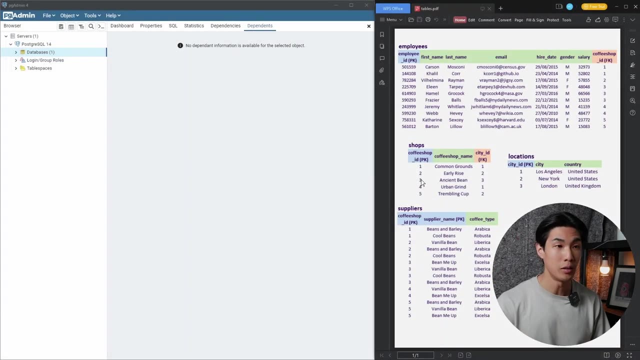 have the suppliers table. within the employees table, you can see that the primary key is the employee ID column, and then within this table, we actually have the foreign key, the coffee shop ID column, which links us to the primary key of the shops table, where the primary key is the coffee shop ID column, and within the shops table you can see that we also 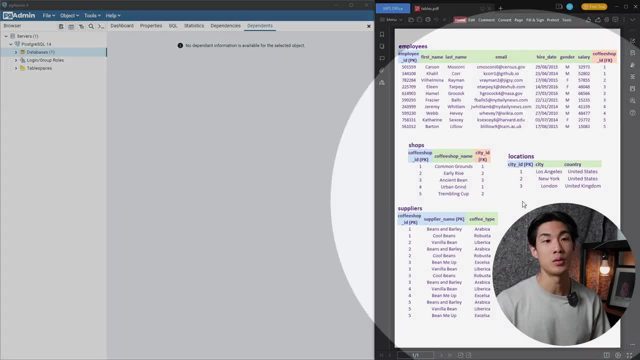 have the city ID as a foreign key, which links us to the primary key of the locations table here, and then, finally, we have our suppliers table with the composite key. so you can see that the coffee shop ID is the primary key, which is also a foreign key because it also links us to the shops table, and 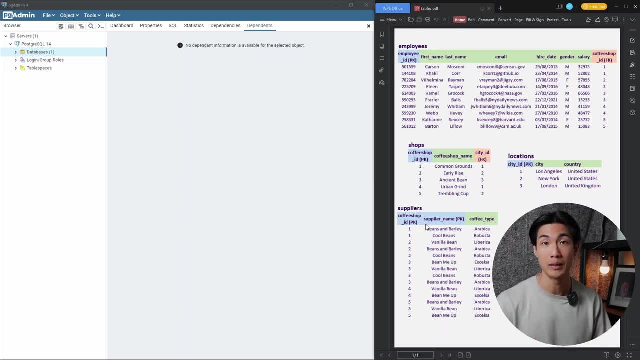 the supplier name, the other primary key. so these two combined they uniquely identify each row within this table. all right, so a quick tour of our pg admin tool here. so let me just click into databases here and you can see. by default, pg admin comes with the postgres database, so we're gonna create. 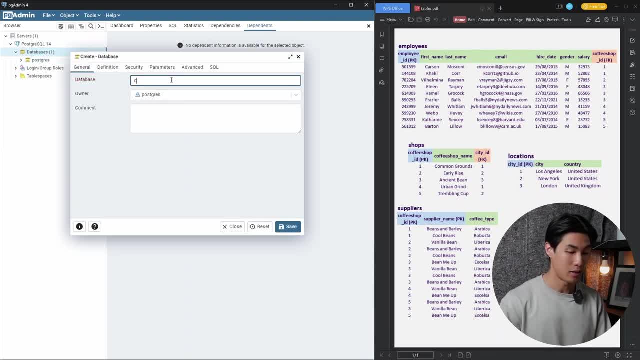 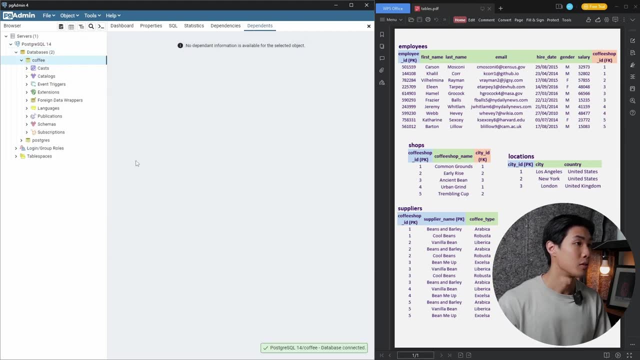 our own database. by right clicking create database and I will just call this database coffee. you can leave the owner as postgres and save. so now that we've created our database, you can see that coffee appeared here. let's go into schemas. so you see that you have a bunch of options here, but the ones we're really going to be interested in. 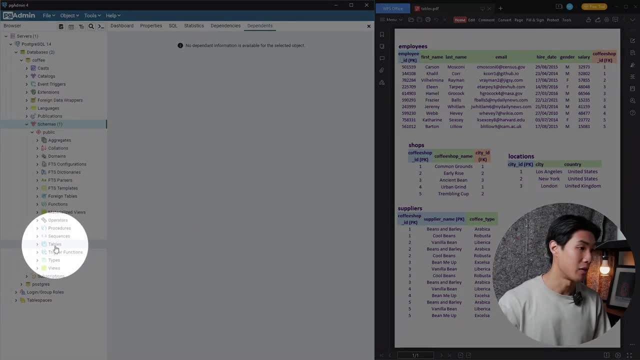 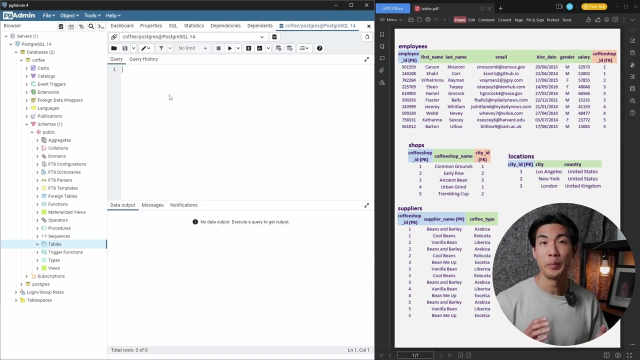 this course will be schemas, and then under schemas we have tables. so if you click into it you can see that at the moment I don't have any tables, which makes a lot of sense because obviously we haven't created anything yet. so let's go to the top and open the query tool. so I won't be typing out any. 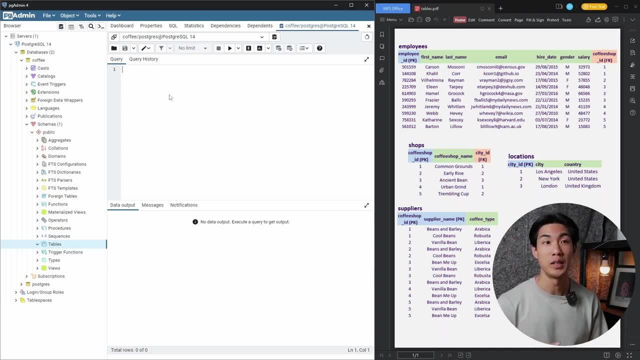 code. really, in this tutorial I'm just going to copy and paste the code in. you can do the same, obviously, using the link below where you can find the code. so first of all let's create some tables. so I'm going to copy and paste in the first two queries and first of all we're going to create the employees. 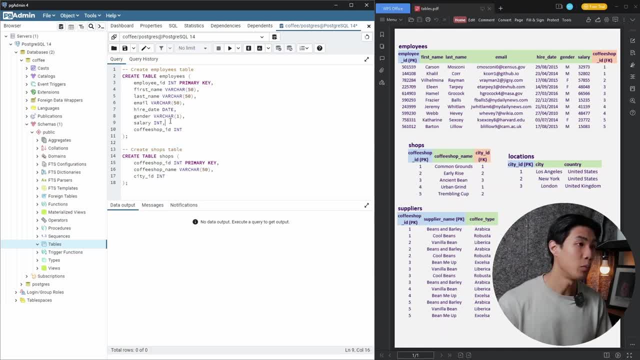 table and then we're going to create the shops table. so create table is the keyword for creating tables, obviously- and then you pass in whatever table name you want- in this case we'll call this because it'll store employee data- and then we need to put in the column names, so we specify them as: 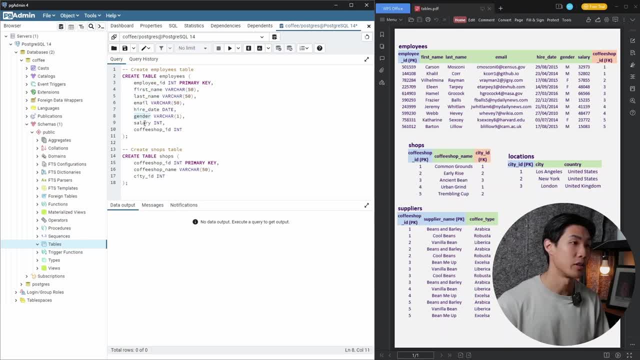 employee ID: first name, last name, email, higher date, gender, salary and coffee shop ID. now, next, we need to define the data type. so employee ID will be of integer data type: first name, last name, and email will be varchar 50 and 50 just refers to the length, the maximum length of the characters. 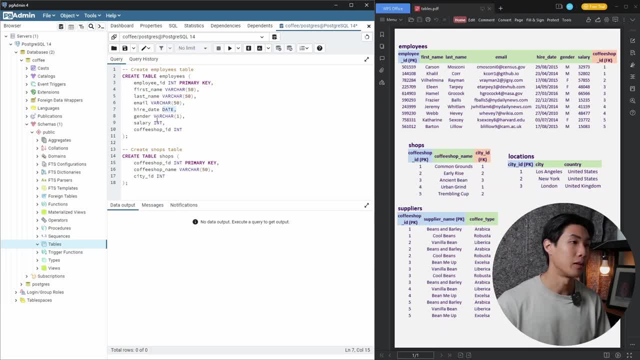 and then higher date will obviously be of date data type. the gender will be a varchar one, so a character length of one, because it's either going to be male, so M, or female. now, salary again will be of integer data type, and then we have coffee shop ID, which will also be of integer data. 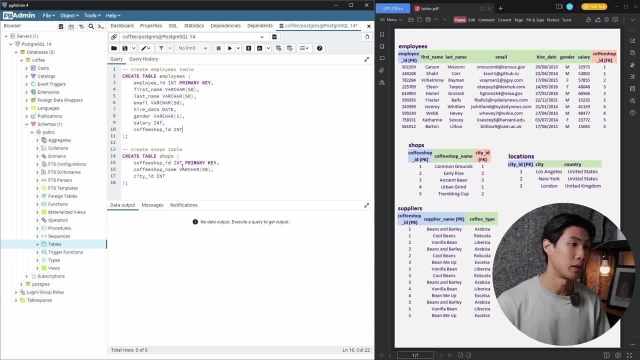 type. so we're going to create this table and then we're going to create the shops table where again you pass in the column names, so coffee shop ID, coffee shop name and city ID, and then you need to pass in the data type, which is integer, and then varchar 50 for the coffee shop name and integer. 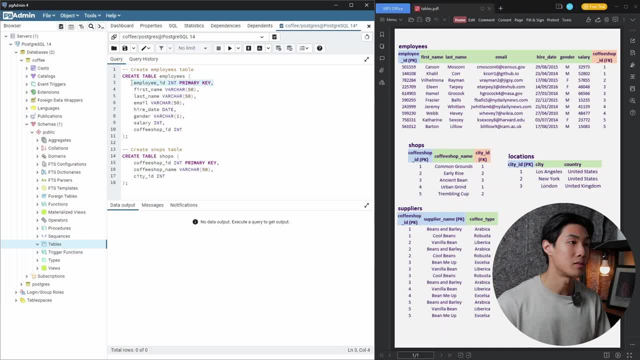 for the city ID here, that in the employees table the employee ID is the primary key, so we define it by passing in the primary key keywords. and then in the shops table you can see that the coffee shop ID will be the primary key. so we define this as the primary key here. so let me just run all of this. 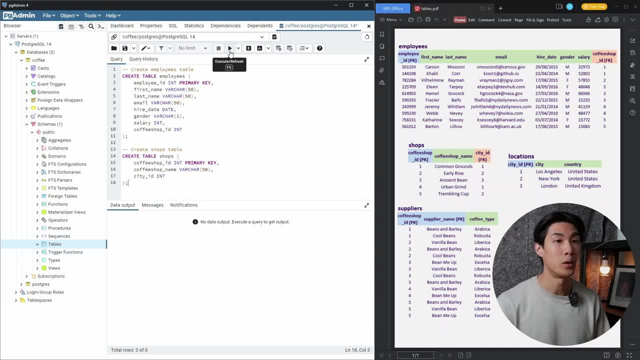 code and you can hit the little play button at the very top, or you can hit F5 and there we go. the query ran successfully. you can see it on the bottom here. it says: query returned successfully in 83 milliseconds. all right, so that's all good, let's move on. so I'm sure you noticed that we didn't do anything. 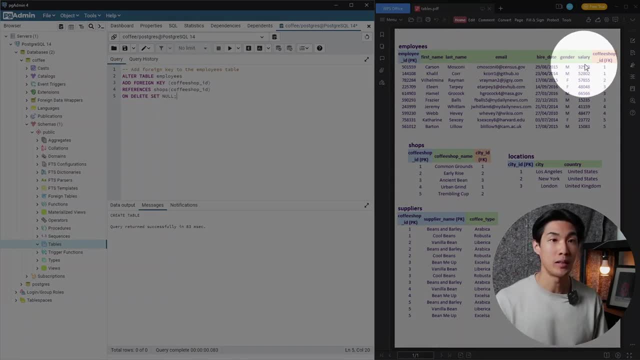 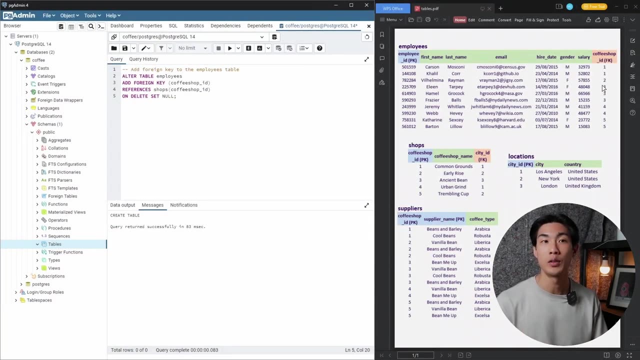 about the foreign key before. so let me just go to the tables here on the right and you can see in the employees table that we have the coffee shop ID as the foreign key. but I didn't actually define this now. why didn't I do that now? this is because I couldn't define it here, because I haven't. actually created anything in the shops table yet, so I cannot define a foreign key that links to the primary key of a table that doesn't exist yet. so that's why let's go back into our admin tool here, and now that we have the employees table and the shops table, I am going to add the 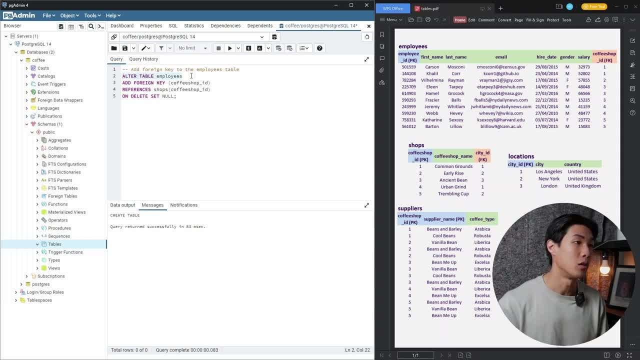 foreign key on the coffee shop ID. so the keywords are alter table. which table you want to alter the employees table? add the foreign key on which column- the coffee shop ID column in the employees table. what does it reference? so you say references the coffee shop ID column in the shops table and 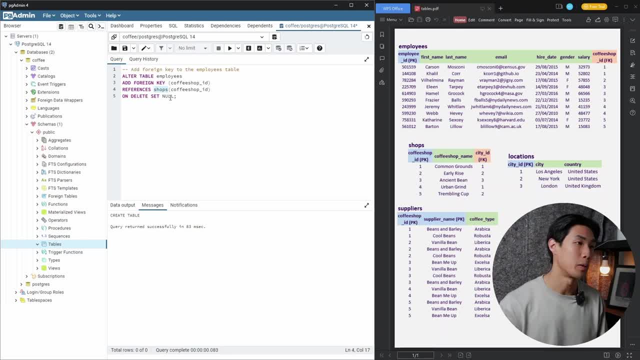 then on delete set: no, this is just a constraint and for the purposes of this course I won't go into constraints in too much detail for now. just go with on delete set no, and let me just run this code and you can see again that the query was returned successfully. so we've added our foreign. 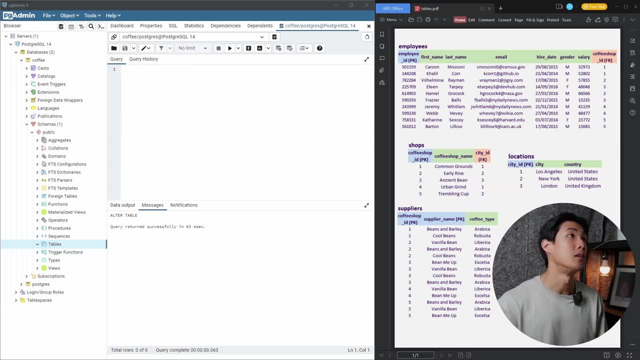 key. okay, so next up, we're going to create the locations table and then we're also going to add a foreign key to the shops table and then create the suppliers table. so you can see the code here: first of all we need to create the locations table. so again, create table. what table name? locations. 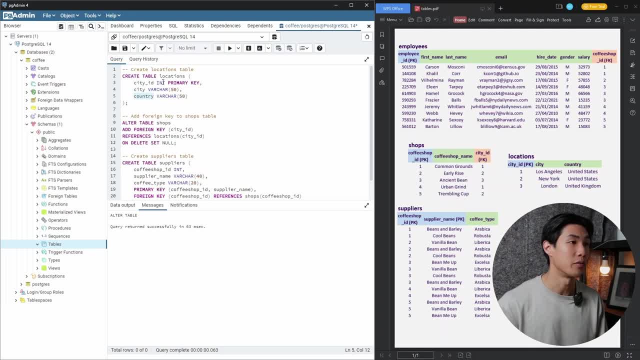 you pass in the column names city ID, city and country. you define the data type integer varchar50 and varchar50 again, and then you set the city ID column as the primary key and you notice here that we're going to add the foreign key to the shops table now. so let's just go to the tables and right. 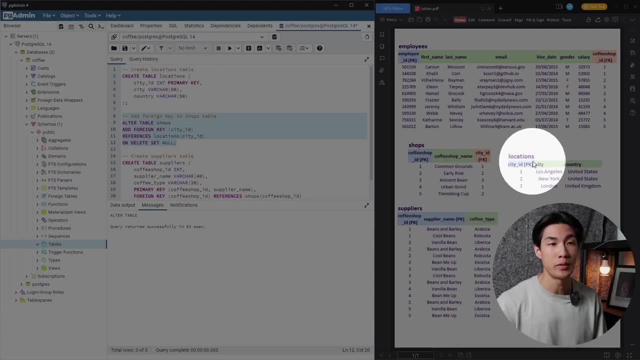 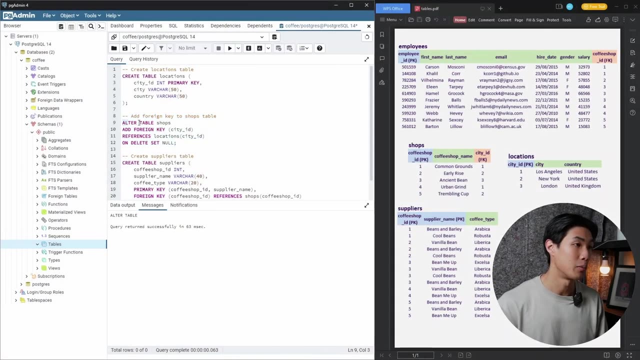 here you can see that city ID is a foreign key here and once we've created the locations table we can link the city ID to the primary key of the locations table. so alter table shops. add the foreign key to the city ID column. references the city ID in the locations table. and again on delete set no. 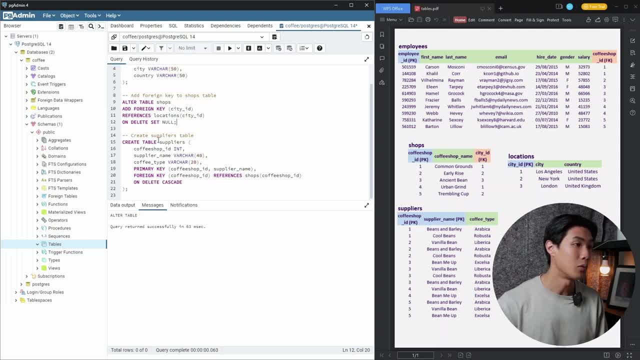 and then we can run that as well, and then, finally, we're going to create the suppliers table. so this is the one with a composite primary key. so create table what the table name is: suppliers columns, coffee shop ID. supplier name and coffee type, and then coffee shop IDs of integer data type and then 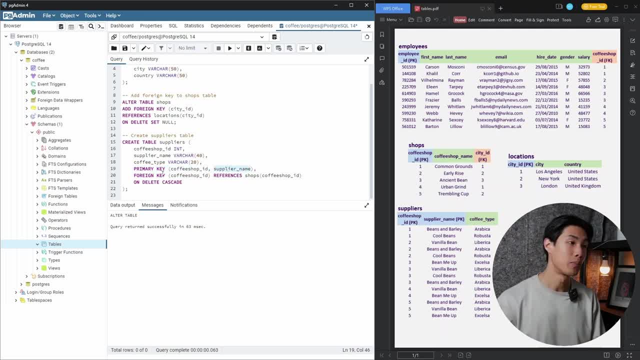 the coffee shop ID and supplier name. so we have a composite key. and then the coffee shop ID is also a foreign key, so let's not forget that- and it links to the coffee shop ID column of the shops table. and then here we set on delete Cascade again for the purposes of this tutorial. just. 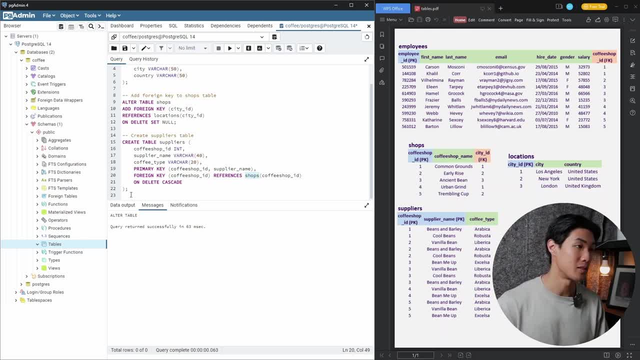 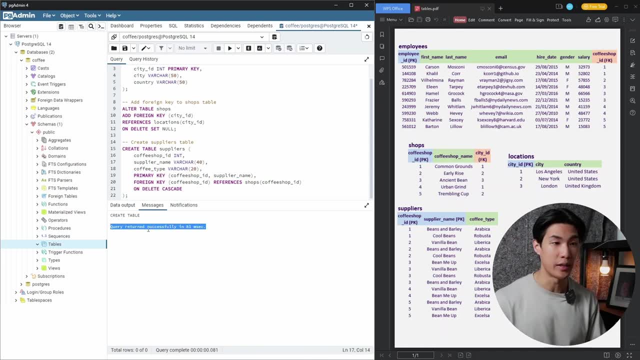 set it like this. I won't go into too much detail about constraints now- so we can go ahead and run this query and you can see that the query was returned successfully again. so now we've created our tables, let's move on to inserting values into these tables. so first of all, we're going to insert: 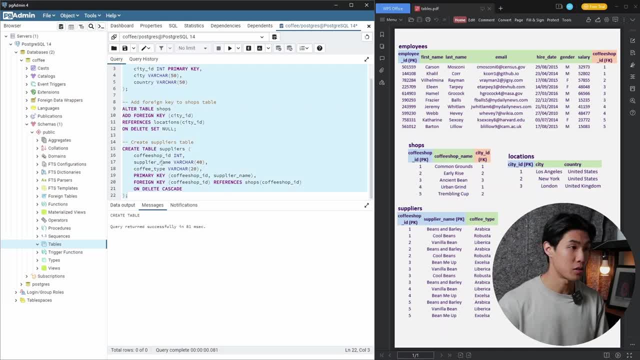 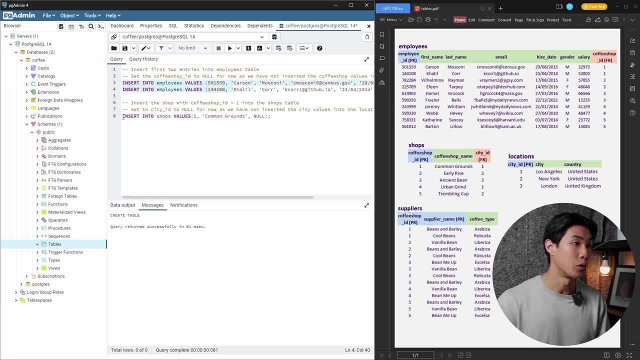 some values into the employees table and the shops table and just copy the code in here. so we're going to insert the first two rows into the employees table here and then we're going to insert the first row into the shops table. so let me just go to my table so we'll insert Carson Moscone Kahlil. 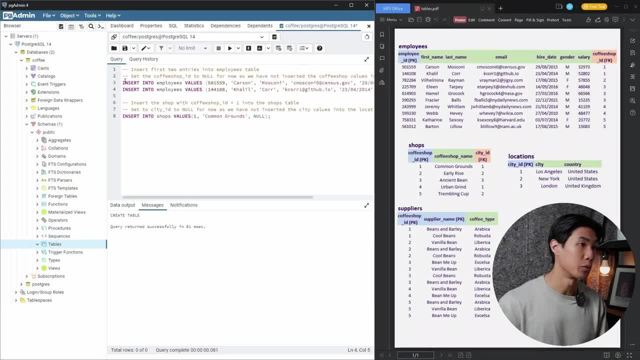 core and then common grounds, right here. so let's go through the code. insert into is the keyword and employees, and then you define values and then you just pass in the values. basically. so you see here that i passed in all of the values and you can see here that for the coffee shop id, i set it to. 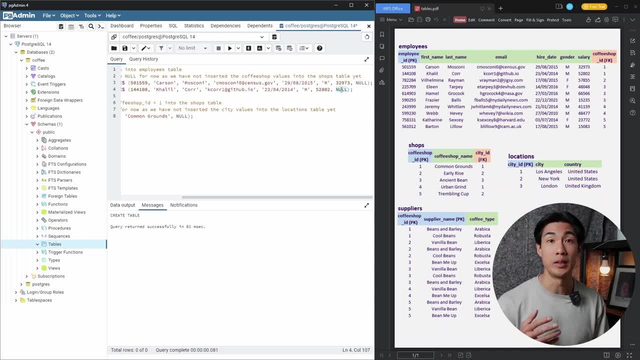 null at the moment. now, this is because obviously, we didn't actually create coffee shop id with coffee shop id one, so we haven't actually created common grounds within the shops table, so we cannot actually link this to the primary key of another table that doesn't exist yet. so i'm just gonna. 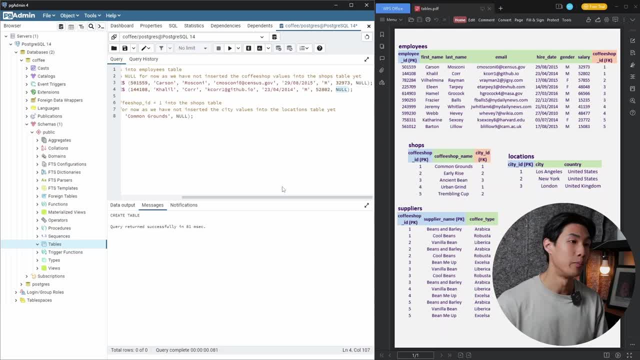 set this to null for now, and i will change it later on. and then, moving on to the shops table, we'll insert into the shops table and then we'll insert these values. now again, we set the city id here to null because we haven't actually created city id with city id, one in the form of los angeles. 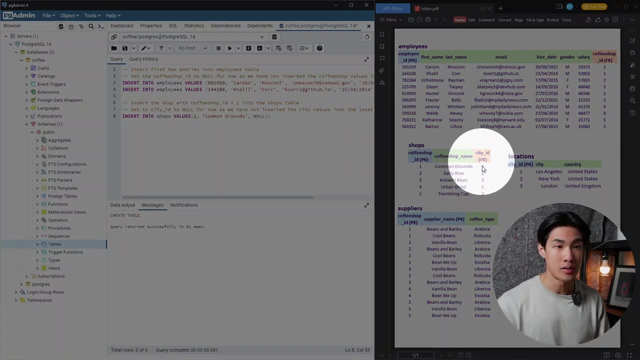 in the locations table. so let's have a quick look here. so you see city id. one is los angeles as you look across, but we haven't actually created this entry yet, so we leave it to null for now. so let me just run all of this code and you can see that the query was executed. 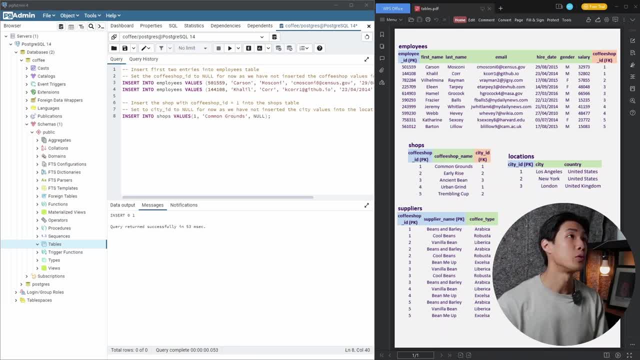 successfully. so now we're going to set the coffee shop id for the first two employees to one. so let me just copy this code in and we're going to update the employees table. we're going to set the coffee shop id to one where the employee id is in these employee ids. so essentially, if i 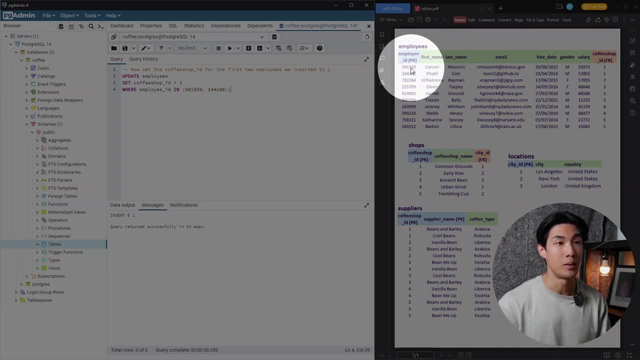 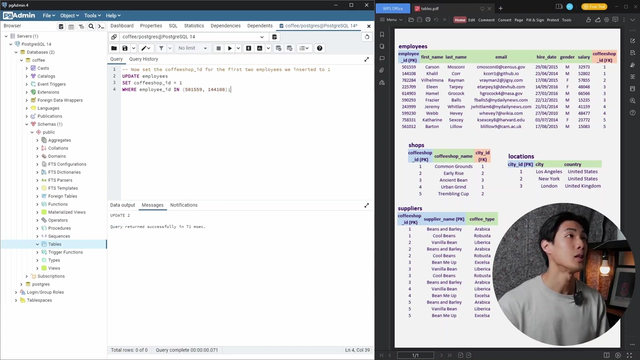 go back to the table here. you can see that the first two employees have employee id 501 559, and we're going to change the coffee shop id from null to one for these employees. so let me just run this code and you can see that the query executed successfully again. so now, next up, let's insert: 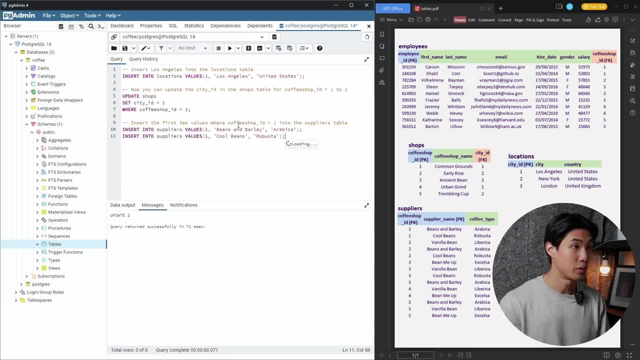 into the other tables as well. let me just copy this code in and you can see that we're going to insert the los angeles values into the locations table. so insert into which table locations, and then the values are one: los angeles and united states. so this the one will be the one that we're 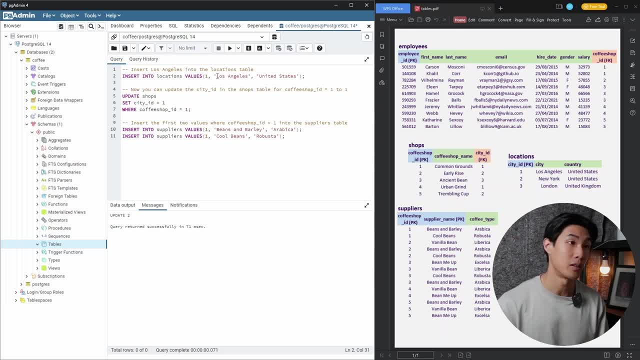 going to be the city id, the los angeles, obviously the city name and united states the country. after that we're going to update our shops table and set the city id to one where the coffee shop id is equal to one, because now we have actually created this los angeles value here so we can. 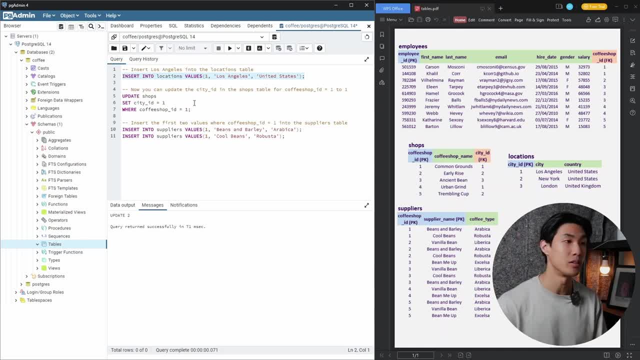 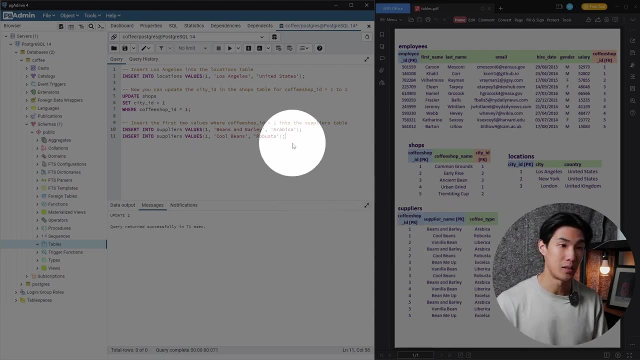 finally link our foreign key to the primary key of another table and then, finally, we will insert the first two values, where the coffee shop id is equal to one, into the suppliers table. so let me just go to the suppliers table and you can see here that the first two values will be in zen barley and cool beans- the suppliers. so let me just run. 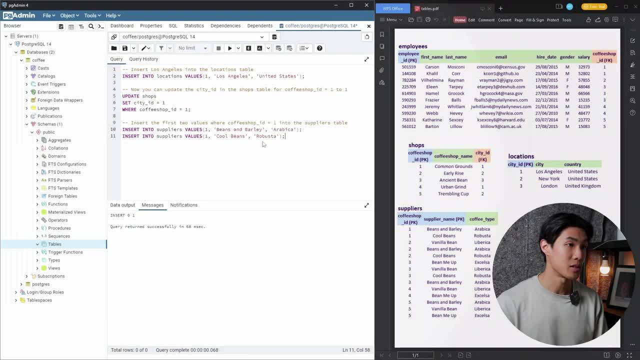 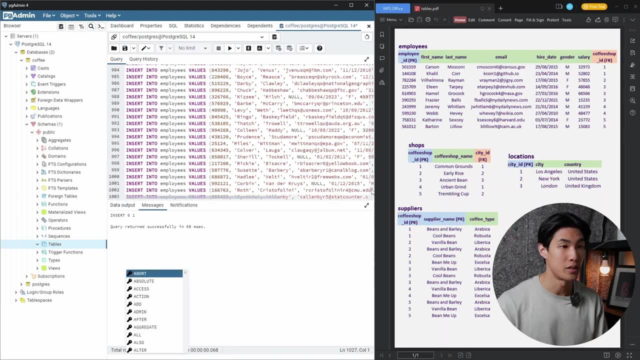 all of this code and you can see again that the query was returned successfully, so all should be good. now next up, i have all of the code in the file, so it's just a bunch of insert statements here. you see that i copy pasted in everything. but essentially what we will do is we will populate. 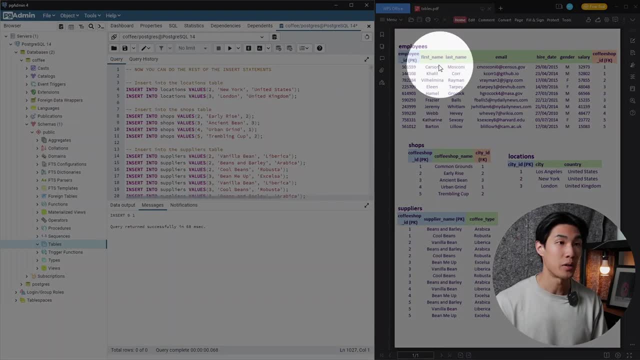 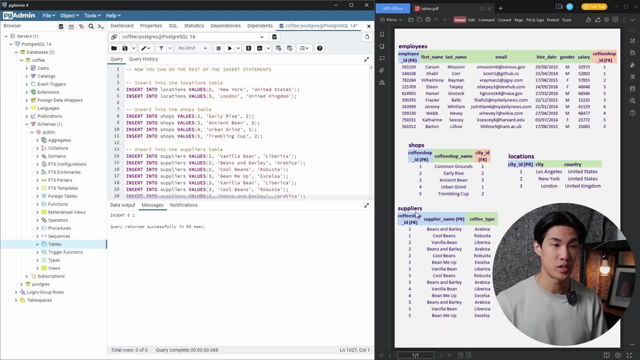 the rest of the tables using these insert statements. so if i go to the employees table, you will populate these eight entries and the remaining 990, and then you you will populate the shops table, the locations table and the suppliers table in full. So let me. 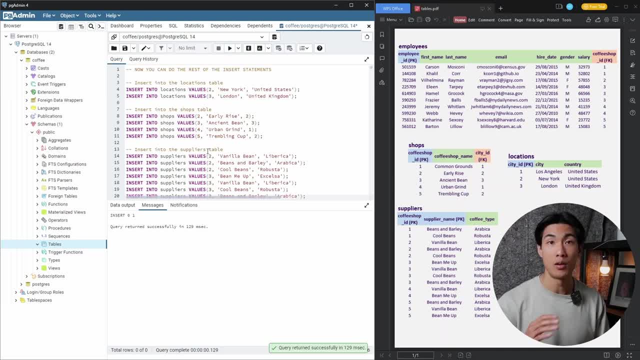 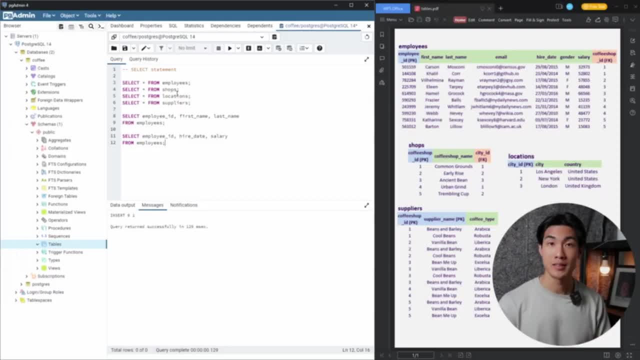 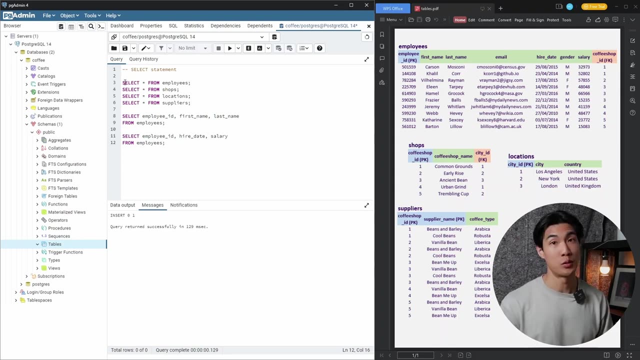 just run this code right here And you can see that now we have all of our tables created and the values inserted into these tables. Alright. so now it's time to move on to some basic select statements. So I've written a couple statements here And you can see that select star will be. 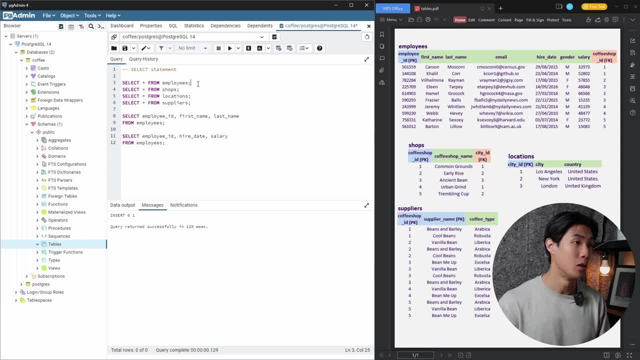 very popular, which is selecting everything from that table. So let's first look at the employees table And you can see that if you only highlight a section of the code here and when you run the code it'll only run that bit of the code. So select star from employees essentially just gives. 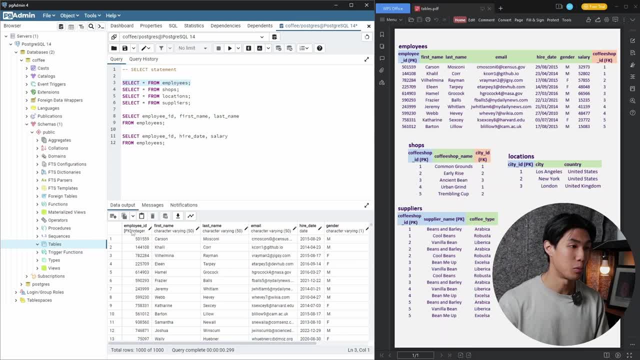 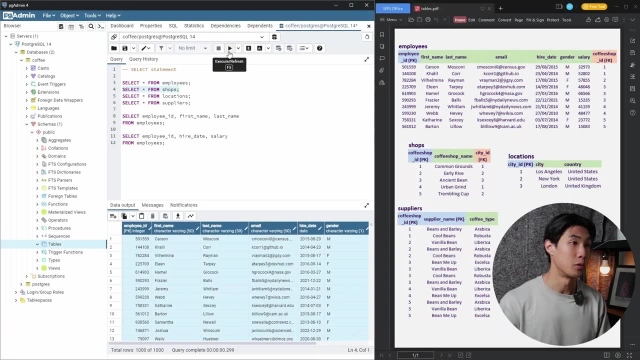 us all the values from the employees table. So you can see that we have the employee ID- first name, last name, email, hire date, gender, And then we also have the salary and then the coffee shop ID at the end, And indeed we have 1000 rows of observations. Now let's do select star from. 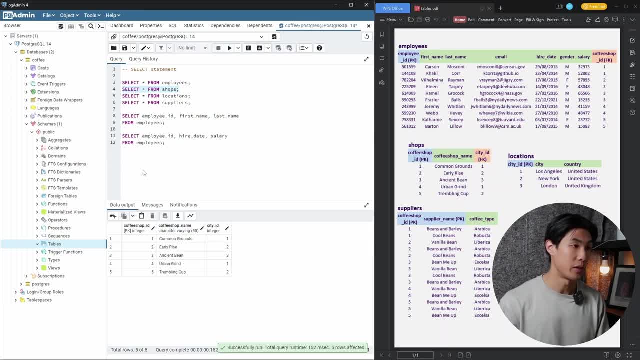 shops, So you can see that we've inserted all of the values correctly. Let's do locations next. Let me just select that And you can see that we indeed have Los Angeles, New York and London and we have United States and United Kingdom as countries. Let's select everything from the suppliers And then you can. 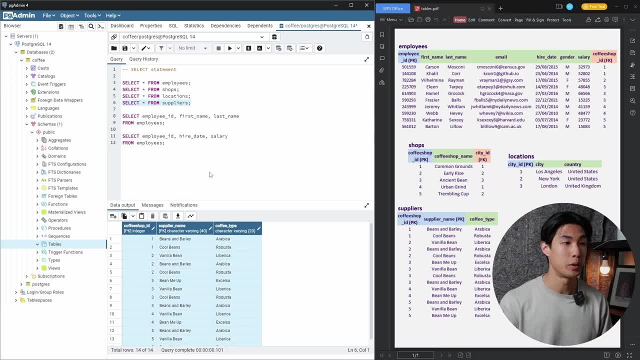 see the coffee shop ID, the supplier name and then the coffee type. Now, obviously, you don't have to select all of the columns within the table, So you can specify which columns you want to select, which is what I'll do next. So I'll only be selecting the employee ID, the first name. 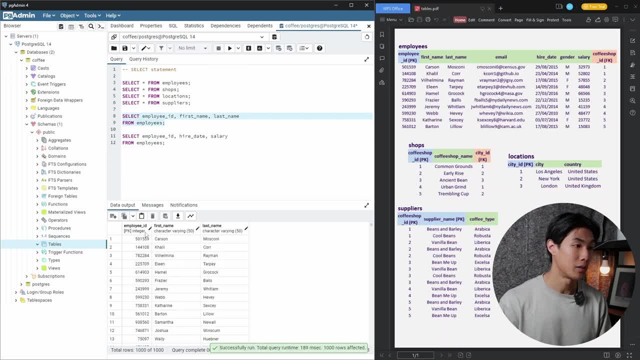 and the last name column. So I'll just select the first name and the last name column And then you can see that now we only get three columns on the bottom here: employee ID, first name and last name. Or we could just select employee ID, hire date and then the salary. So let me just run this. 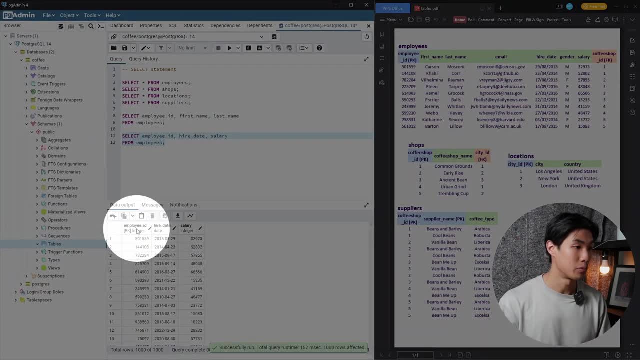 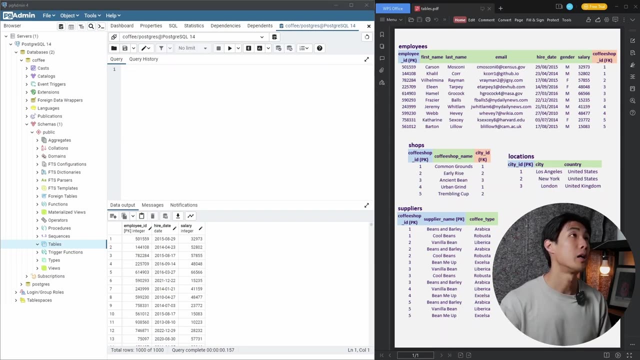 bit of the code here And there we go. You see, on the bottom we have employee ID, hire date and the salary. Now that we're done with the basic select statements, Let's combine these select statements with some where clauses using and, and or. So here's the code, And first of all, 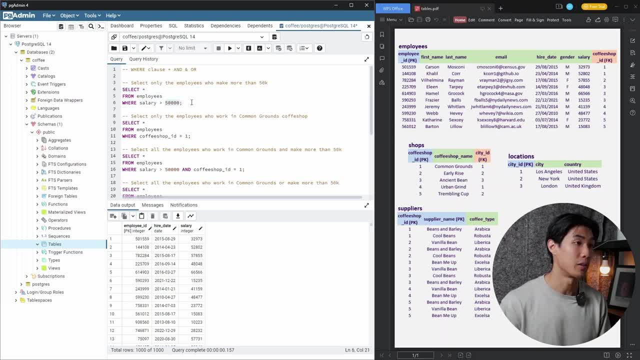 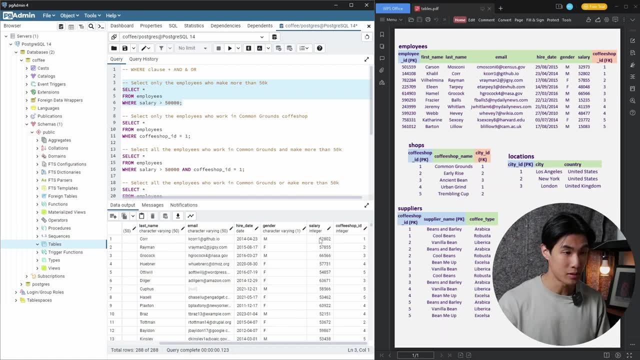 let's select all of the employees whose salaries are greater than $50,000.. So let me just run this code here And let's quickly look down the columns, And you can see the salary column here all of the values are above 50,000.. Next, let's select all of the employees who work in the common grounds. 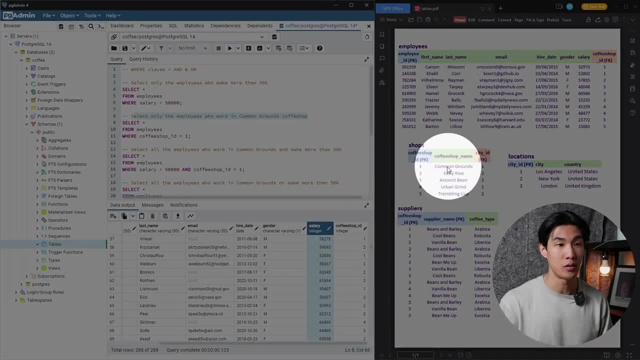 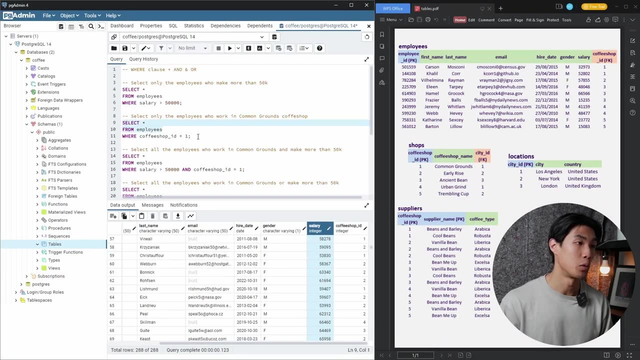 coffee shop. So if we look at our tables here, you can see that the coffee shop name is common grounds here and the coffee shop ID is one. So what we will do is we'll select star from employees. coffee shop ID is equal to one And if I run this bit of code here, you can see that the coffee shop 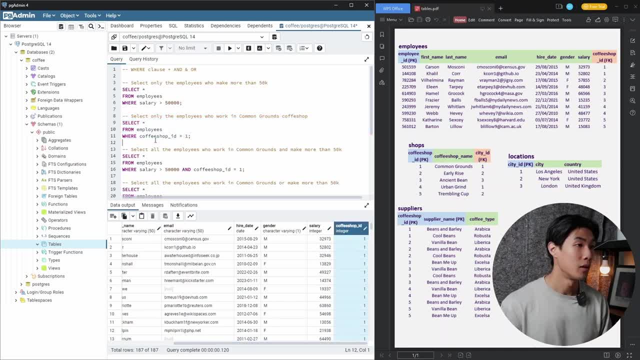 ID column only has values of one. Oh, and just quickly, by the way, you can do this hyphen, hyphen to create a note. So the moment you do this, SQL won't recognize that line of code as actual code, it will just be a note. you see here Now it's in a different color, So let me just undo that. 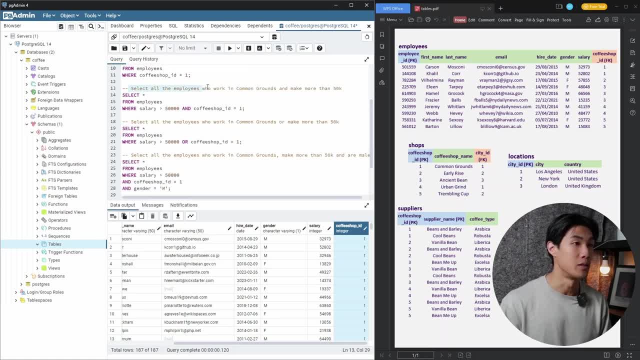 And then let's move on to selecting all of the employees who work in common grounds and make more than 50,000.. So we'll use the end operator with the where clause here. So we're saying that you need to be making above $50,000 and be working in common grounds. So let's 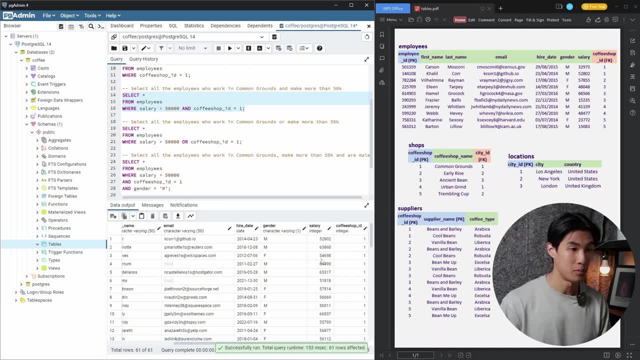 return that, And here we go. Let's just look down the columns. you see the salary: everything is above 50,000.. And then the coffee shop ID is one all the way. So next up, let's use the or operator. 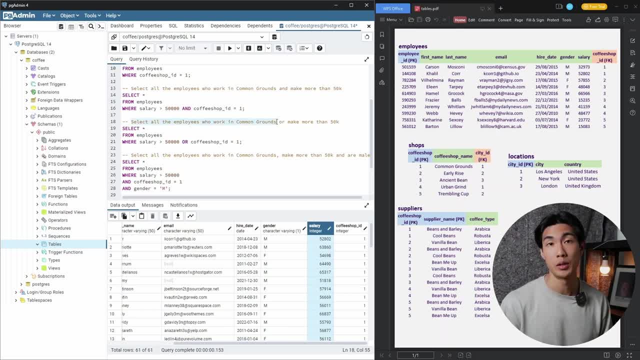 So we'll select all of the employees who work in common grounds- more than 50,000.. So let's run this bit of code here And now. if we're looking down the columns you can see that you know we have people working in coffee shop ID two, three and fives. 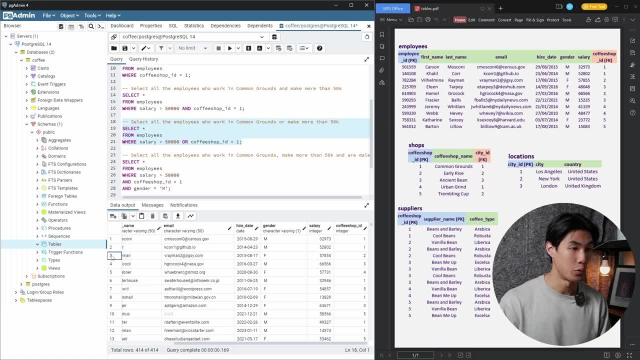 But this is because those people say, for example, row three: here this person is working in coffee shop, ID two, but is making more than 50,000.. So the query returned it. If we look at the first row, for example, this person makes less than 50,000, but is working in common grounds. So we 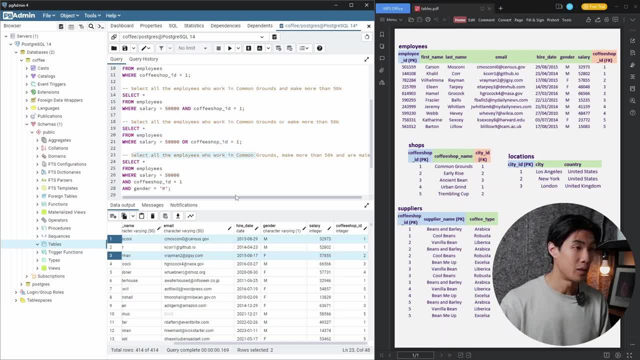 know the query returned it. Let's move on to selecting all of the employees who work in common grounds, make more than 50,000 and are male. So we're using two and operators here. we're saying if the salary is greater than 50,000, and the coffee shop ID is equal to one and the gender is. 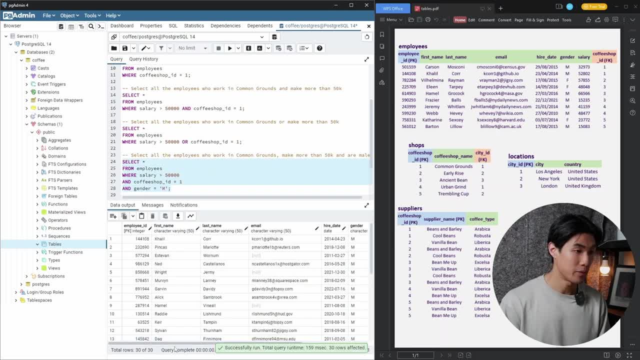 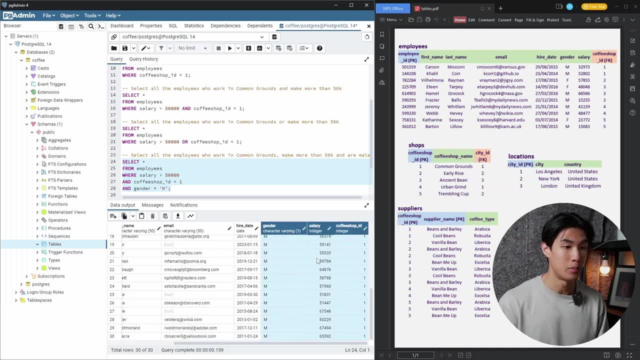 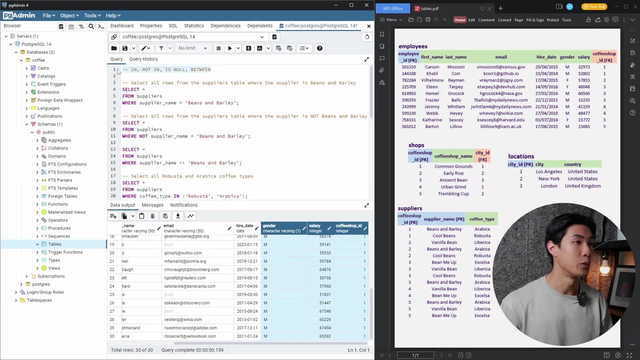 equal to male return that. So let's just do that. I mean, look across the rows here So we see gender is only M coffee shop ID, only one salary: all above 50,000.. All right, next up we'll be going through the in- not in his know- and between operators. So first of all we're going. 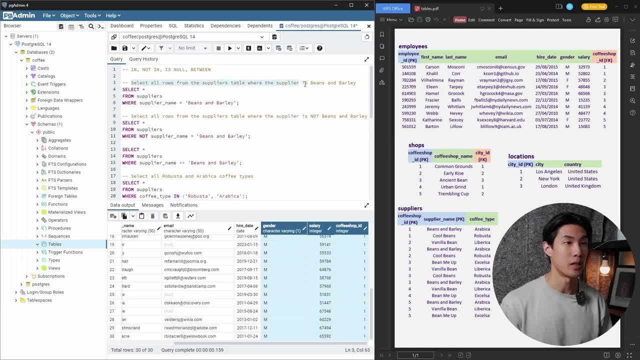 to select all of the rows from the suppliers table where the supplier is beans and barley, using the equal sign, So sex star from suppliers where the supplier name equals to beans and barley. So let me just run this code here And you can see that the supplier name here is only beans. 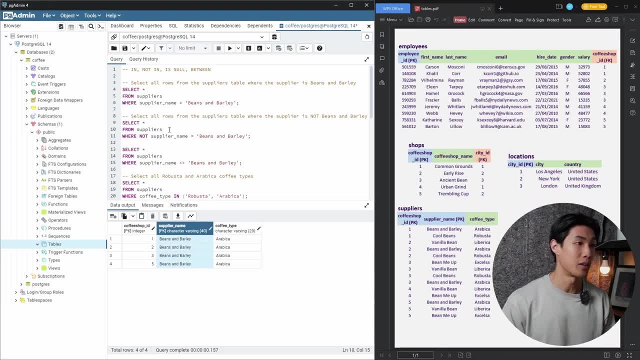 and barley. Now we can also do select everything from suppliers where the supplier name is not to beans and barley, just using the not operator. so let me just run that. so you see this line of code here: where not supplier name is equal to beans and barley. so let me just run this code here. 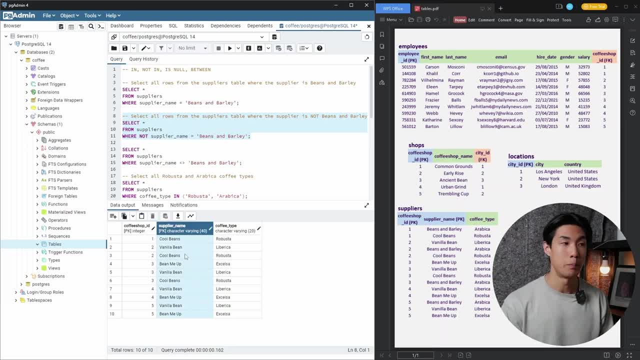 and you can see that now the supplier name has everything but beans and barley. so, moving on, you can use this sign as well, which is a not equal to sign, so this will return the exact same thing. let me just show you, and there you go: the supplier name has everything but beans and barley. okay, so 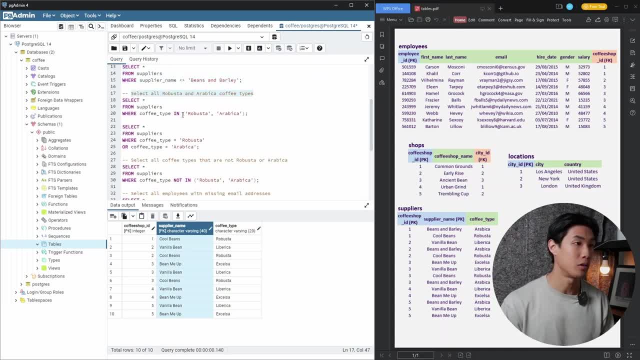 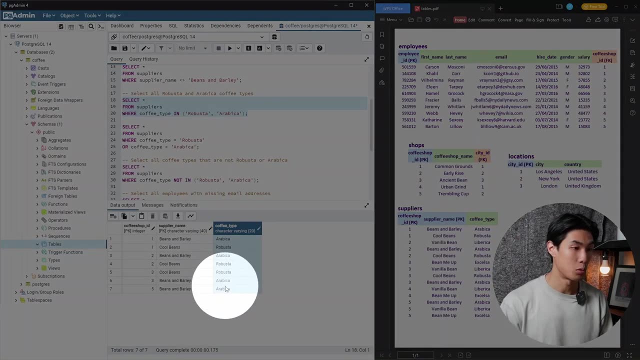 let's select all of the robusta and arabica coffee types using the in operator. so all i'm saying in the where clause here is: if the coffee type is in either robusta or arabica, then return that row. so we see here that the coffee type is only arabica or robusta, and obviously you could use the or. 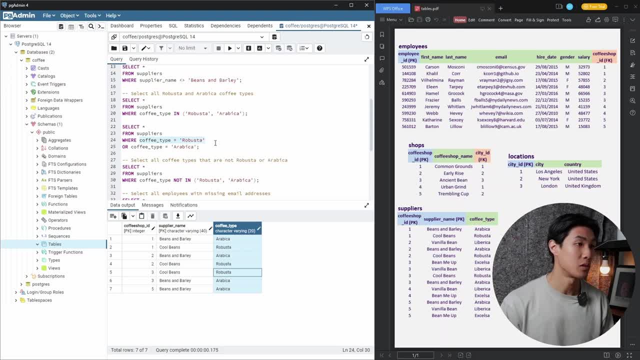 operator as well. so where coffee type is equal to robusta or coffee type is equal to arabica, and then it'll return the exact same thing. but probably using the in one is just a little bit neater and nicer because it's less repetitious. but 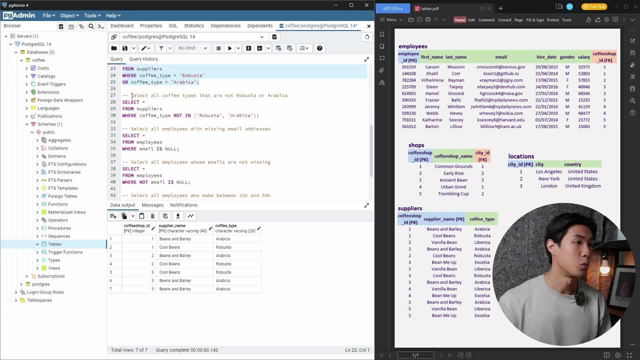 it's a matter of preference, i guess. so next up we'll select all of the coffee types that are not robusta or arabica. so obviously you could use the not in operator to do this. and let me just run this code here and you can see now that if i look down the coffee type column, you can see that i. 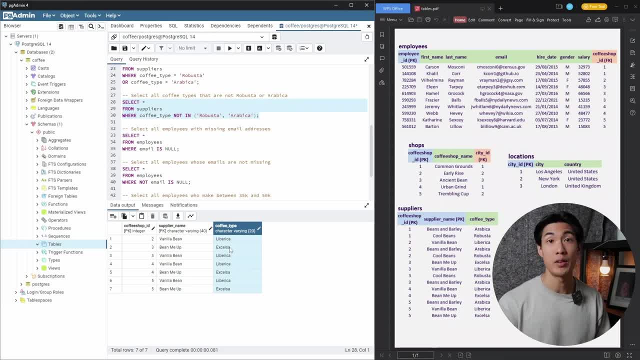 only have librica and excelsa coffee types, so everything but robusta or arabica. now next up, we're going to return all of the employees with missing email addresses, so select star employees, which is selecting everything from the employees where the email is no. so let's see what this 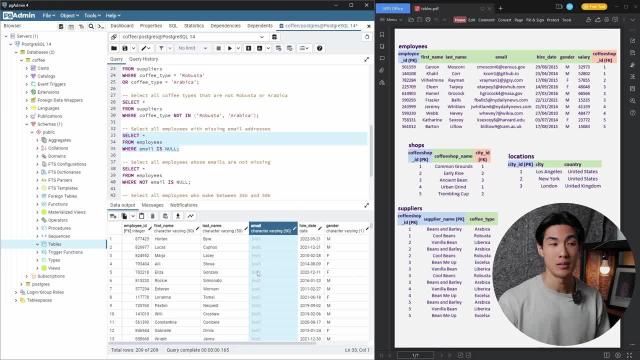 returns. let's look at the email column and indeed we have returned everyone whose emails are missing, and if you're wondering how many there are, you can see. the total number of rows returned is 209. so we have 209 employees with missing email addresses. now let's return all of the employees. 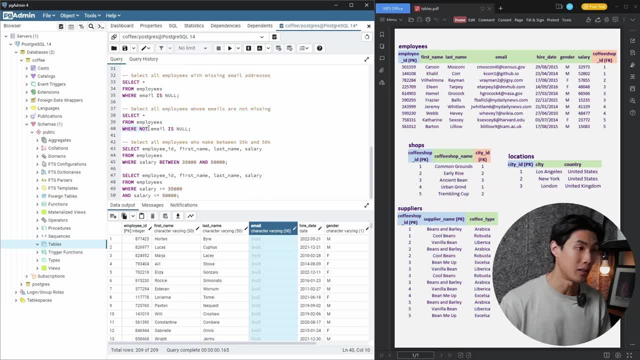 whose emails are not missing, let me just use. where not email is null, let me just run that and then you see, now the email column only has populated values, and then we have 791 employees whose email addresses are not missing. now. next up we'll select all of the employees who make between 35 000 and 50 000, using the between: 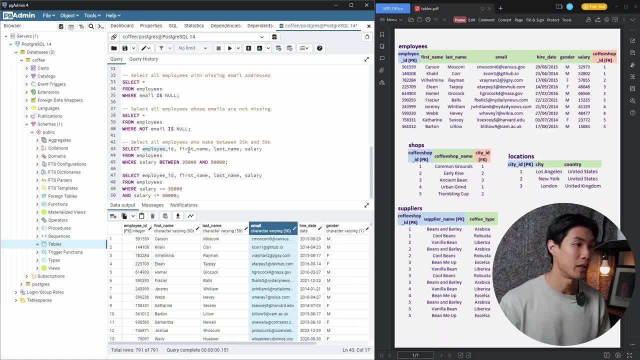 operator. so we'll only select the employee id, first name, last name and the salary columns, this time from the employees table. and we're saying that where the salary is between 35 000 and 50 000, return the rows. so this between operator is inclusive of both ends. 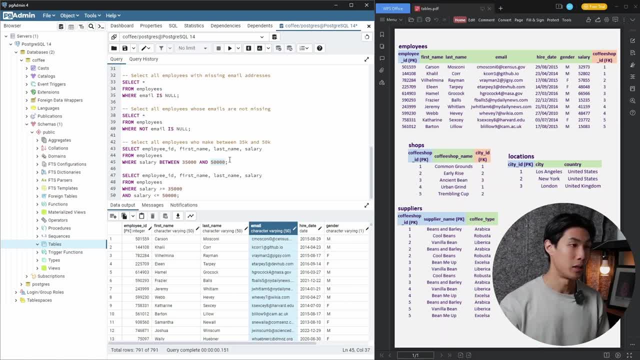 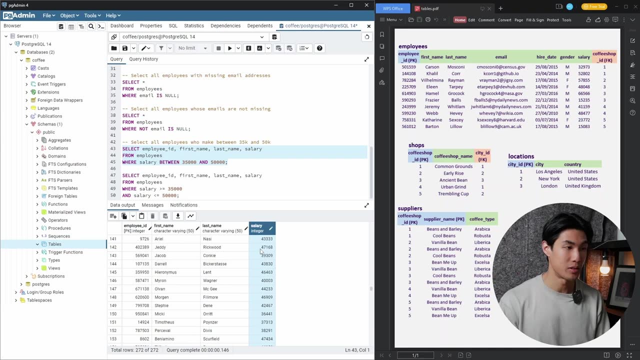 so if you're making 35 000, you're gonna be returned in this query, and if you're making 50 000, you're also gonna be returned in this query. so let me just run this bit of code here and let's look at the salary column as i scroll through. you can see that all these values are between 35 000 and. 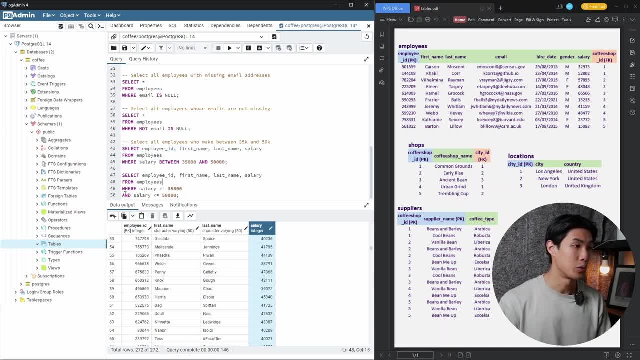 50 000. so next stop. obviously you could use the salary column in the salary column and, if you're, use the end operator as well. So this will give you the exact same result. Let me just run this code here. Let's look down the salary column And you can see that all of these values are between: 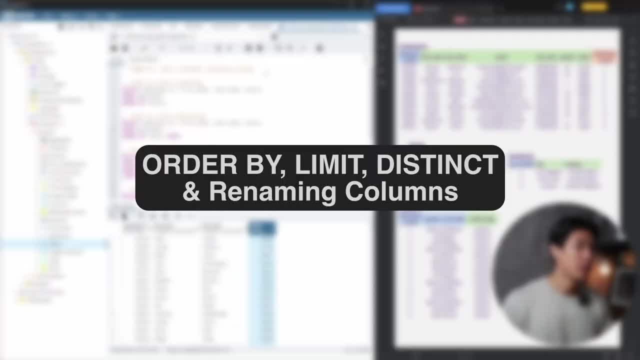 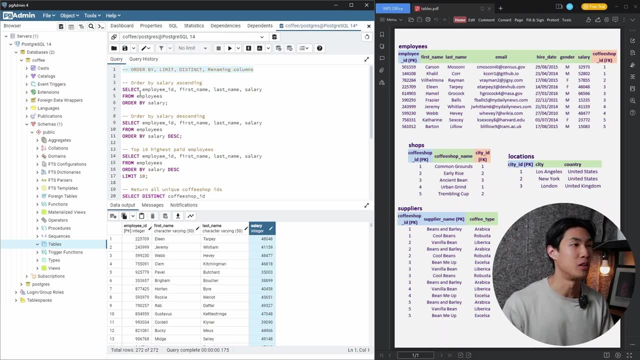 35,000 and 50,000.. Okay, we're doing really well. Let's move on to order by limit distinct And we'll also rename some columns. So first of all let's order by the salary ascending. So again, 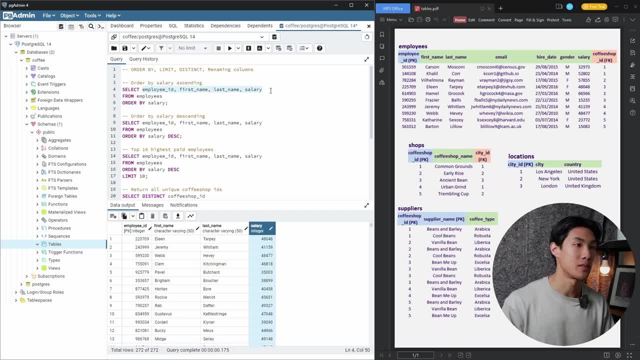 I'll only select specific columns. So I'll select the employee ID, first name, last name and the salary columns from the employees table, And then the keywords are order by, and then you just specify which column you want to order by. So this is salary for me in this query. let me just run it. 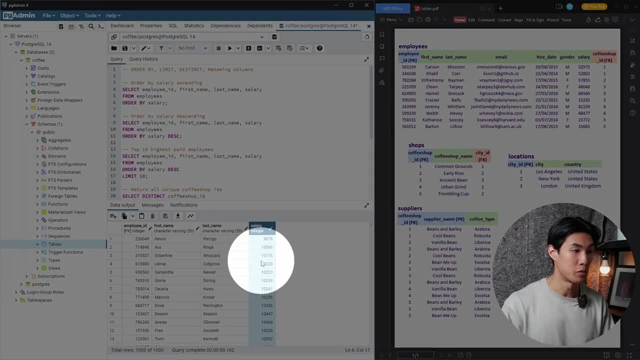 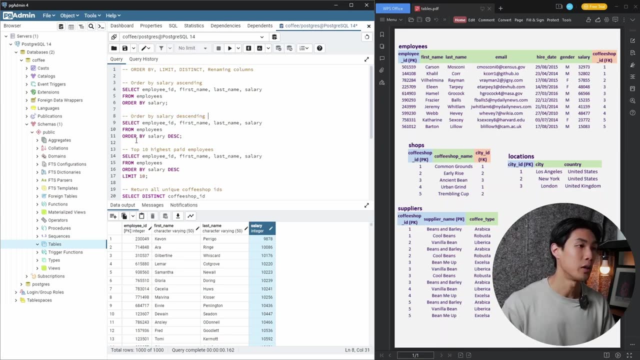 And then you can see by default in the salary column the order by happens in an ascending order. So next up, let's order by the salary descending. So the only thing you have to do is, after you put an order by and the column name, you pass in the keyword DESC for descending And 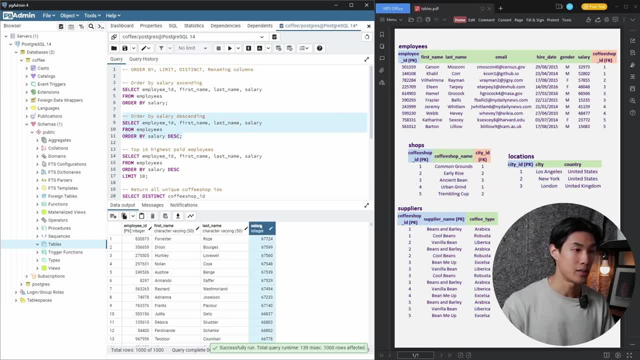 let's just do that. Let's run the code And now, if I look at the salary column, you can see that you have the highest salary on the top. So the maximum salary is 67,724.. And then the minimum is $9,878.. 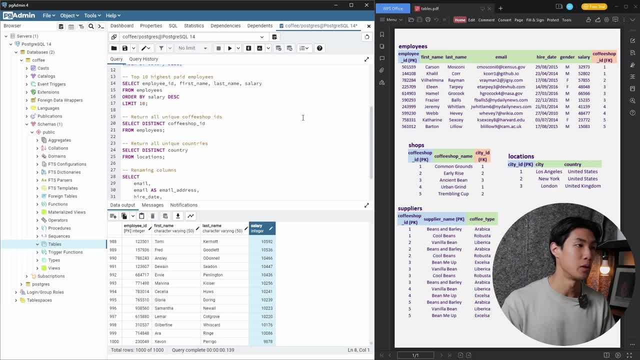 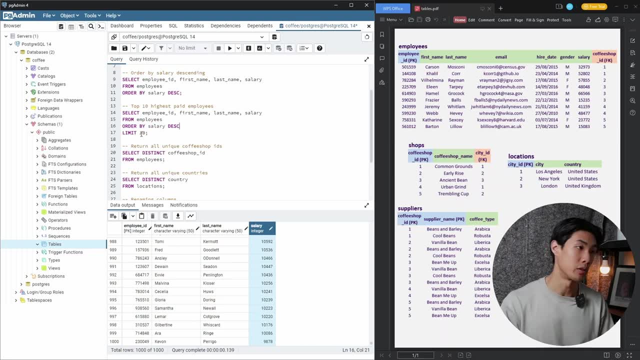 Okay, so how about we return the top 10 highest paid employees? So the only thing we have to do, compared to the previous query, is, after order by salary descending, we need to limit what we return. So if we limit it to 10, obviously we return the top 10.. 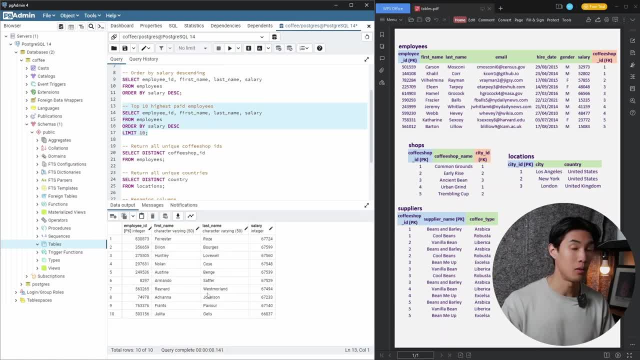 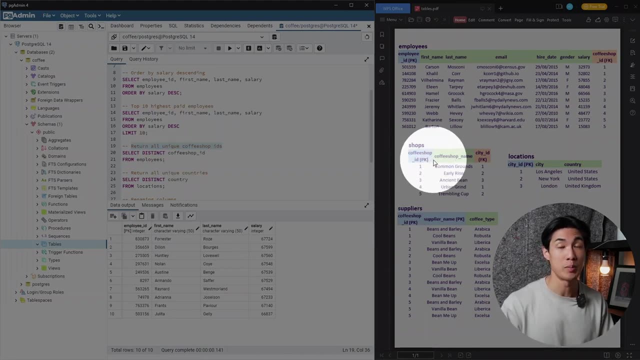 highest paid employees. So we can see that these people are the highest paid people. Now how about we return some distinct or unique coffee shop IDs from the employees table? So we know that within the shops table we have five coffee shop IDs corresponding to the five coffee 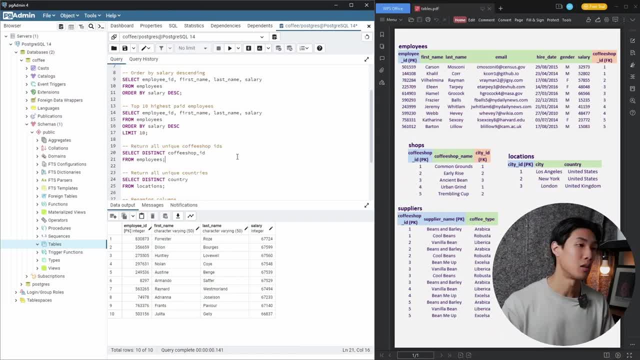 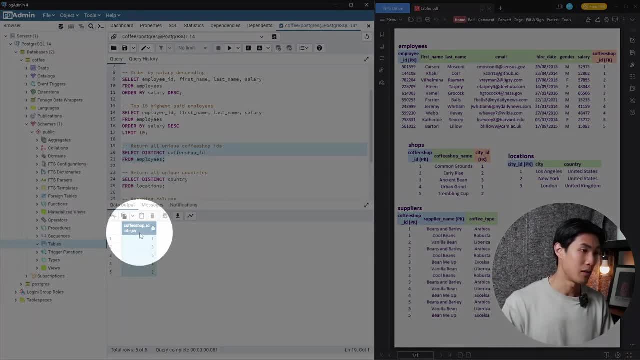 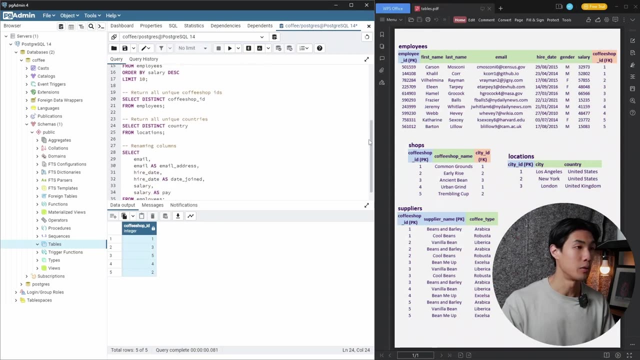 shop names. So we're expecting to see five unique coffee shop IDs in the employees table as well. So let me just run this bit of code here And you can see here that indeed we have five unique coffee shop IDs, So 12345.. Now how about we return the unique countries from the locations table? So 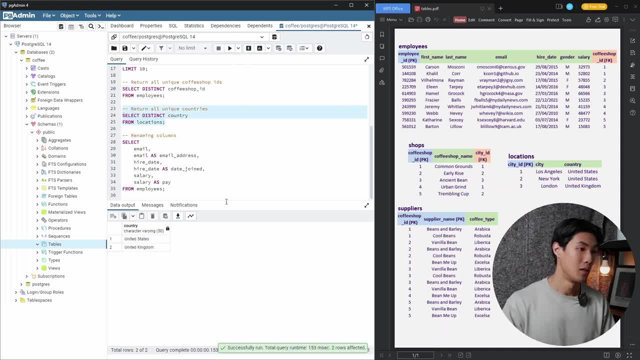 select distinct country from locations. Let me just run that. And indeed we have two unique countries, the US and the UK. So next up let's rename some columns. So renaming is very, very simple with the as keyword. So I am going to select the email column and then the email column. 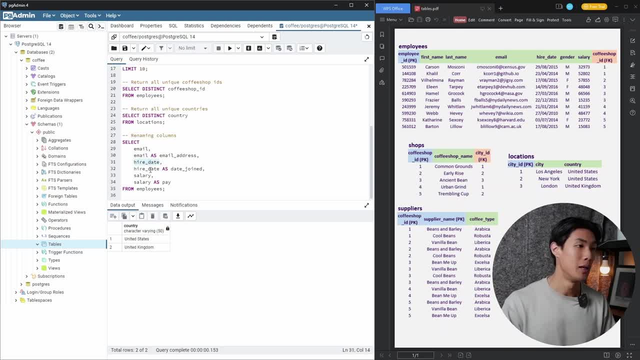 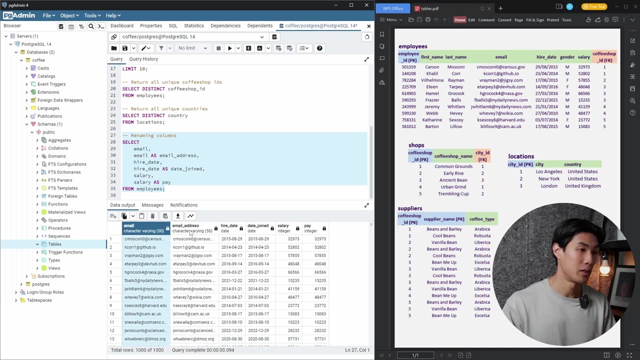 renamed as email address, then also the higher date column, and then the higher date column renamed as date joined, and then the salary column, And then I'm also going to rename the salary column to pay. So let me just run this code here And you can see that now we have six columns on the bottom. So email and then we have email. 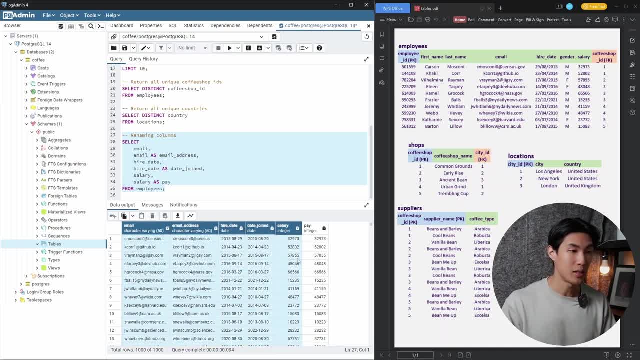 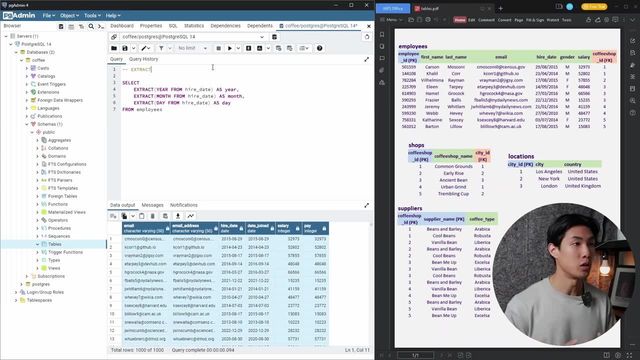 address, we have higher date and then we have date joined, we have salary and then we have pay. Okay, moving on to extract. this is going to be a short section, So all we're going to be doing is extracting some date information from the date column. 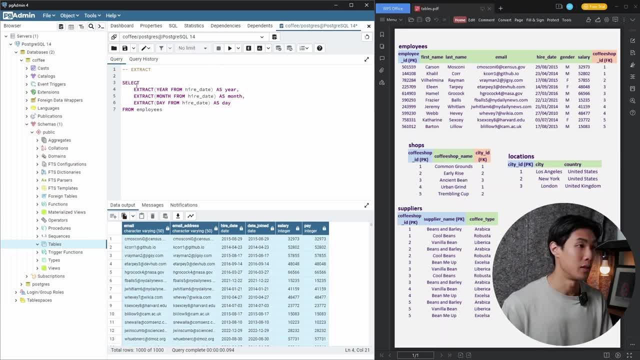 Which is our higher date column. So you can see here that the function we use is extract, and then we define what we want to extract from the specific column. So first I'll extract the year from the higher date column, And then I will extract the month and then the day, And then I am. 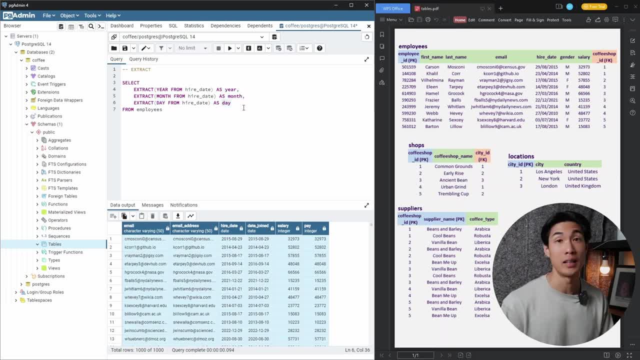 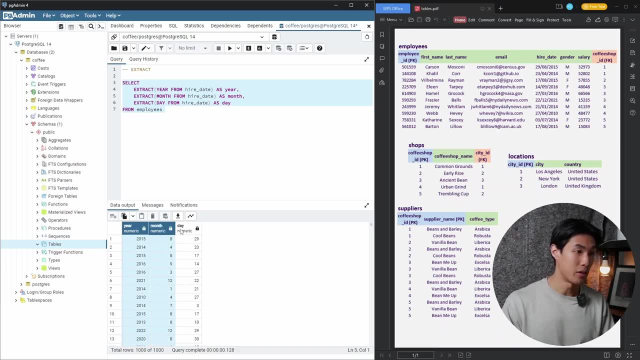 going to rename these columns as year, month and day respectively. So let me just run this code here And you can see that on the bottom now I have the year, I have the month and then I have the day. And let me just actually pass in the year, month, and then I have the day And let me just 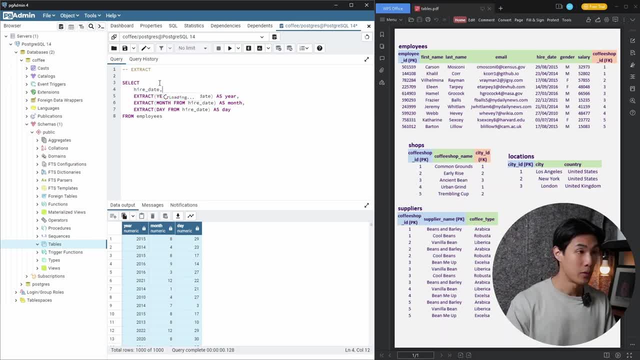 extract the actual column as well. So higher date right here, And then it's easier just to see what we extracted. So if you look at row one here, you can see that the higher date is 2015,, August 29.. So the year is going to be 2015,. the month will be eight, obviously for August. 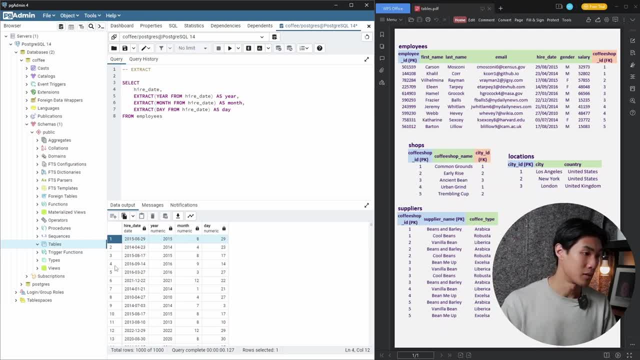 and then the day is 29.. Or let's look at another one, say row five here: 2016,, March 27.. So the year is obviously 2016,. the month will be March, so three. and then the day is: 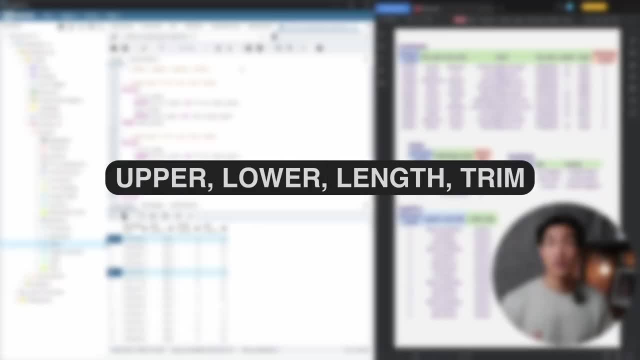 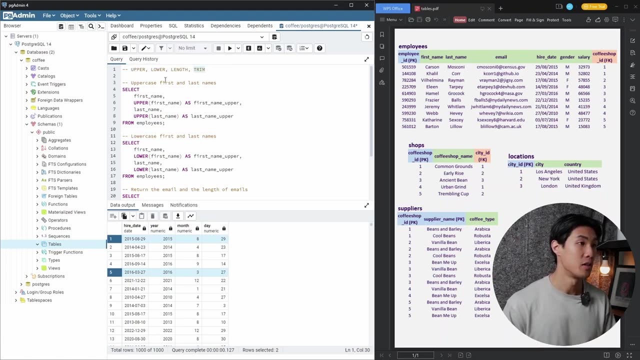 27.. And that's extract for you. Alright, so let's move on to some string manipulation. So we'll use the upper, the lower, the length and the trim functions first. So first of all I will uppercase the first and the last name. So I will select the first name column And then I will uppercase the. 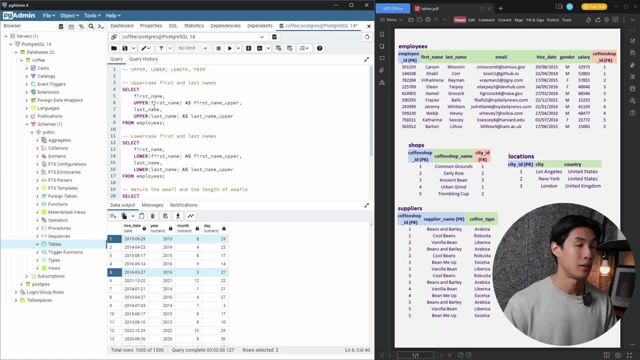 first name column and name it as first name upper And then I will select the last name And then I will uppercase the last name column and rename it as last name upper from the employee. So let's see the results. So if you look at the bottom, now we have the first name And then we have the first. 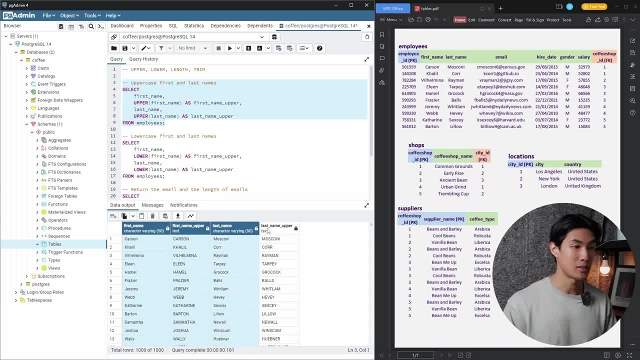 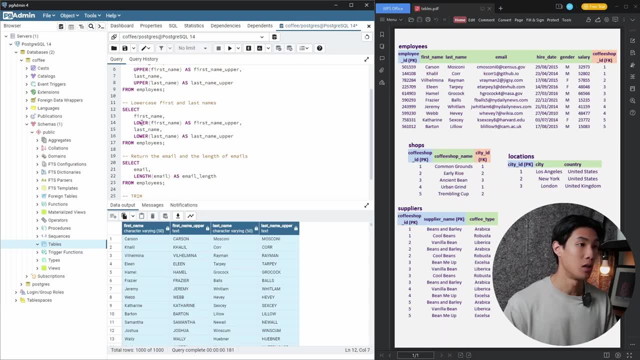 name in uppercase, And then we have the last name, And then we have the last name in uppercase. So we can obviously, of course, lowercase these letters as well. So you just need to change the upper to lower. So let me just do that in the next query, And if I run this one now, you can see that we. 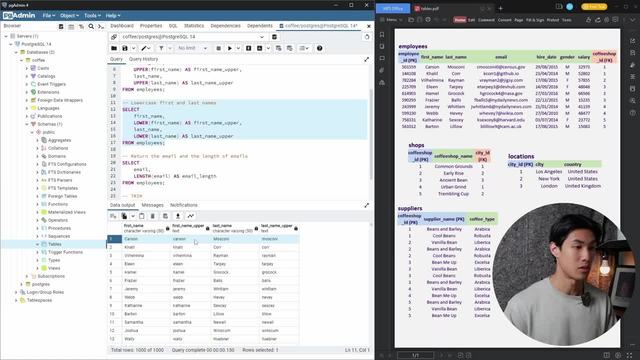 have Carson in the original format, then we have Carson lowercase only, And then we have Moscone in the original casing, And then we have Moscone in lowercase only, And then we have Moscone in lowercase only. So next up we'll use the length function and we will return the length of the 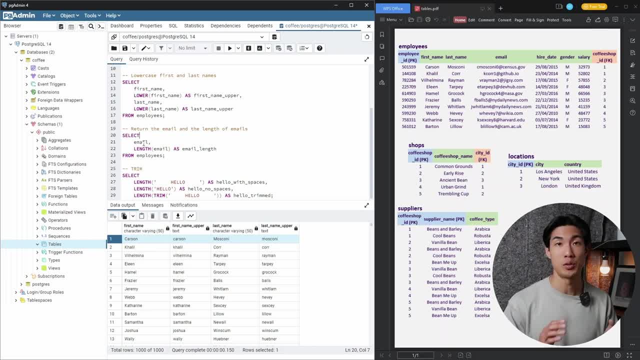 emails. So first of all I will select the email column, just so you can see what it looks like, And then I will return the length of the email column. So essentially this one just counts the number of the characters. So let me just do that And let me make the email column a little bit wider here. So 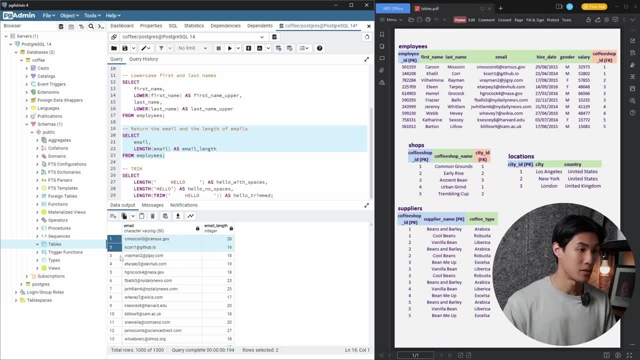 you can see that the first email has 20 characters, the second 116, the third 118, so on and so forth. Next up, let's look at the trim function. So for this, I just created some simple hello text here. 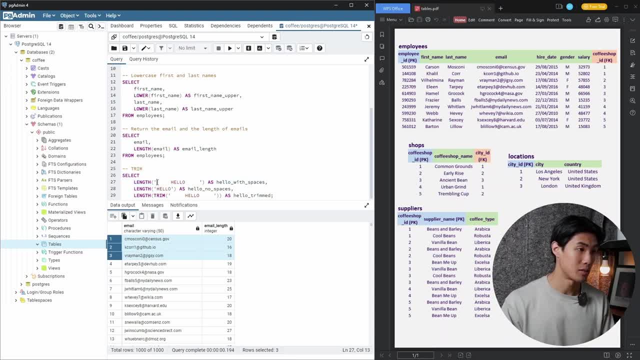 So you can see that the first one is hello with spaces. So you can see that I passed in a bunch of spaces here. And then the second length is just for hello, with no spaces. And then the third one. I'm using the length function But within this function I'm actually trimming this hello with. 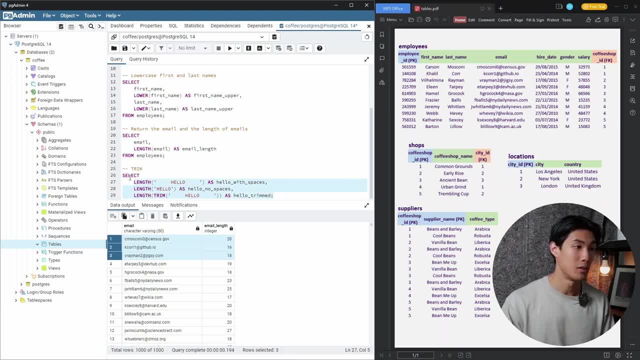 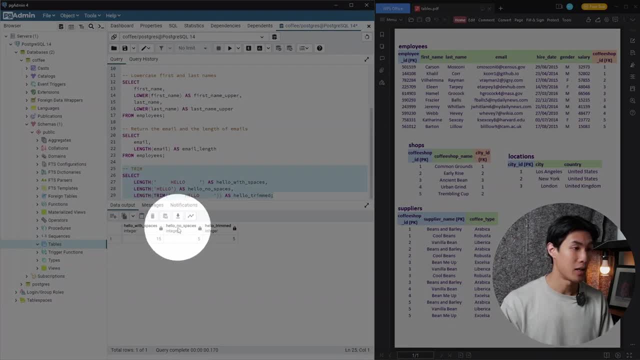 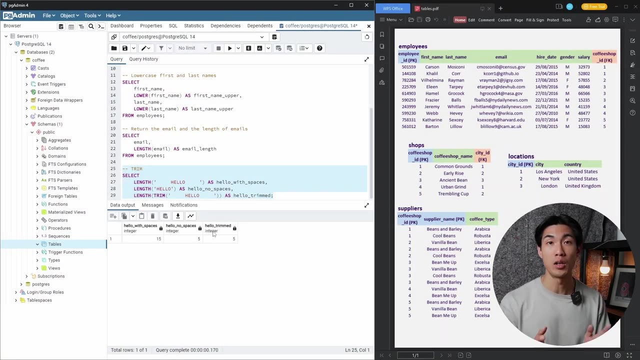 spaces And I'm calling this column as hello trimmed. So let me just run this code here And you can see that the hello with spaces has 15 characters, the hello no spaces has five characters and the trimmed hello also has five characters. So the trim just removed all of the 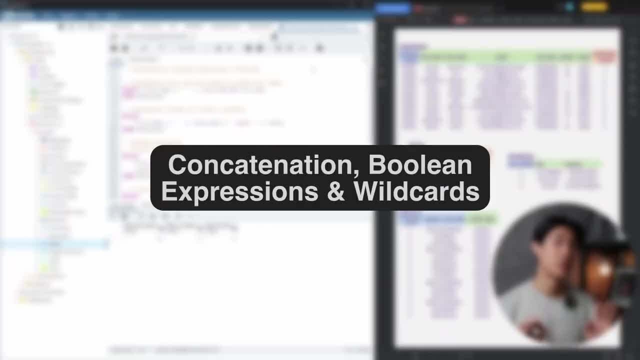 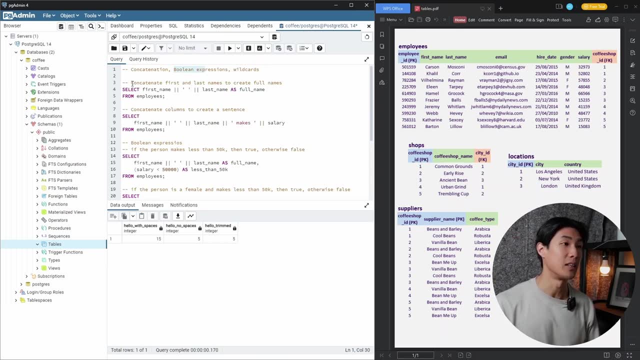 white space. Alright, next up some more string manipulation using concatenation, Boolean expressions and wildcards. So first of all, let's concatenate the first and the last name to create full names. So when we're concatenating text, we're just joining text one after the other, basically So 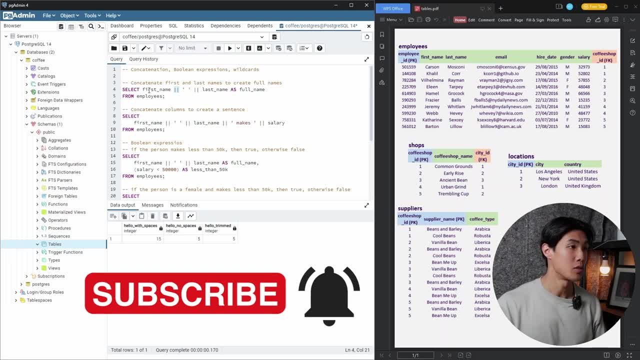 you can see this double vertical bar here. this is what you have to use. So first I'll select the first name column And then I want to pass in a space between the first name and the last name. then I select the last name column and I renamed this column as full name. So let me just run this. 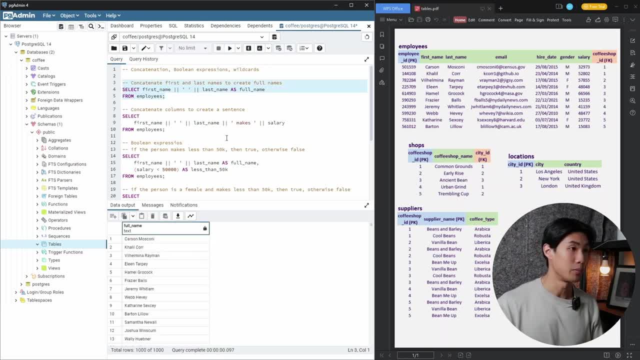 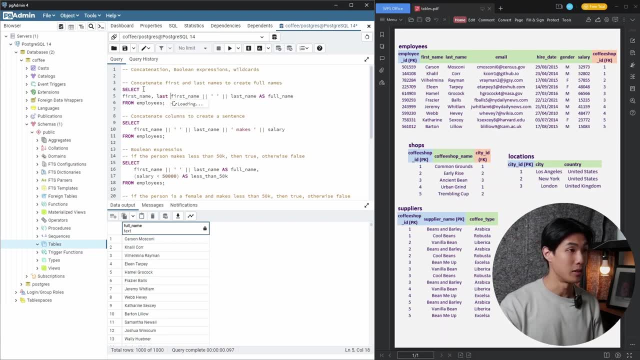 code here And you can see that now we have the full names on the bottom. And just to make it easier for you to see, let me just pass in also the first name and then the last name, And then you can see that now. 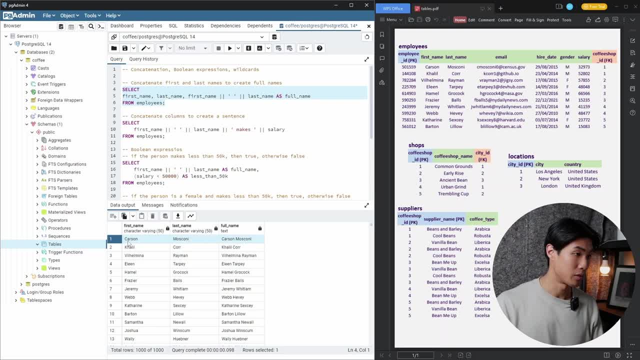 easier to see, probably. So if you look at row one, you have Carson here as the first name, last name is Moscone And then you have the full name, which is Carson Moscone. So we can also concatenate columns to create a sentence or whatever text you wish. So in the 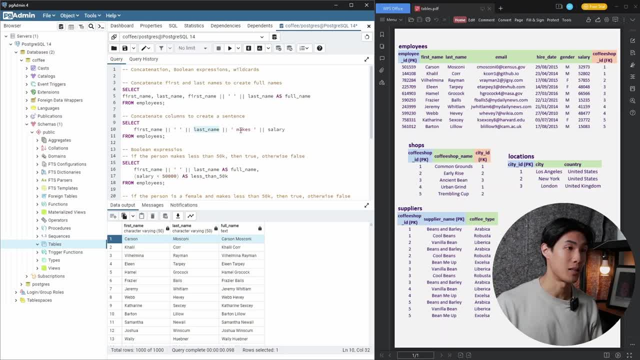 next one. we're going to say that first name space, last name makes this much money. So let me just run this. And now we can see that Carson Moscone makes $32,973.. Kalila core makes 52,000.. And 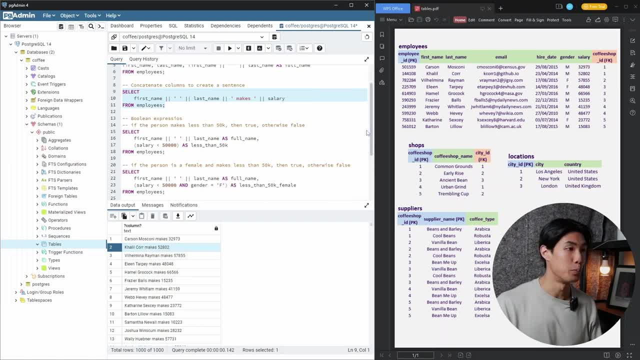 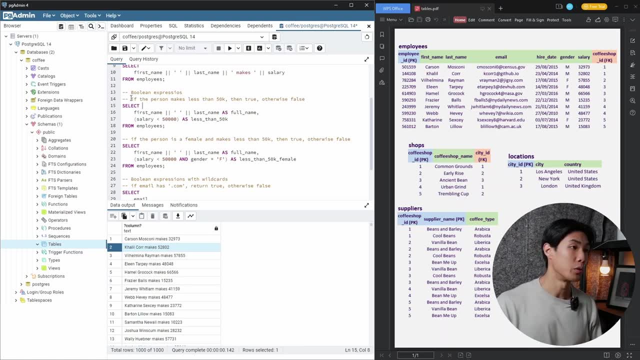 then we can see that Carson Moscone makes $10,842.. Now let's move on to Boolean expressions, And Boolean expressions are essentially just true or false expressions. So first of all, we're going to say that if the person makes less than $50,000, then it's true, Otherwise it's false. So I'm 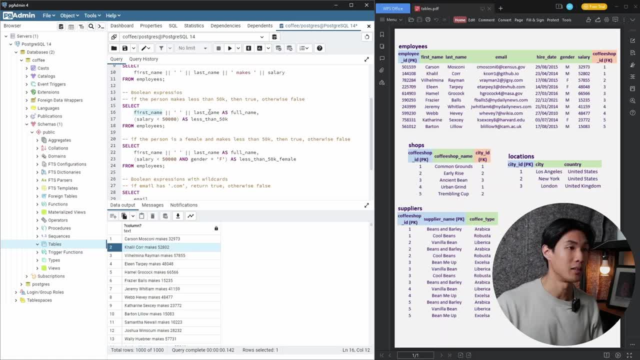 saying here: select first name and then we're concatenating the last name as the full name column, And if the salary is less than 50,000, then just give me true, otherwise give me false And I am going to name this column as less than 50k. So let's see what happens here. Let me just 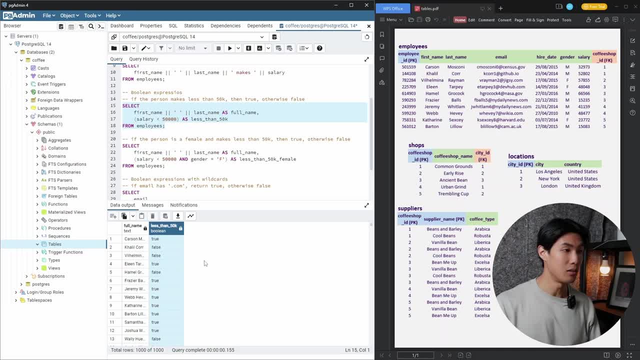 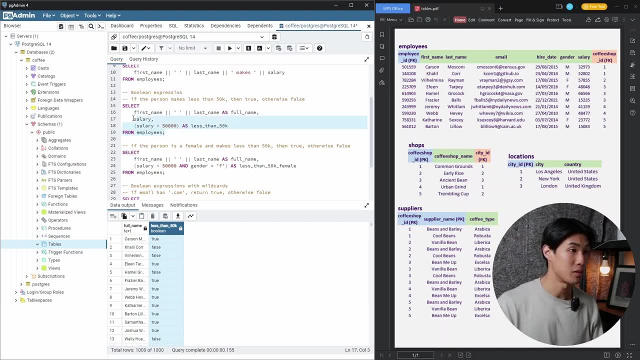 run this code And you can see that within this less than 50k column we just have trues and falses returned, And it would probably help if I passed in the salary as well here. So let me just find the salary column And then now, if we look at it, you can see that Carson Moscone makes under. 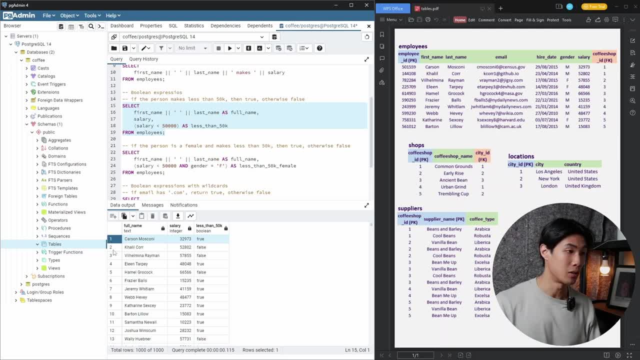 $50,000 here. So it will be true. But Kalila core, on the other hand, makes over $50,000.. So it will be false. Now, next up, let's go with another Boolean expression. So if the person is a female and makes less than 50,000, then true, otherwise false. So now we have an end operator. 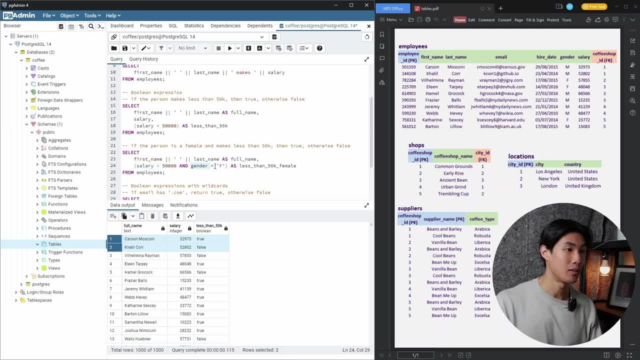 here. So we're seeing that if you're making less than 50k and you're a female, then give me a true, otherwise give me a false and I am going to name this column as less than 50k female. So let's select this And now we can see. again we have the trues and falses And again it would. 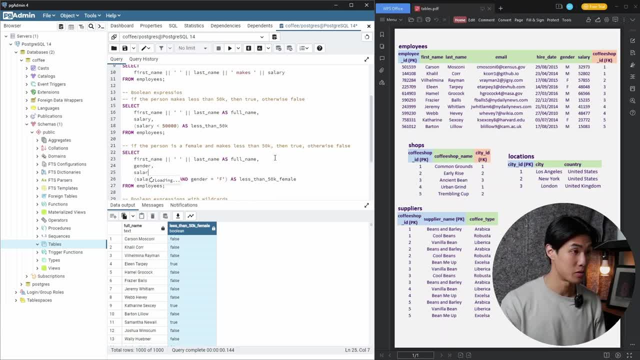 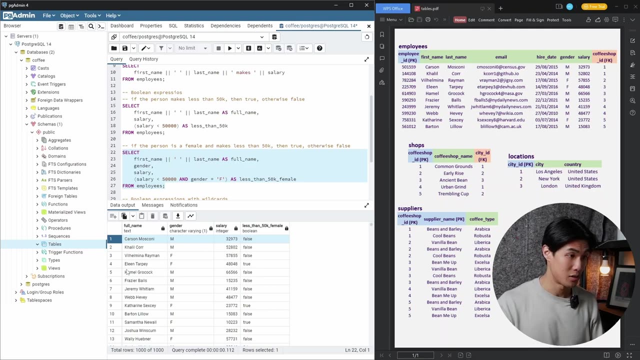 probably help if I just chose the actual column, So salary, as well. Let me rerun this code right here And you can see now that say, for example, the first entry here is false because the person is a male and well, makes less than 50,000.. And then let's find an entry that's true. So there we. 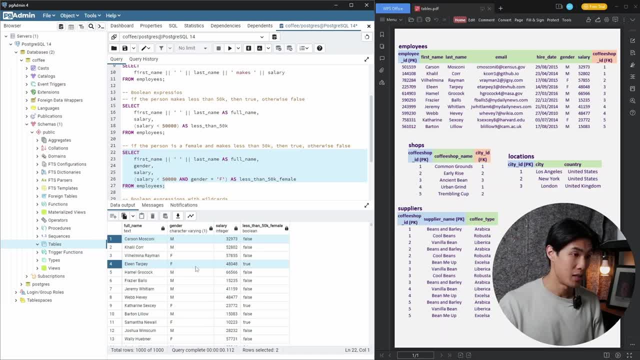 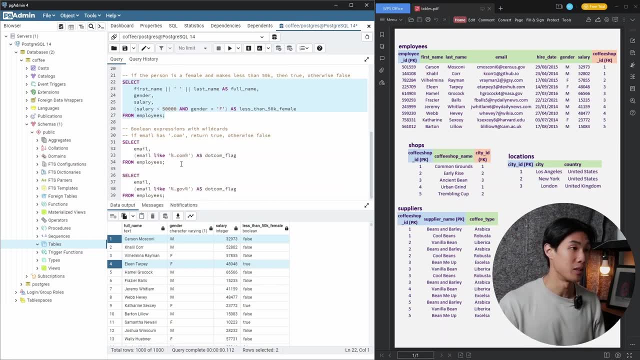 go row four: Aline Tarpeh. So she's a woman and she's making less than $50,000.. So the condition will be true. Now let's move on to something a little bit more interesting. So boolean expressions with wildcards. So wildcards are just string jokers. 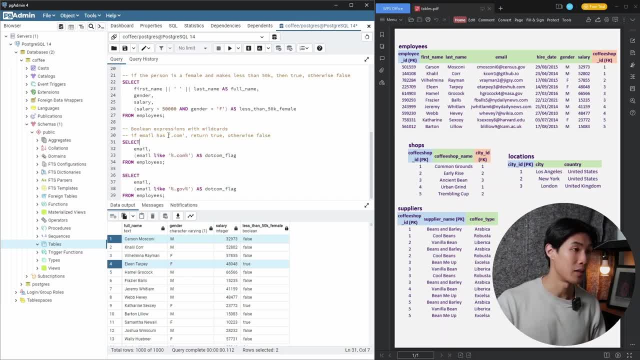 And we're going to find emails that have acom convention and then return that as true, otherwise as false. So we're going to select the email column And then you can use the like operator, And then you can use this percent sign to look for wildcards. So basically I'm saying: 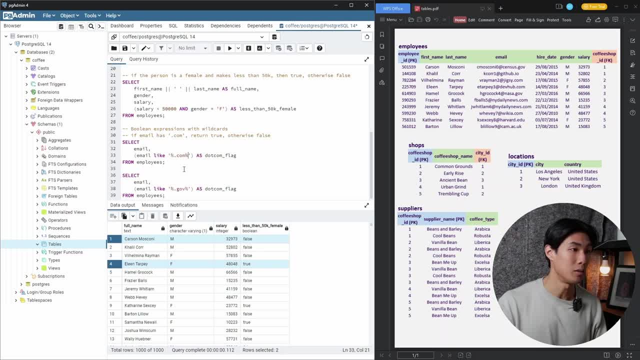 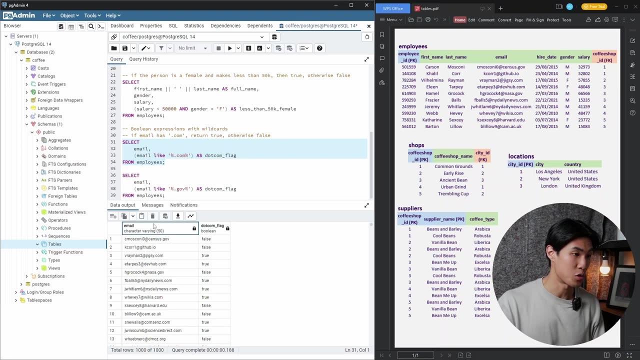 that anything beforecom and anything aftercom, just as long as it has thecom convention, then give me a true and I will call this columncom flag. So let me just run this code here And you can see that everything that has acom in there will be returned as true. So if I look, 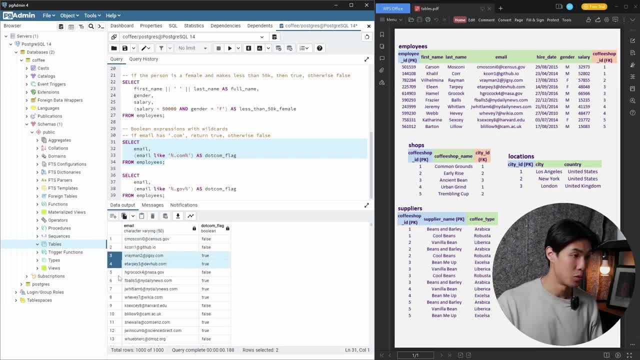 at row four, it's true, row three also true. But if I look at row one, for example, it'sgov and it's false. But obviously we could look for any other naming conventions as well, or email conventions. So I'll look forgov next And it'll be the, not thecom but the. 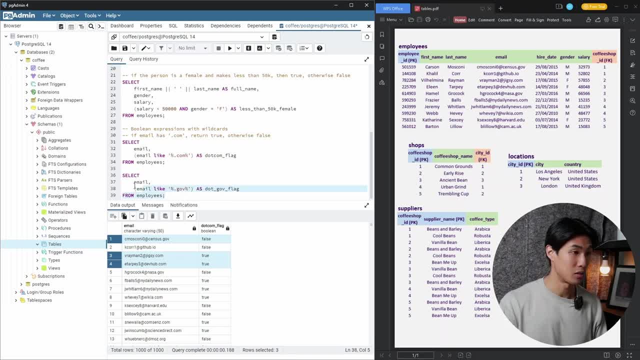 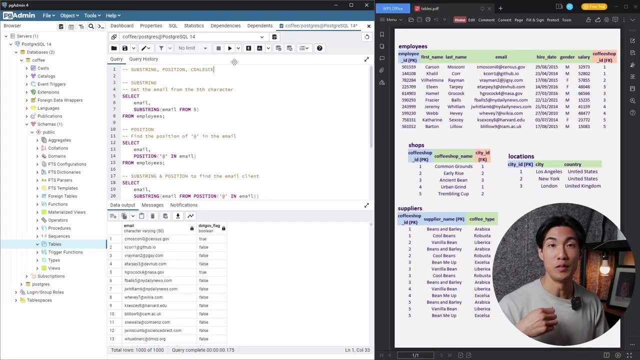 gov flag. So I'm just renaming this asgov And then now, if I run this code, you can see that the first line will be true. the second line will be false, because the first line isgov, the second line isio. Let's continue with the theme of string manipulations And we'll use substring. 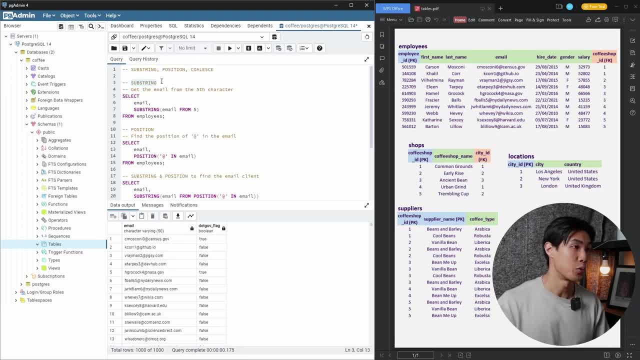 position and coalesce. So let's go through substring first, And substring essentially just gets you a text from whatever character you specify. So what we're going to do here is substring the email column and we're going to get all of the characters from the fifth one onwards, inclusive of the fifth character. So let's see. 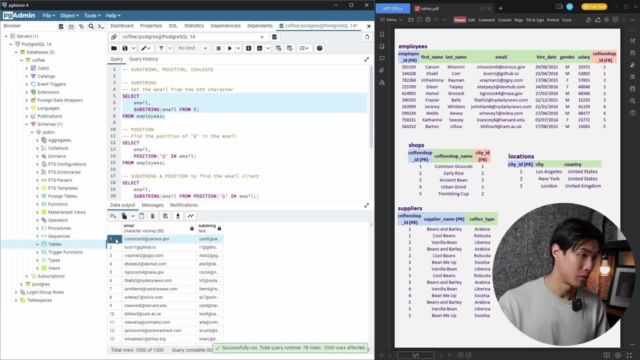 what this is going to return. And you can see that we have the first row here, So cmosconi at cmosconi, zero at censusgov. But then in the second column we only have coni zero. So this is because coni- the C in the coni, is the fifth character And we're returning everything after. 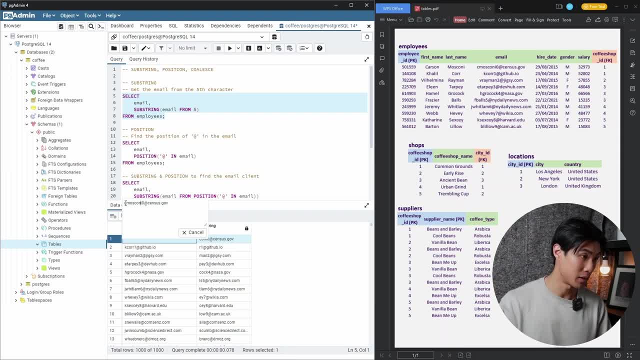 the fifth character. So let's just count the character So I can go to the beginning here: 12345.. And the C right here is indeed the fifth character. Now let's move on to the position function. So this is used to find the position of whatever character you want. 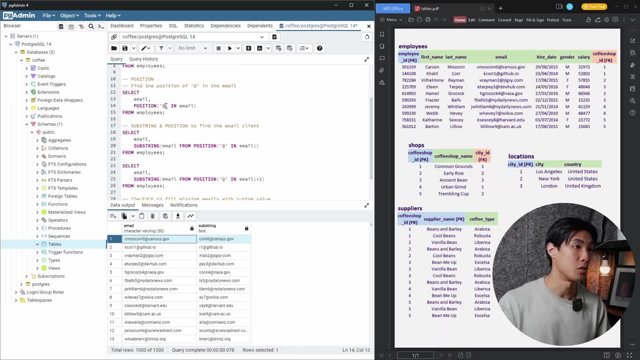 And in this case we are going to find the position of the app in the email column, So let me just use that, run the query And you can see that in cmosconi zero at censusgov, the at is at the 10th position, so the 10th character. And then in kcore1 at githubio. 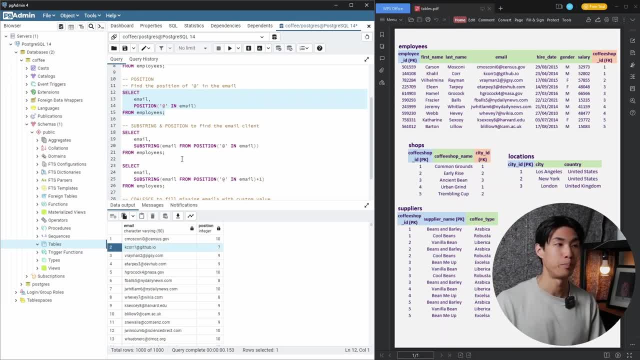 the at sign is at the seventh character. Now next up, let's do something a little bit more interesting and probably quite useful. So we'll combine the substring and the position functions to find the email client for each of the employees. So what we'll do here is within: 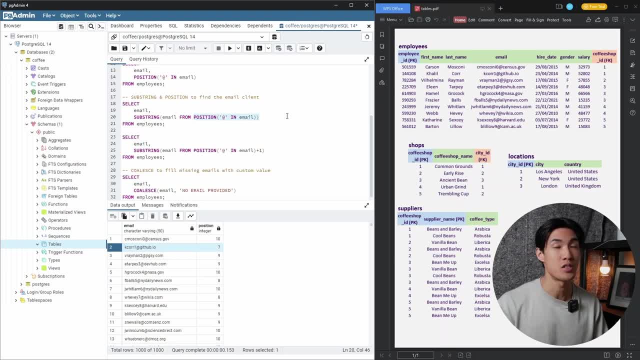 the substring function. we'll actually use the position function to find the position Of the at sign And then we'll just say substring email column and then from this position. So it's dynamic because it'll find it for us. Let me just pass this in and let me run this code. 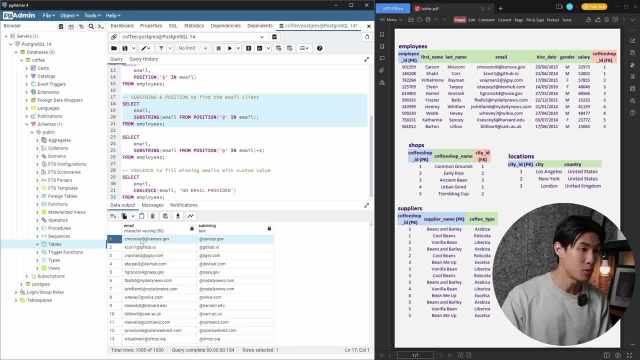 So you can see now that in the first row, instead of cmosconi, zero at censusgov, we only have at censusgov. And then if you look down this column, you can see that basically these are all the email clients. Now, this is probably still not the best way, because you can still see the 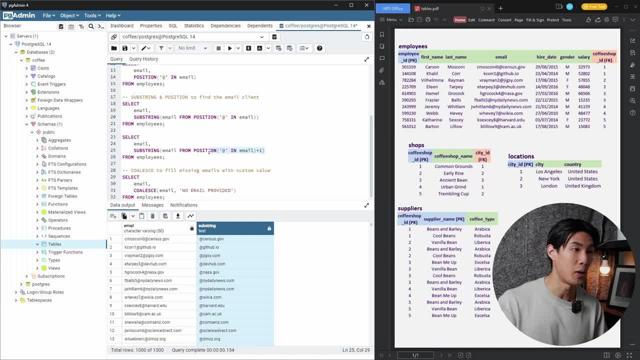 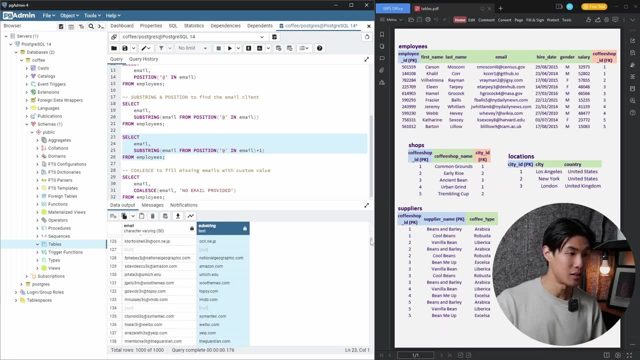 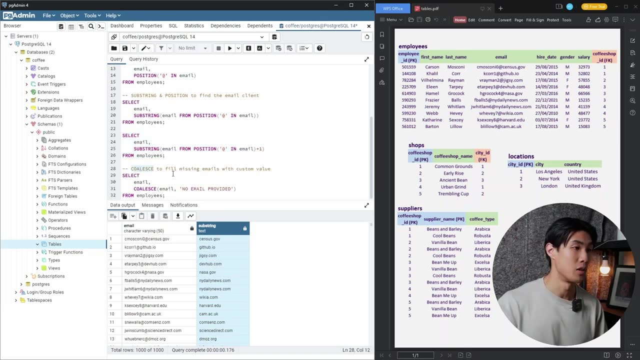 at sign. So to get rid of that, you just need to add one to the position here- And let me just do that- and run the code again And you can see that now it's nice and clear. you only have the actual exact email client returned. So the next one will be the coalesce function, which is used. 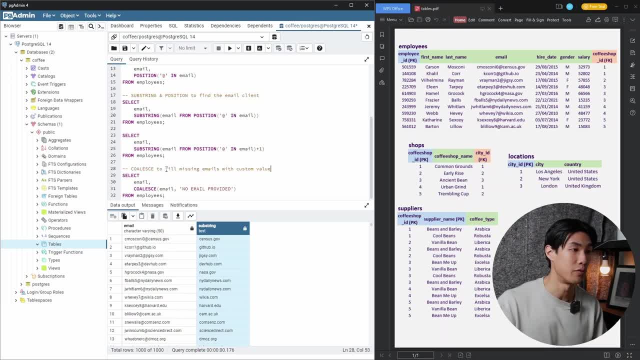 to fill missing values with a custom value. So we'll fill the missing emails with a custom value that we specify, And in this case I will specify this custom value as no email provided. So this is a very simple function. you just pass in the function name which column you want to. 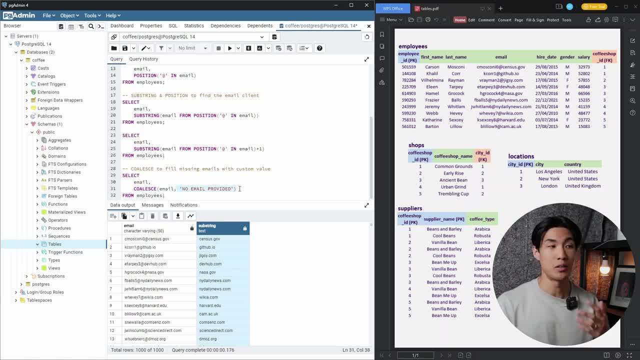 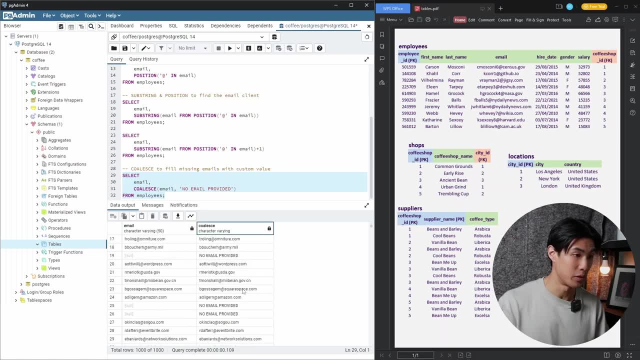 apply this on and then whatever value you want to fill the missing values with. So let me just do that. And now you can see that all of the empty emails will be filled with no email provided. So row 19,, row 25,, row 26.. Let me find another one. There we go row 42.. Okay, so now that we've 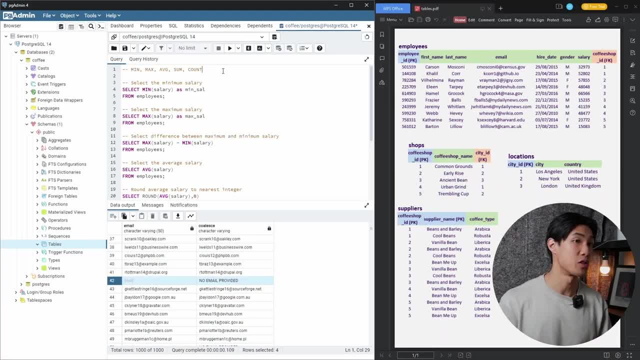 covered a bunch of string functions. let's move on to some functions, some numerical functions. We'll cover min, max, average sum and count. So let's first of all select the minimum salary. this is really simple. So the function is min. you pass in the column name. I renamed this column as: 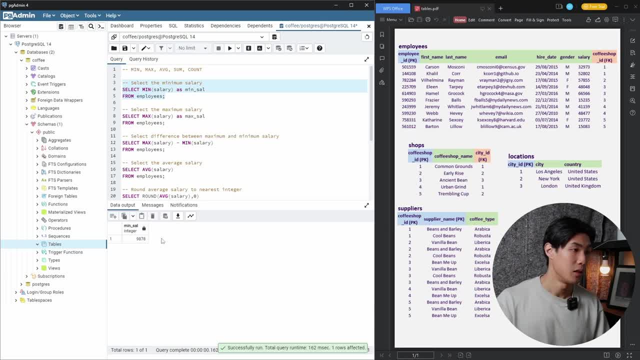 minimum salary from employees. And let me run this And we can see that the minimum salary is $9,878.. Again, you can find the max salary as well using the max function. So if I run this, you can see that the max salary is $67,724.. Now we can do some. 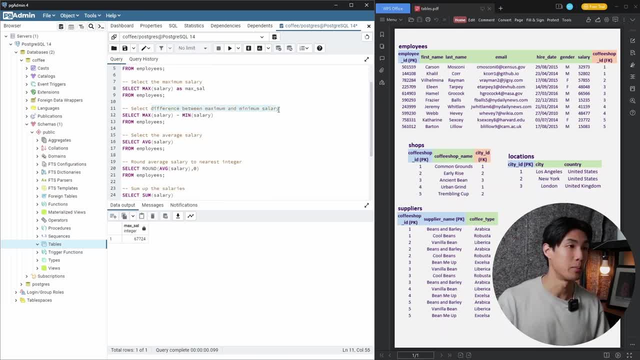 arithmetics as well. So let's select the difference between the maximum and the minimum salary. So max sell minus the minimum salary from the employees table. Let me run this And then you can see that the difference is $57,846.. You can use the average function to find the average. 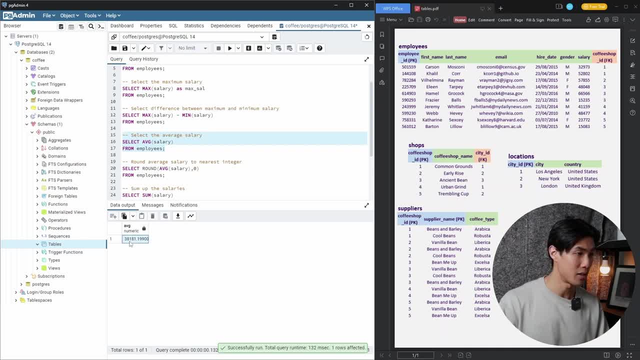 salary. So if I run this you can see that the average salary is $38,181.. But this looks quite ugly with all the decimals. So we can use the round function round this average salary to zero decimals. So I'll do that And when I run the query, 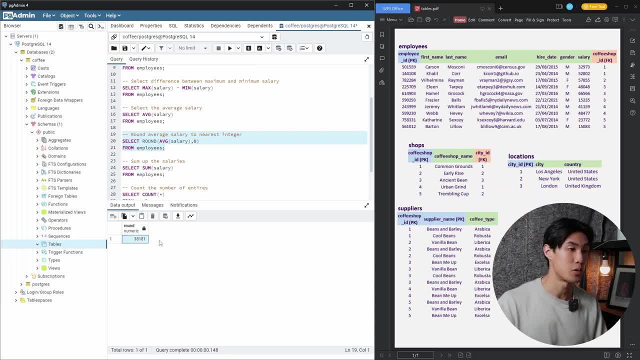 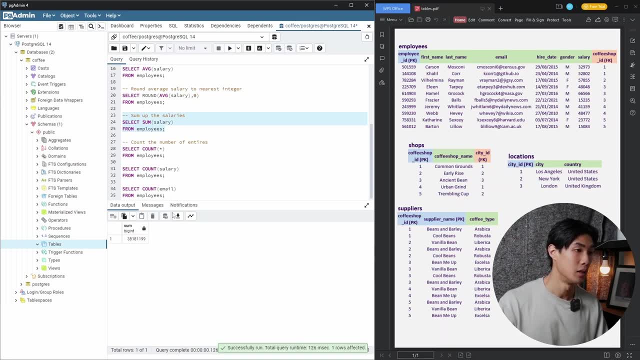 you can see now that it only returns $38,181.. So, next up, you can use the sum function to sum up all of the salaries, which is what I'll do now, And you can see that this is the total of the salaries. Now you can use the count function to count the number of the entries. 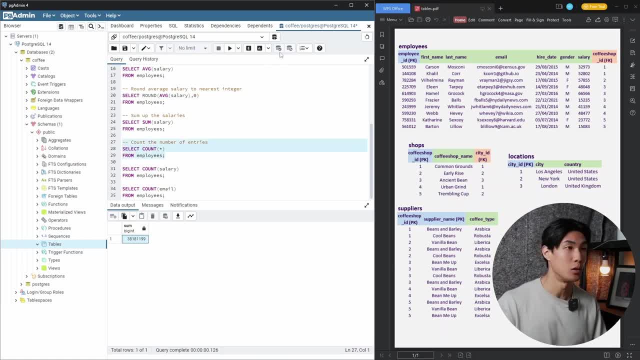 So let me just do that. So count star, which is counting all of the rows, everything, and then you can see that indeed, in the employees table we have 1000 rows, so we have 1000 employee records. Now I could count on a different column, so the salary column only, and then you see. 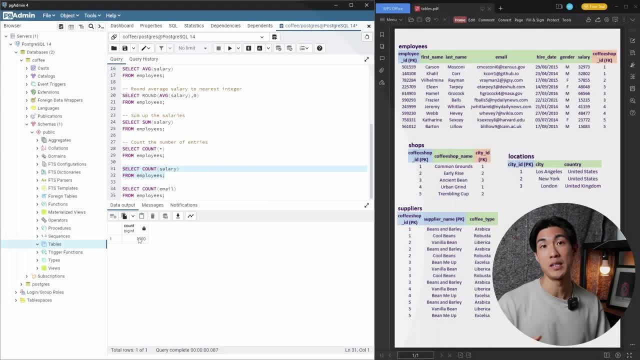 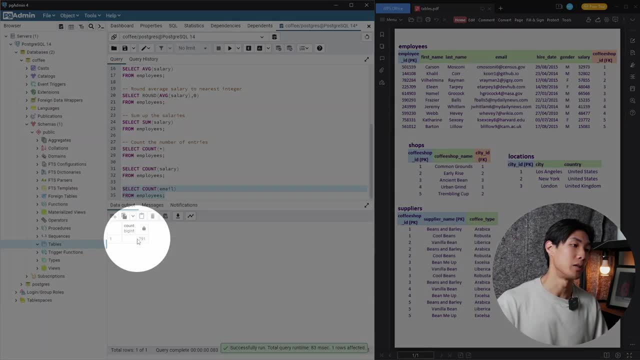 that we have 1000 salary values, So there's basically no missing values in the salary column. But again, if I count on the email column, you'll see now that we only have 791 values, which is correct because we do know that we have missing values in the email column. 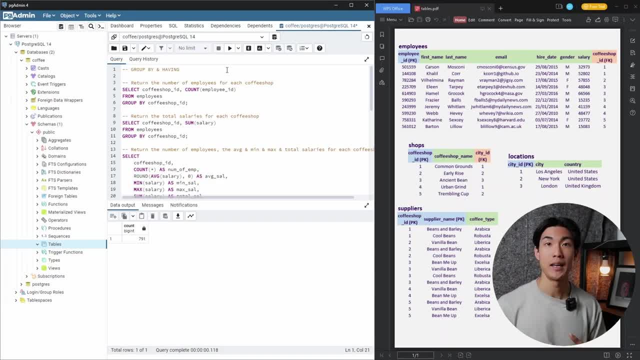 We're doing really well. let's move on to group by and having. So we'll use group by to group by, first of all, the coffee shop ID within the employees table to find out the number of employees for each of the coffee shops. So let's do that first, So I will select the coffee shop. 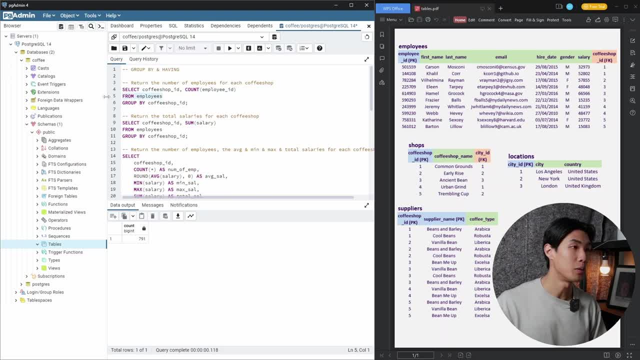 ID and then I will count the employee ID from the employees table And then I will group by the coffee shop ID. So if I run this bit of code here, you can see now that coffee shop ID one has 7 employees, coffee shop ID 3 has 214 employees, coffee shop ID 5 has 203 employees. Now, whenever 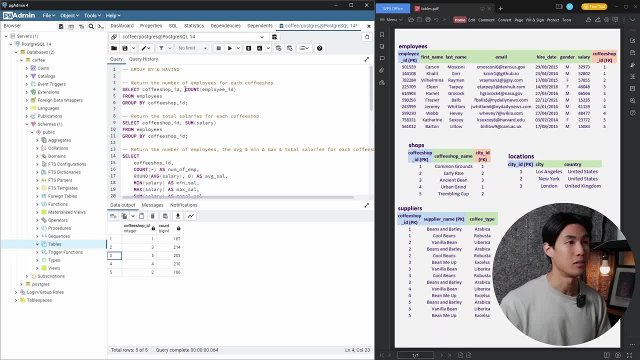 you use an aggregated function, so like count, sum, min, max, average. here within your select statement you're always going to have to group by whatever column you pass in here. So this coffee shop ID has to appear here and here as well. Now let me show you why, Because say for example: 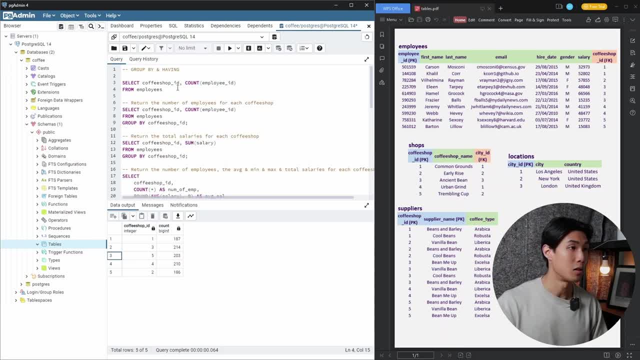 if I only run this bit of code here. so let me just copy it here. you'll see that this won't work. There we go. SQL actually gives us an error message and it tells us what we're doing wrong. So it's saying that columns employeecoffeeshopID must appear in the group. 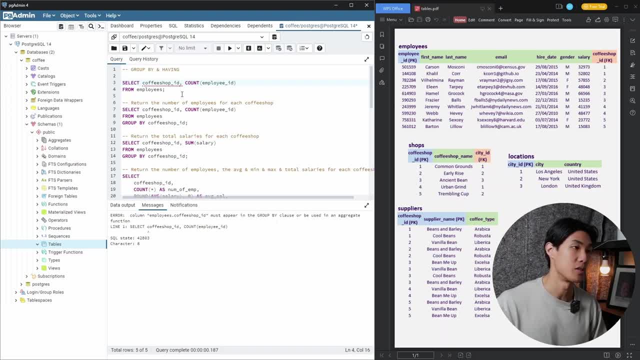 by clause or be used in an aggregate function. So that's why we're using group by here to group by the coffee shops. Now, next up, we can return the total salaries for each of the coffee shops. So I am selecting the coffee shop ID, I'm summing up the total salary. 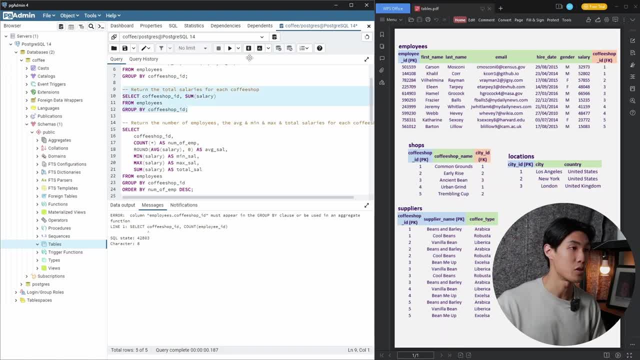 From the top, I'm going to add the total salary. So I'm going to add the total salary From the employees table and again I'm grouping by the coffee shop ID. So there we go, And you can see that now we have the total salary for each of the coffee shops Next up. let's do something a little. 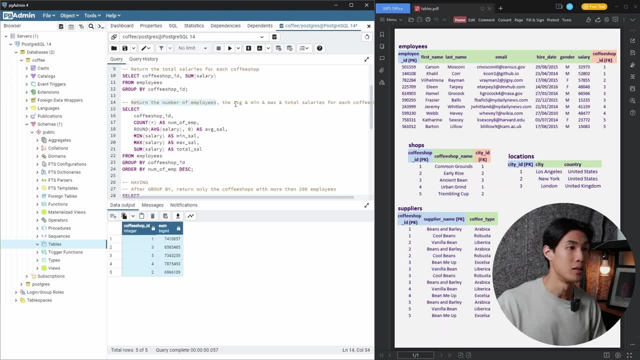 bit more complicated. So let's return the number of employees, the average, the minimum, the maximum and the total salaries for each of the coffee shops. So again, we select the coffee shop ID column, we count everything and we'll name this column as the number of employees will round the. 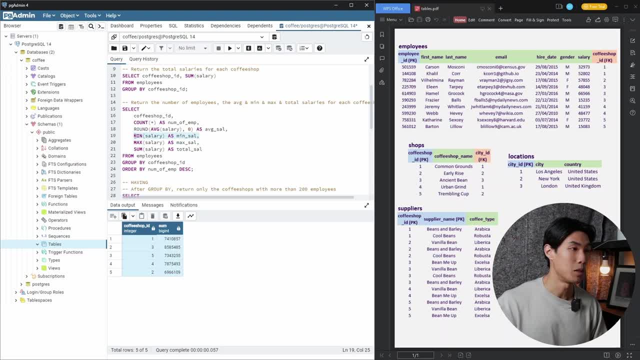 average salary And then we'll return the number of employees, the average, the minimum, the maximum and the total salary to zero decimals. We'll select the minimum salary, the maximum salary and then the sum of the salaries from the employees table And then we'll group by the 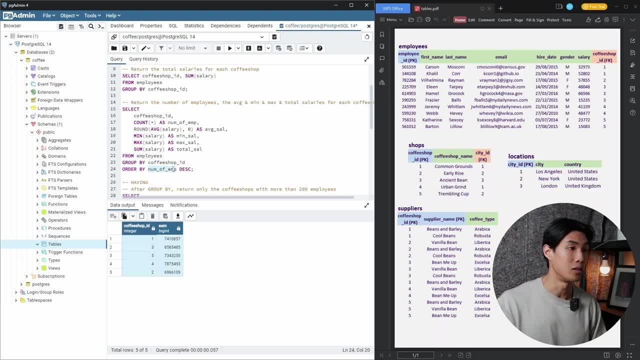 coffee shop ID And then finally, we'll order by the number of employees descending. So let's run this query here And we can see that coffee shop ID three has the most number of employees: 214.. It's got an average salary of 40,119 and a minimum salary of 10,592.. 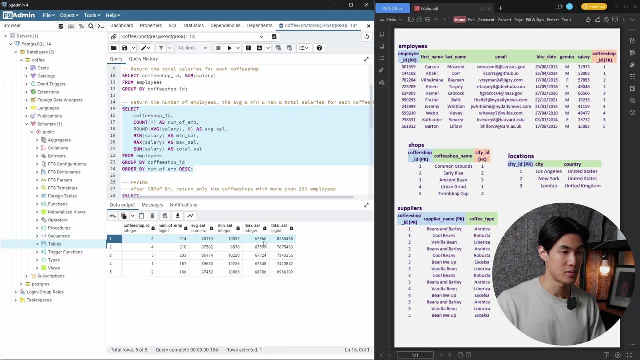 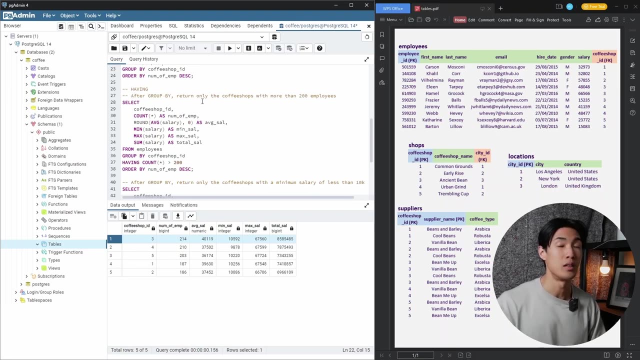 with a max salary of 67,560.. And the total salary, I believe that's $8,585,485.. So next up let's use the having clause. So after group by, you must use the having clause. you cannot actually use the where clause anymore, So it's kind of just a special where clause that. 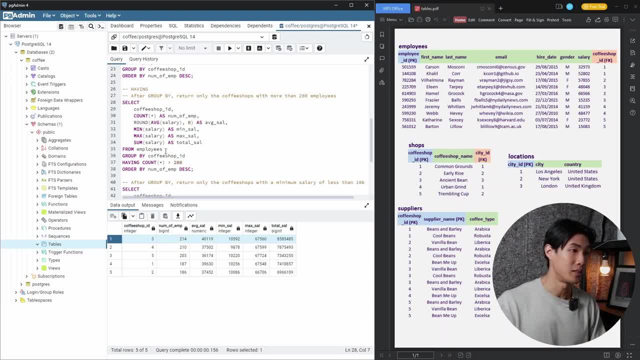 you use after the group by. So again we have the exact same query all the way until the group by coffee shop ID here, And then we have the same query all the way until the group by coffee shop ID here. the only thing that's different is now we're seeing that halving, so it's kind of just a filter. 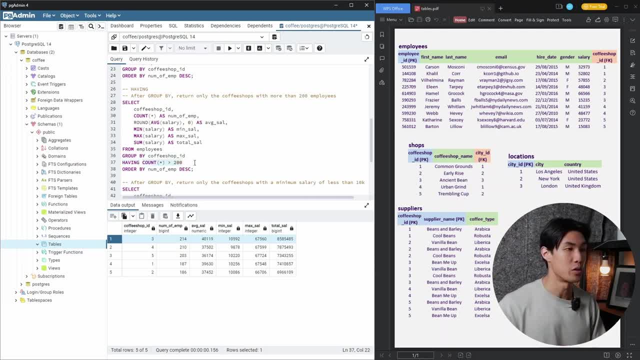 so we want all of the coffee shop ids with more than 200 employees return. so we're saying count star is greater than 200. so let's see what we get now. so you can see that if i look into the number of employees column we have 214, 210 and 203. so we've only returned the coffee shops that have. 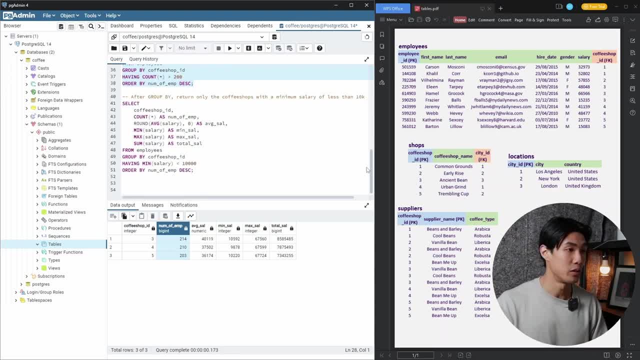 more than 200 employees. now let's move on to another query. we can also return only the coffee shops where the minimum salary is less than 10 000, so let's do that. let me just select this. and now, if you look into the minimum salary column, we actually only have one coffee shop where the 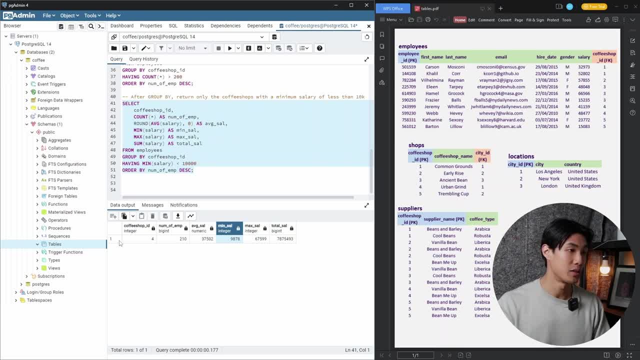 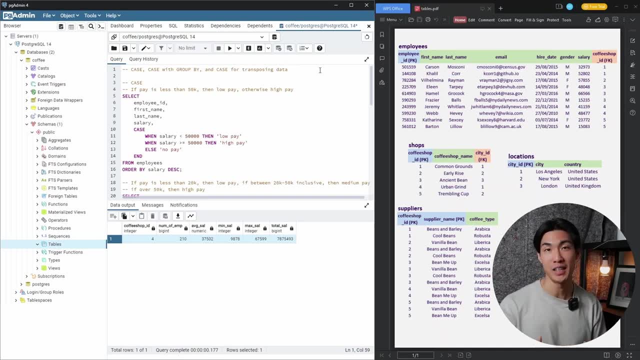 minimum salary is less than 10 000. so this is coffee shop id 4.. okay, we're almost at the very end. let's move on to some case statements, and we're also going to combine these case statements with group by, and then we're also going to use case. 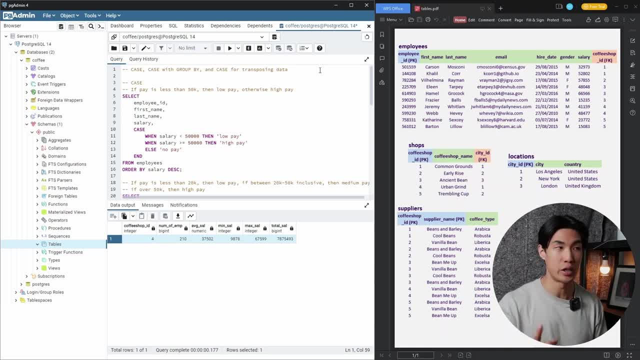 statements to transpose our data, which is going to be pretty cool. so let's start out with the basic case statements here. so case statements are kind of like if statements, and first of all we're going to say that if the pay is less than 50 000, then give me low pay, otherwise give me high pay. so i 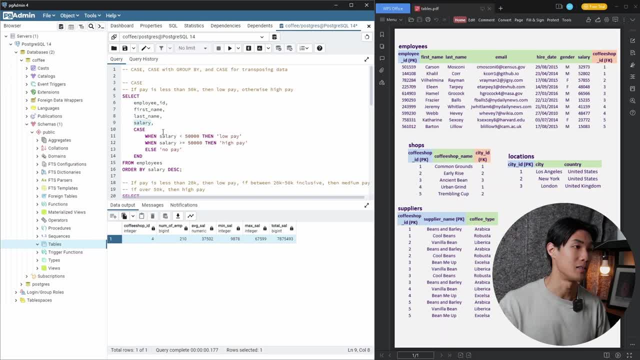 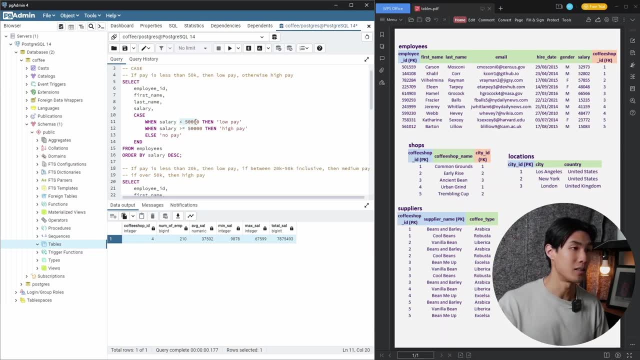 am just going to select the employee id, the first name, the last name and the salary columns, and then i am going to use a case statement. so i'm saying case, when the salary is less than 50 000, then give me low pay. it reads just like english, in my opinion. 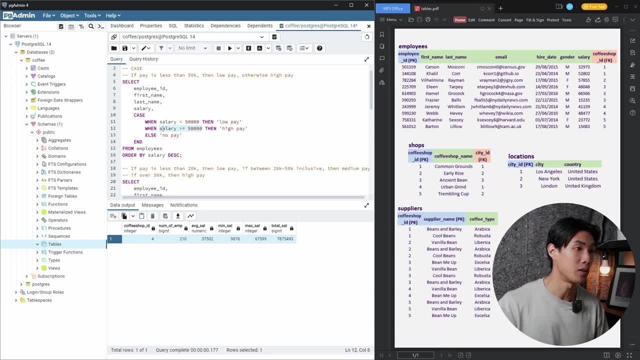 so when the salary is more than or equal to 50 000, then give me high pay, else no pay. in this case, else is not really needed because we've pretty much covered all of our bases. the salary can either be less than 50 000 or equal to 50 000 or more than that, and then make sure you end. 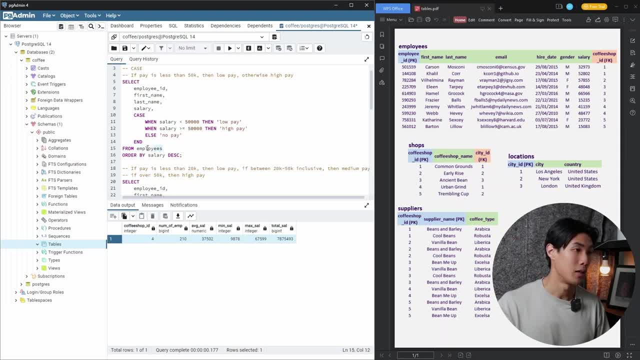 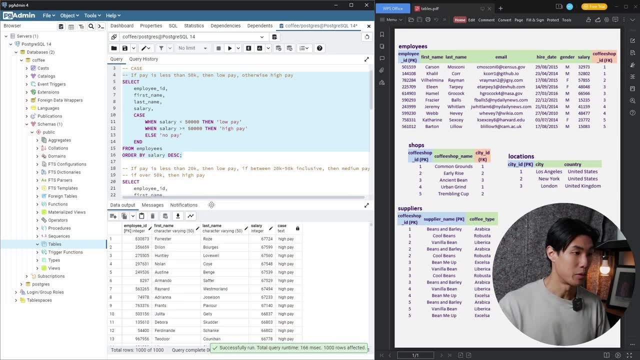 your case statement with the end keyword, and this is from the employees table, and then let's just order by the salary descending. so let me select this, let me run this query and you can see here that if i look into my case column here you can see that obviously i'll only 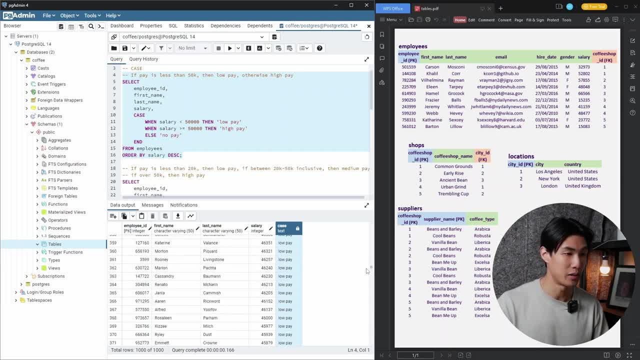 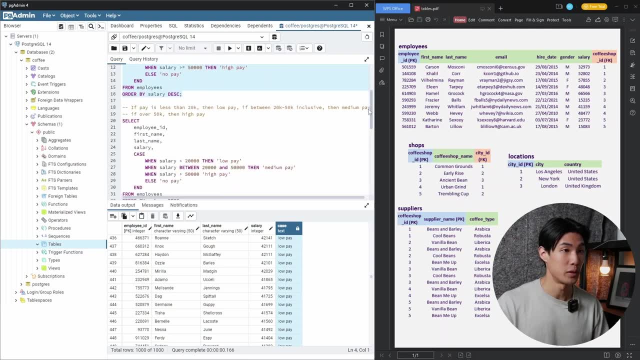 have the high pays first of all, and then, if i scroll further down, once i hit below 50 000, i will actually only get the low pace. now let's move on to another case statement. let's introduce another condition. so now i'm saying that when the salary is less than 20k, give me low pay. when 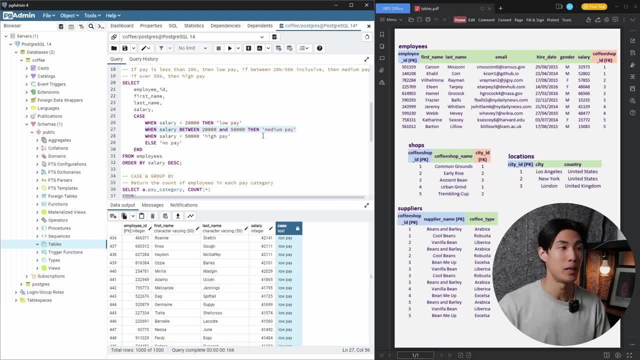 the salary is between 20k- and i'm going to increase the salary a little bit more, and then you need to- and 50k, give me medium pay, And when the salary is above 50k, give me high pay, else give me no pay. 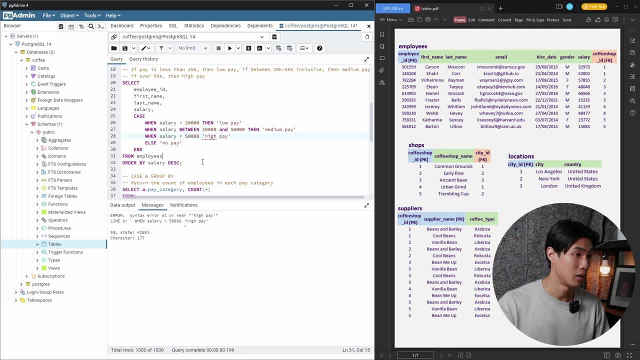 So let me just select this, let me run the query, And something didn't work here because I'm missing a then keyword here. So let me just run this again. And here we go. Now you can see that if you look into the case column, you have high pay, And then, as I scroll through it, I have 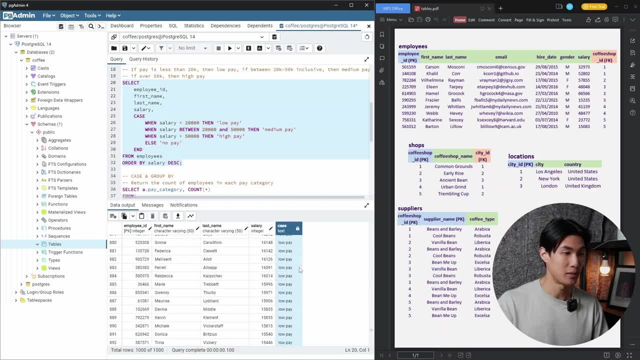 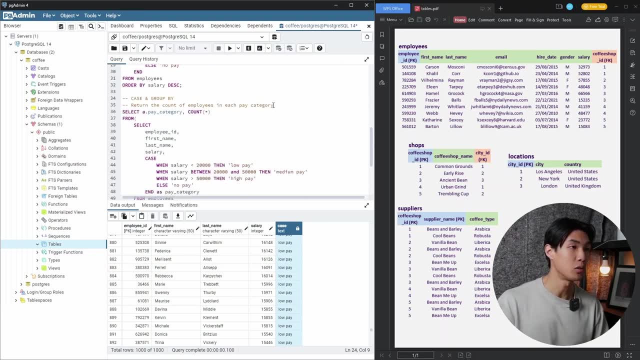 medium pay between 20k and 50k, And if I scroll to the end I only have low pay. Okay, so next up we'll use a case and group by to return the count of the employees in each of the pay categories. 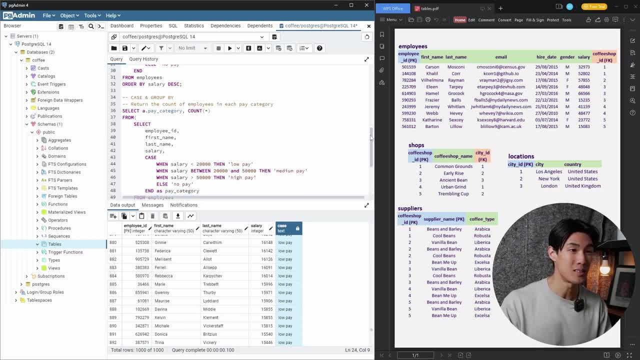 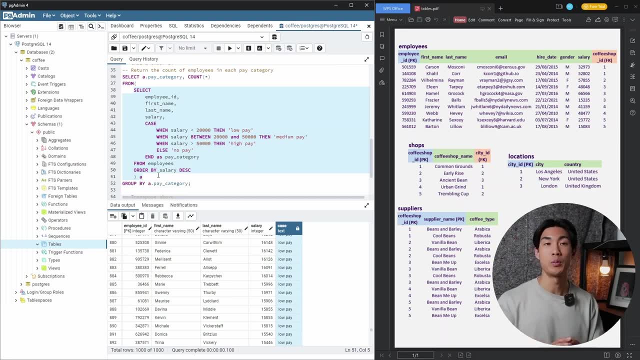 that we create with the case statement. So this is a bit more complicated query And actually we have a sub query right here running within this query. But don't worry too much about the sub query. we're going to cover this in the next section. So for the purposes of this query, 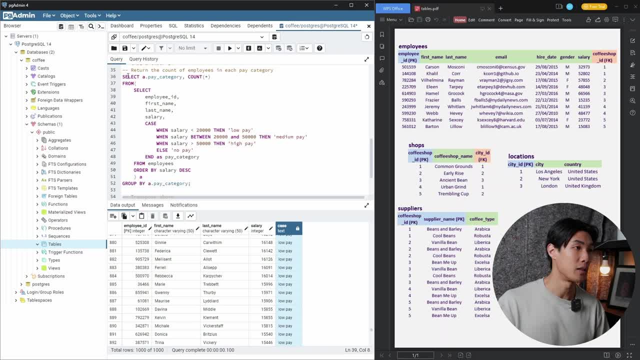 just focus on the case statement. So all we're doing here is we're selecting the pay category from this a table. So this a is just an alias. So you see here, this is my query and I created an alias for this query. So I'm. 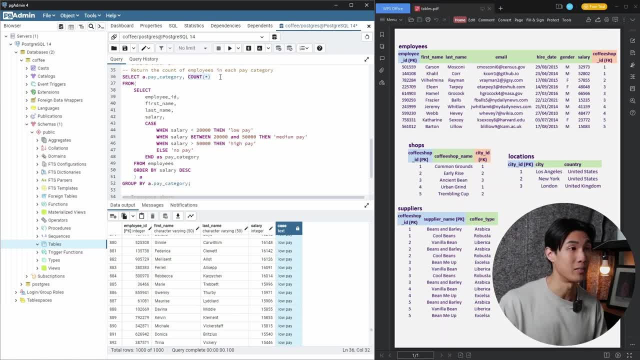 selecting the pay category from this query And then I'm counting everything within this query And then finally I'm just grouping by the pay category. So the pay category is just this case statement here. So all I said was the same as before. So give me low pay, that medium paid and 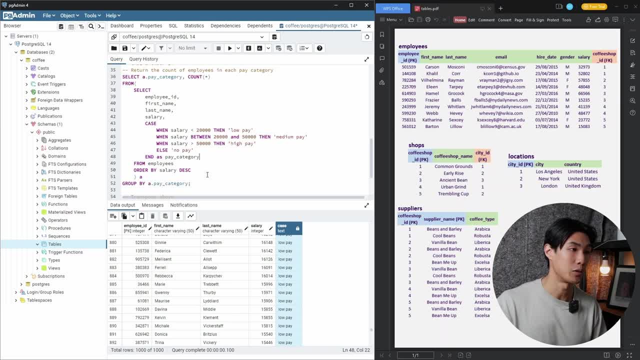 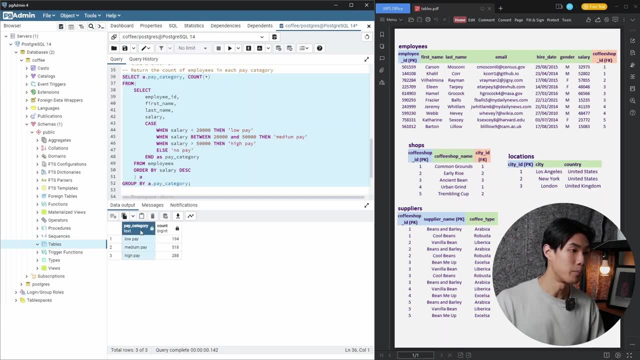 give me high pay And then call this column as pay category. So let's see what happens when I run this code here. So you can see, now that I have the pay category here, And then I have the number of employees within each of the pay categories And this is how you can use the case. statement with group by. 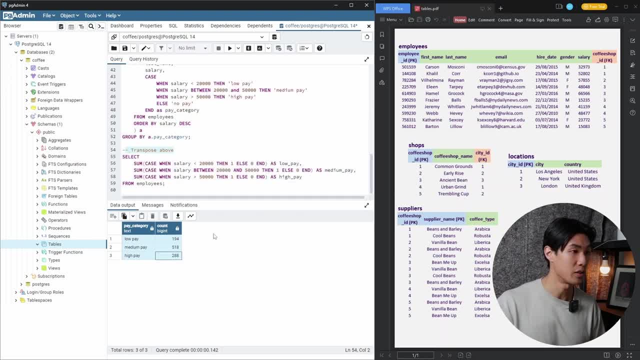 Okay, next up, another cool thing. So we'll transpose our data. So we will transpose this bit of data here. transposing is just turning the rows into columns. So we will select sum case. when the salary is less than 20,000, then give me one else, zero. So basically we're just. 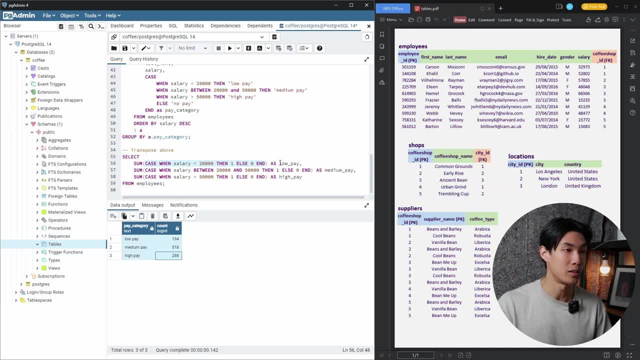 going to count the number of employees and then return this as low pay, And then we'll do the same, but this time we're counting the employees where the salary is between 20,000 and 50,000.. So give me the one that's the count and that we just add them up, And then, finally, we have high pay Again. 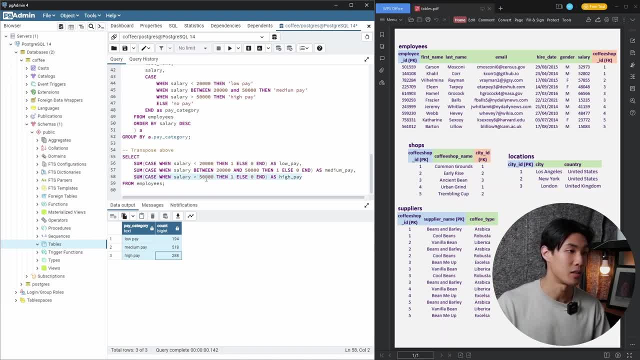 we do the exact same thing, but for the salaries over 50,000.. So if I run this code here, you'll see that now the bottom bit, so the low pay, the medium pay and the high pay will turn into columns. so let me just run this query here and you can see that we have successfully transposed. 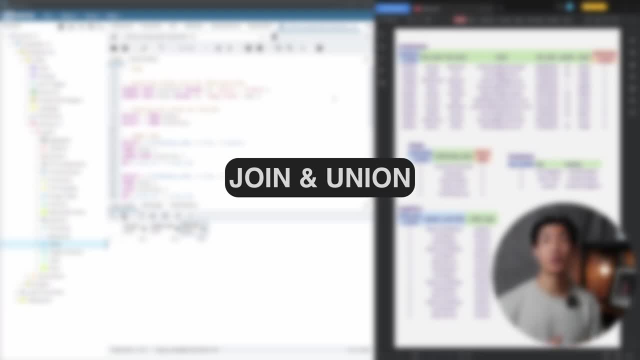 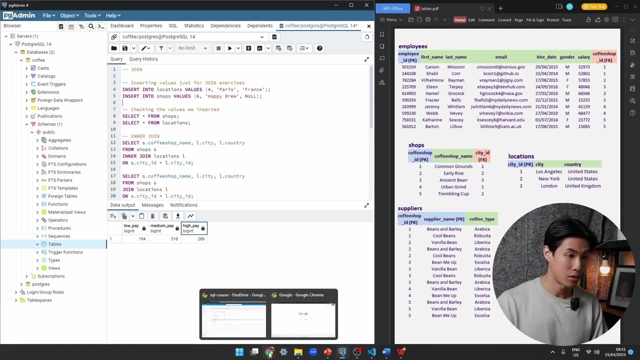 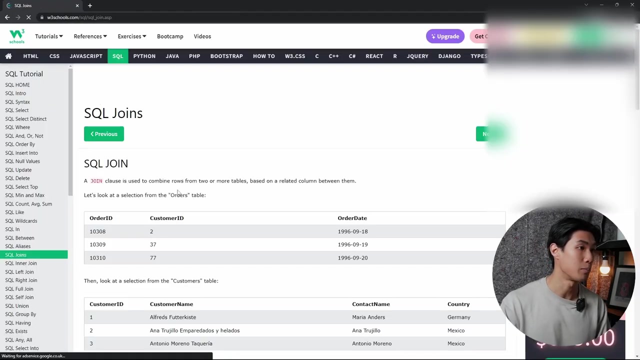 our data all right. next up, we are going to work with multiple tables using joins and unions. but before i go into the joins here, actually let me just go through some some theory around the joins. so i'm just search something on google: w3 schools- yep, that sounds good to me and let me just 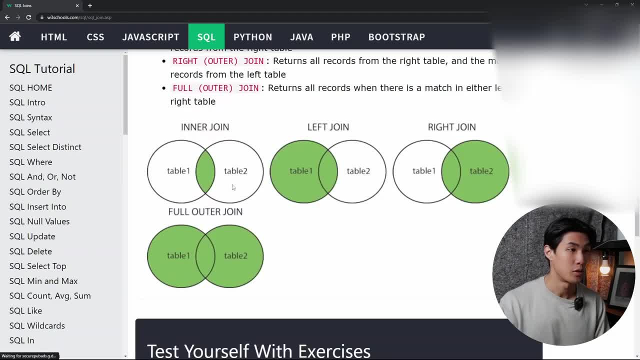 find an illustration here, so let me scroll here. so essentially we'll cover inner joins, which is basically just the intersection of the two tables: left join, so everything from the left table, even if it's missing in the right table, and then right join will take everything from the right. 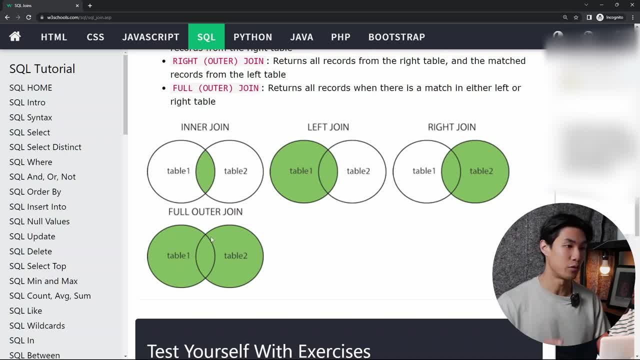 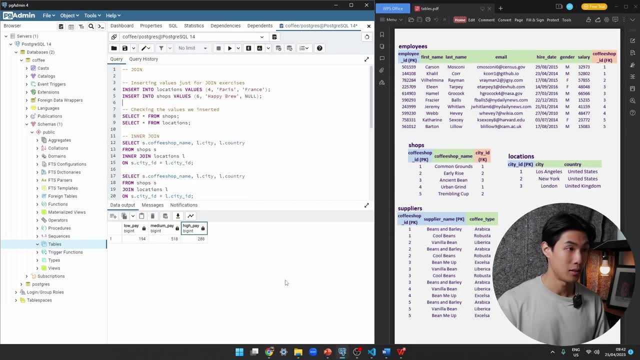 table, even if it's missing in the left table, and then the full outer join will just basically give you everything. so let's jump back into our exercise and here we go. so first of all, let me just insert something: values just for these join exercises. so i am going to insert values into the locations. 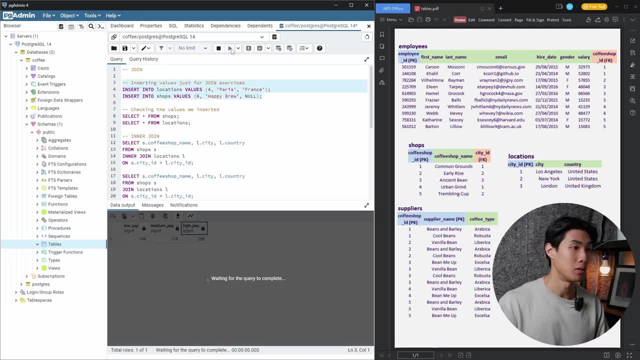 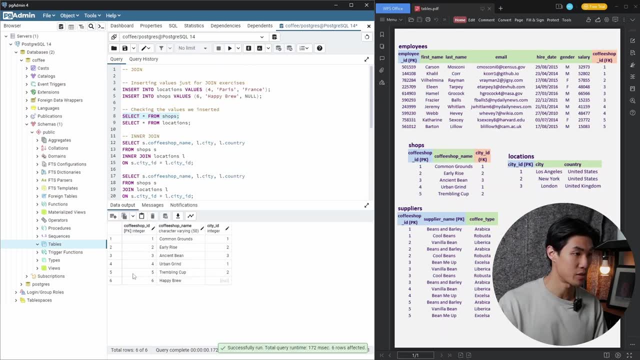 and the shops tables. let me just do that, run the code and there we go. the query was returned successfully. now let's check the values we inserted. so i'll select everything from the shops first, and you can see row 6 here. happy bro, the city id. i on purpose left it as null and then let 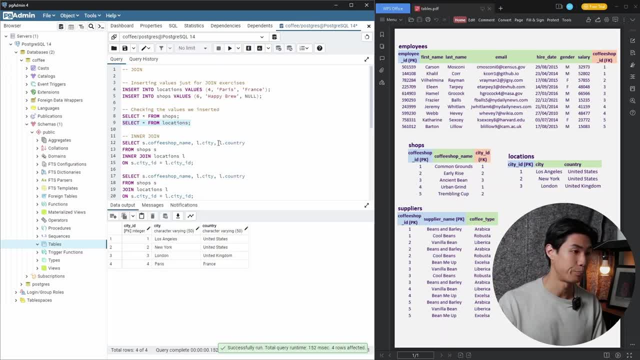 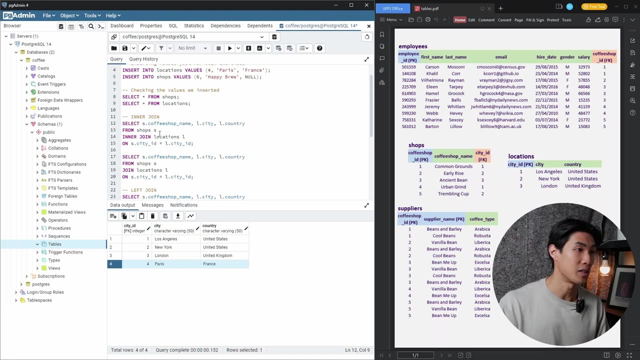 me look into the locations table, select that, and you can see that now we have a fourth location, which is in paris, which is in france, obviously. so first of all, let's do the inner join. so i am going to select scoffeeshop name- and this s is just an alias for the shops table- and then i will select lcity and 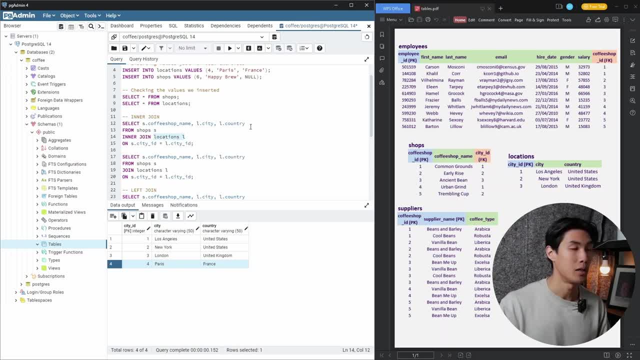 l again is an alias for the locations table and i will also select the country column from the locations table and then i'm saying inner join locations l. so basically i am inner joining on the scity id, so the shopscity id and then the locationscity id. so let's have a look at our shops. 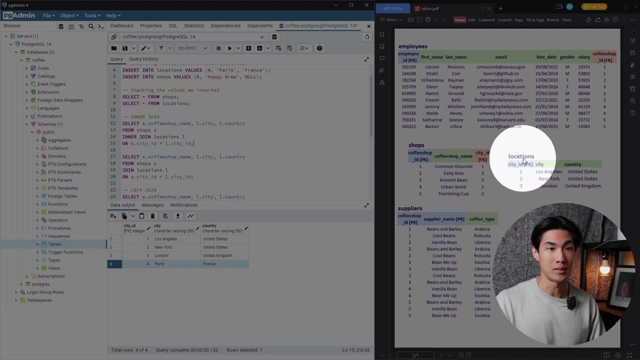 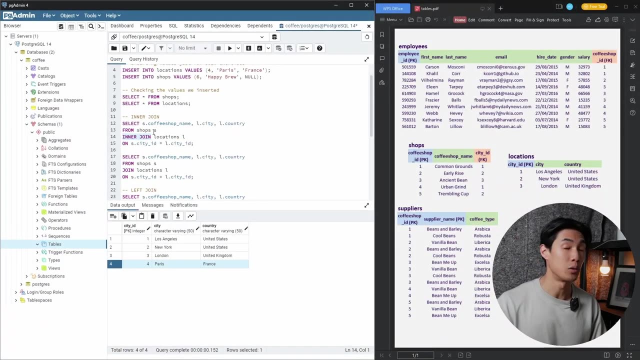 table you can see that city id is the foreign key and then we can see that in the locations table the city id is the primary key. so basically, this is what we're joining on, and inner join or join is exactly the same. so by default, sql just assumes that you're doing an inner join. so 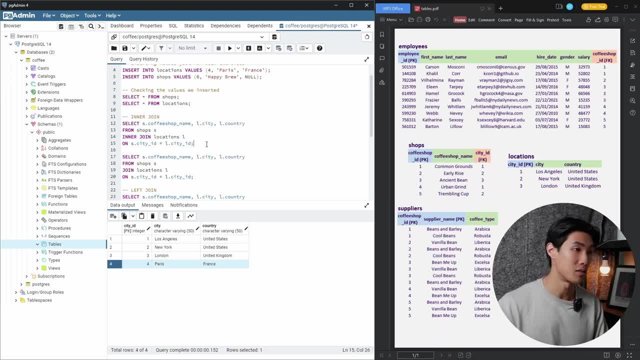 if you pass in join or inner join, it makes no difference. so let me just run this code here and you can see now that we've combined these tables, we've joined these tables. so we took coffeeshop name from the shops table, then we took city from the locations table and then we also took 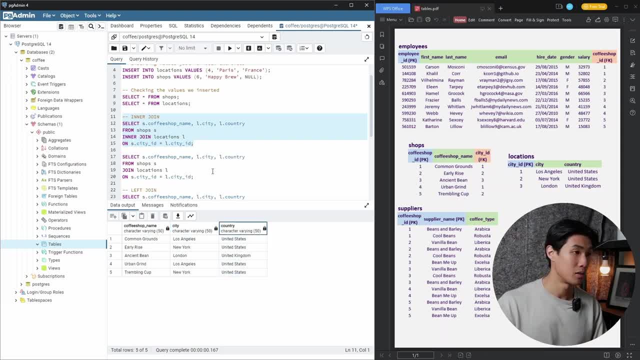 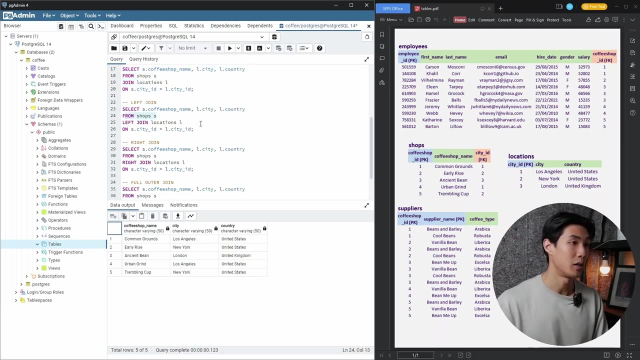 country from the locations table. so next up, let me just show you that join is exactly the same as inner join. let me run this code and you can see that this table is exactly the same as before. now let's quickly do a left join. so this time i'm joining the shops table and the locations table. 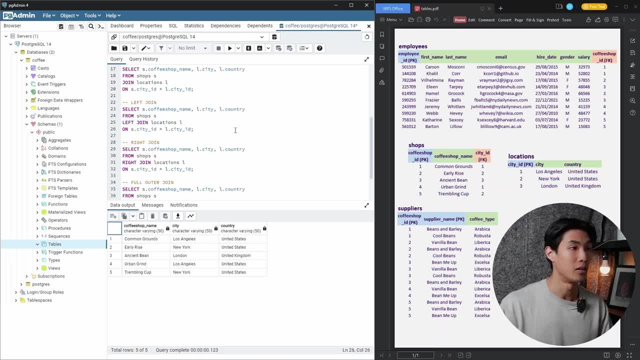 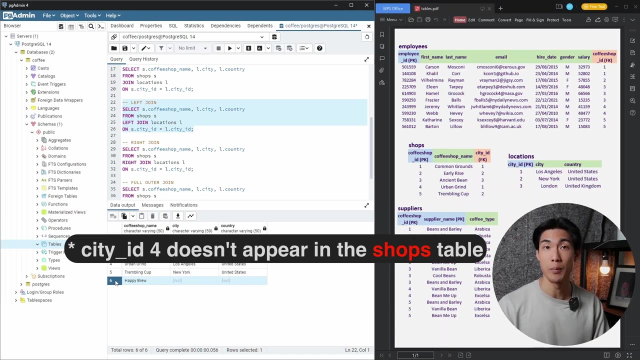 but this time i'm left joining the locations table on the city id. so let's see what happens now. let me run this code here and you can see that we took everything from the shops table, so we took happy brew, even though city id 4, which is paris, doesn't appear in the locations table. 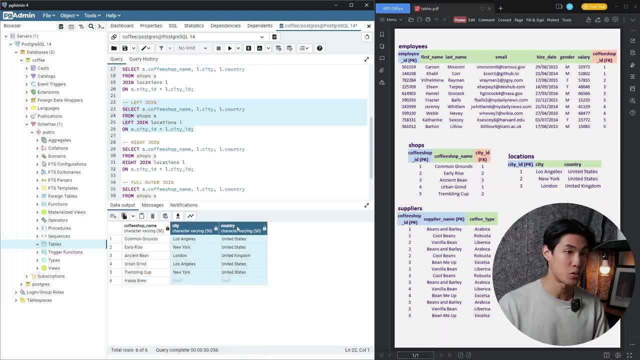 so there you go. you see the city is null here, and then the country is also null. so there we go. this is left join. we're taking everything from the left table. now moving on. we're going to run the city id table table now moving on to right join. so this time again it's the same query, but this time we're. 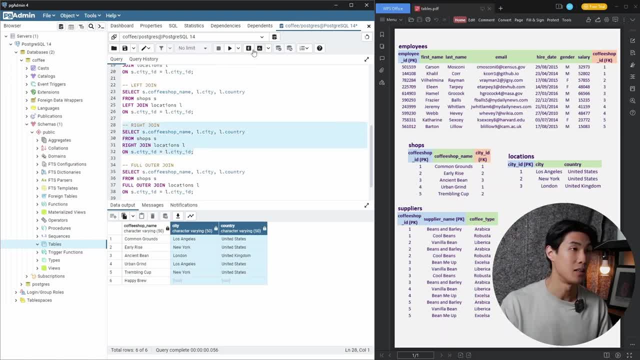 right joining the locations table. so let's see what happens now. so you can see that this time, what's happening is that we're taking everything from the right table, so the locations table, and you can see that we have paris in here. indeed, so row 6 for the coffeeshop name will be empty. 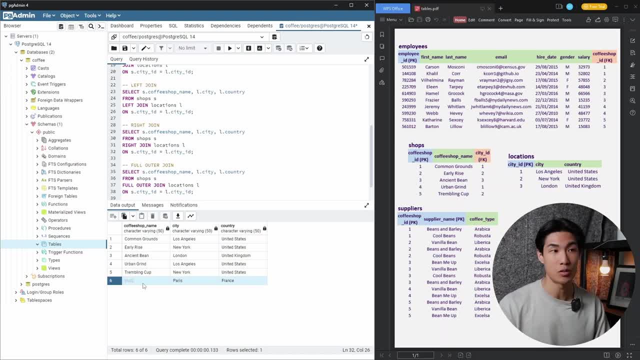 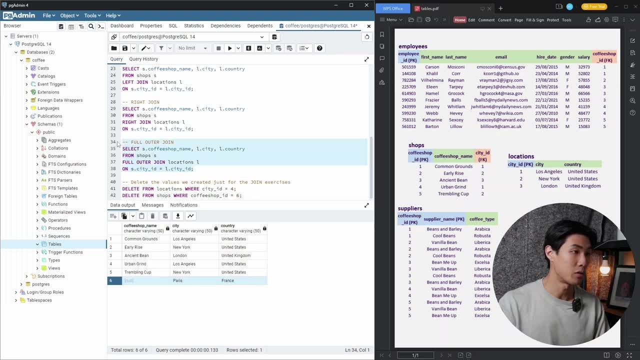 because we're joining, we're right joining everything from the right table, even if the value is missing from the left table. and then, finally, let's do the full outer join here and then after that i will just delete the values that i created just for the join exercises. so the full outer join. 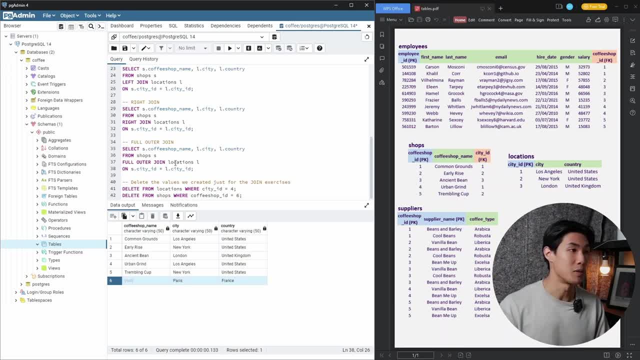 will just take everything. so if the value is missing from the right but in the left, it'll take that. if the value is missing from the left but in the right, it'll also join that. so again, we're joining on the city id and we're saying full outer join this time. so let me run this code. 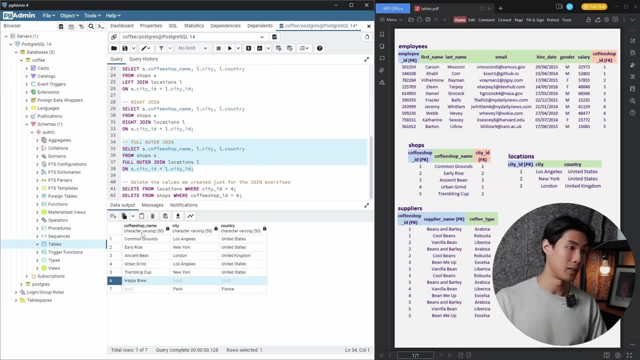 can see that we have everything. so we have the line with the happy brew coffee shop name, and then we also have the row of data where paris and france appears only in the locations table, and then, finally, i'll just run the delete from statements here, just to delete these two queries. 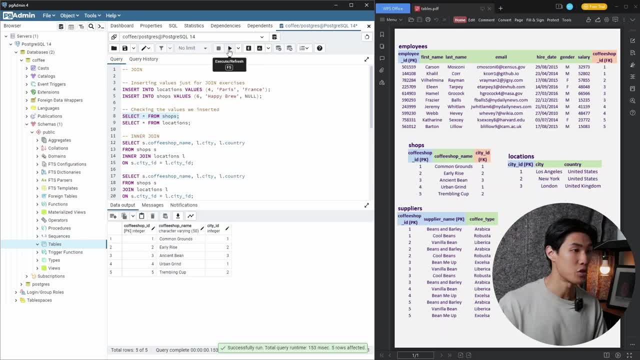 and i can show you that they have been deleted. so let me select everything from the shops and you can see that we no longer have the shop that i just created, which was- i actually forgot its name, and then, oh yeah, happy brew. there we go and then select everything from locations, so you 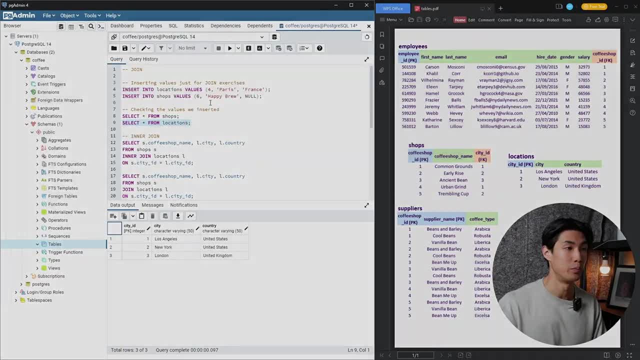 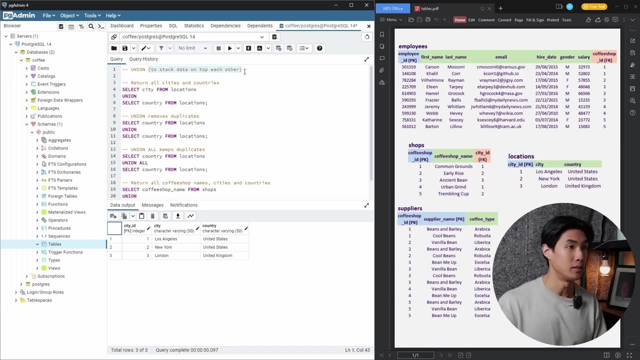 see that paris no longer appears in this table. now that we've covered joins, let's move on to unions, so you can use unions to stack data on top of each other. so, rather than joining data horizontally, you'll just be stacking data vertically. so let's return all of the cities. 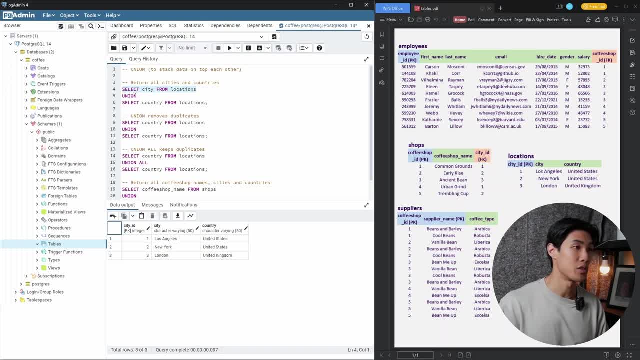 and countries. so we're selecting city from locations and then we're union in get with selecting the countries from the locations. let me just run that and there we go. you see that we have all of the cities and the countries. what you have to keep in mind is that. 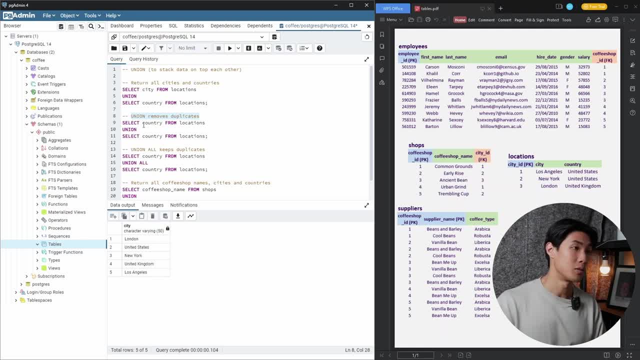 the union removes all of the duplicates. so say, for example, if i'm selecting country from locations and then i'm obviously selecting country from locations again and then i'm unioning these, you can see that i won't have duplicate values. so i still only have the united states and the united kingdom. 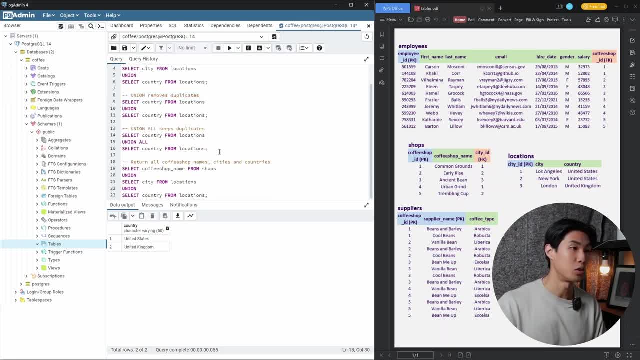 but you use union all. this will keep the duplicates. so let me run the same query, the only difference being union all rather than union. so when i run this, you can see that i have us- us- uk, us- us- uk, so we'll keep the duplicates. now we can obviously return all of the coffee shop names, cities and the 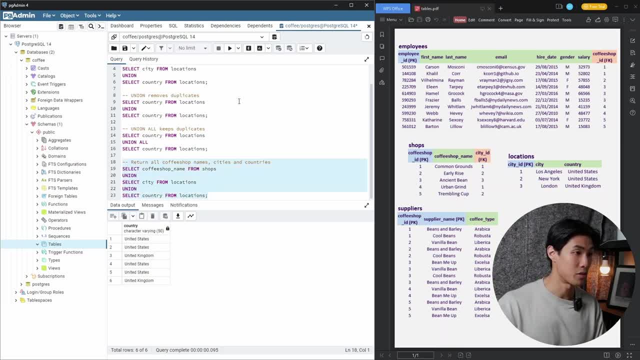 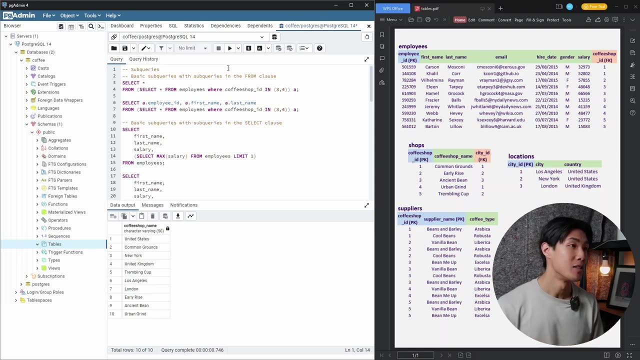 countries with the union statement here. so let me just run this bit. and now we have all of the coffee shop names, all of the cities and all of the countries and we used unions. well, it works on city and city, where you can see the not just cc data but also the other. 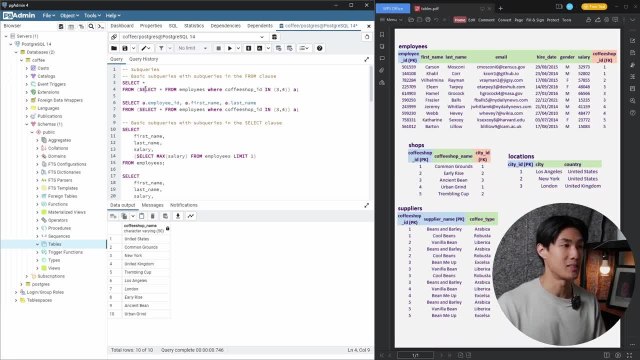 parallel properties. so let's run the same thing on the english comment into the barns from, and then i'm using this select statement again. so i'm selecting everything from the employees where the coffee shop id is in three or four, and then i'm aliasing this query as a 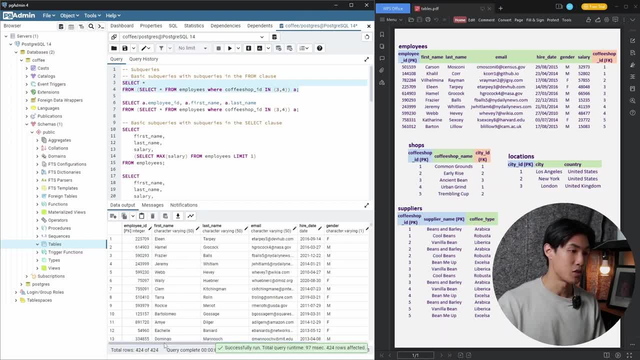 so let's see what this returns. and we can see that we just selected everything that was in the from clause. but of course we could use this alias a to specify which column names we would like to select. i'll only select employee id, first name and the last name columns. let me just run this. 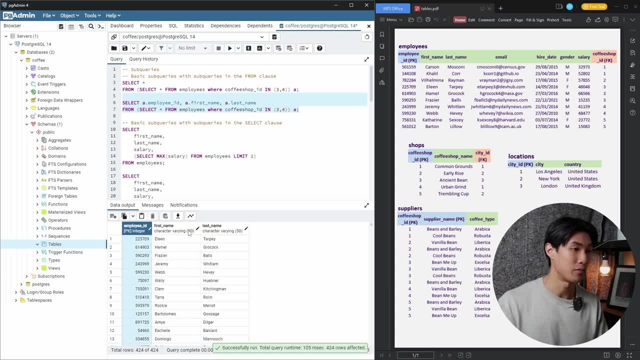 query here and you can see now that we only have employee id, first name and the last name columns selected. so let's move on to some sub queries within the select clause. so first of all i will select the first name, the last name, the salary and then i will return the maximum salary within. 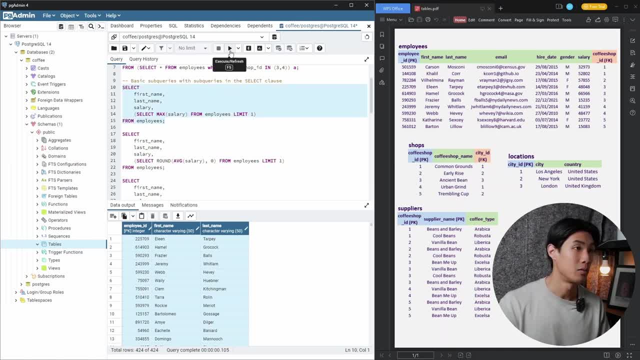 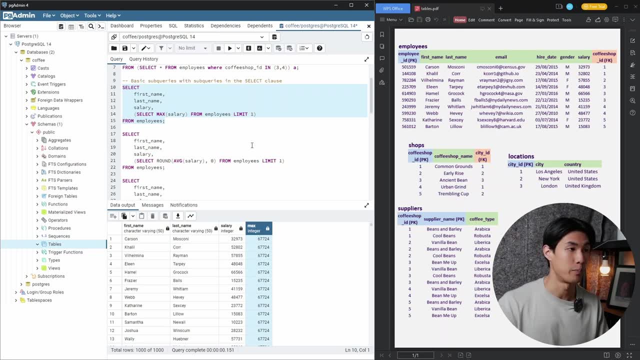 the entire table. so let me just do that: run this query here and you can see that we have the maximum salary returned for every single one of the rows here next up. we could do this, obviously, with the average salary as well, so we can select the average salary, which is rounded to zero decimals. 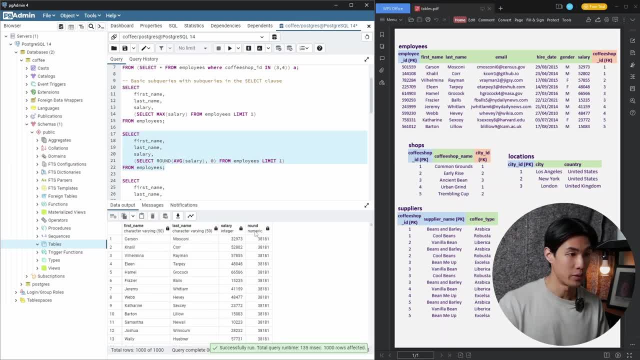 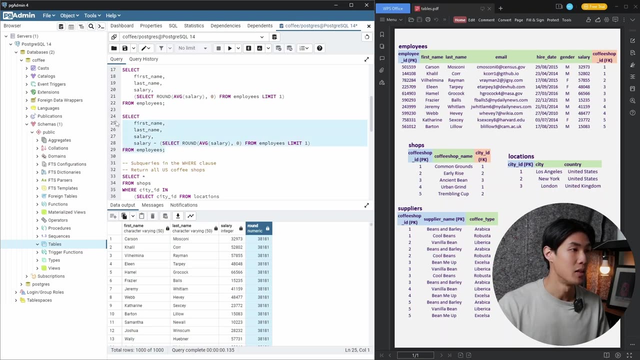 here and then let me just do that, and there we go. now, here you can see that the average salary is displayed in each and every one of the rows. now say, for example, you could do some calculations here so you could find the difference between the person salary and the average salary. so let me just 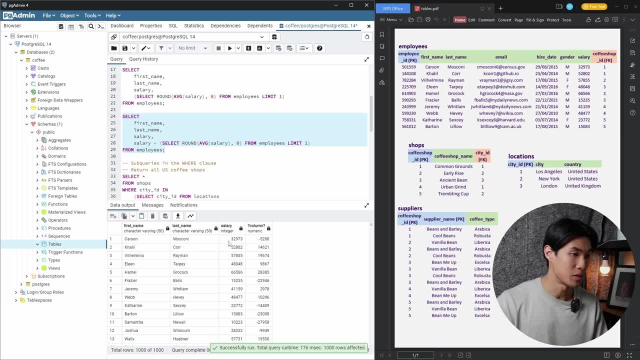 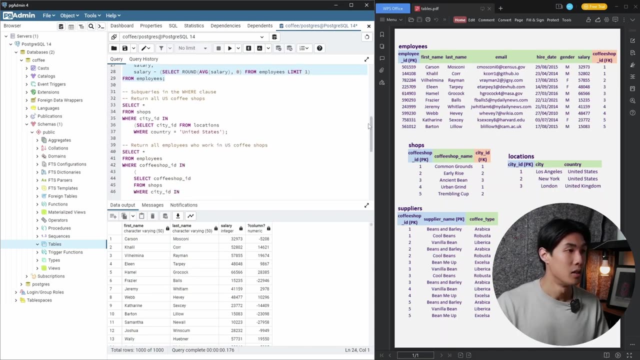 run this code here and then. now you see that carson mosconi, you know, the difference between his salary and the average salary is 5208, meaning that he actually makes less than the average salary. now next up, let's use some sub queries within the where clause. so how about we return all of the 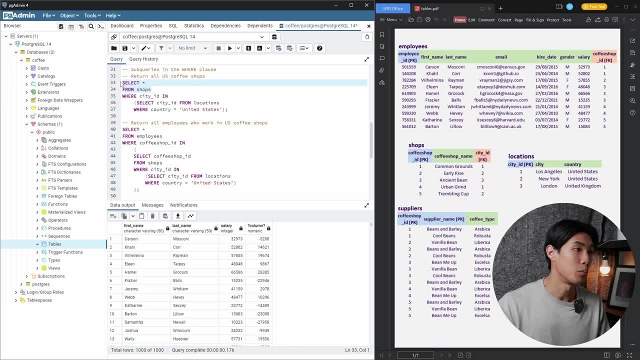 us coffee shops. so select everything from the shops and then where city id is in- and this is where we use a sub query, so i'm saying that the city id has to be in- and then i'm selecting the city id from the locations where the country is equal to united states. 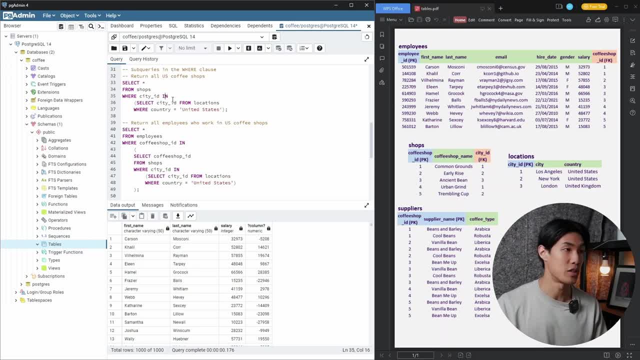 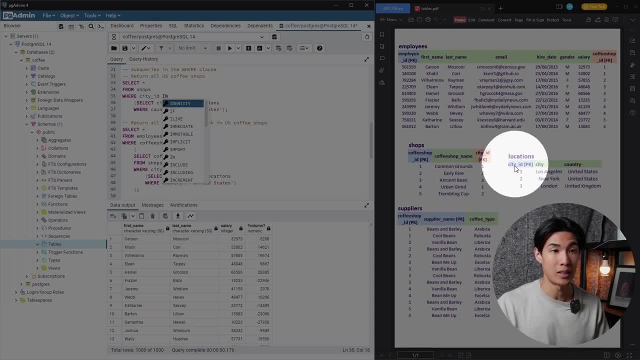 so we connect basically to the locations table using this query. so let's look at the shops table. you can see that the foreign key here is city id and then primary key in the locations table is the city id. so i'm saying that only select the city ids from the locations table where the country 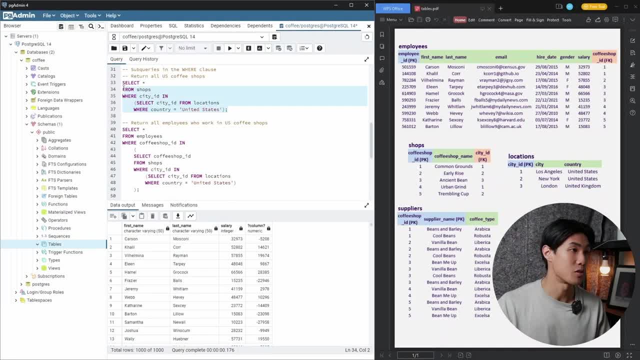 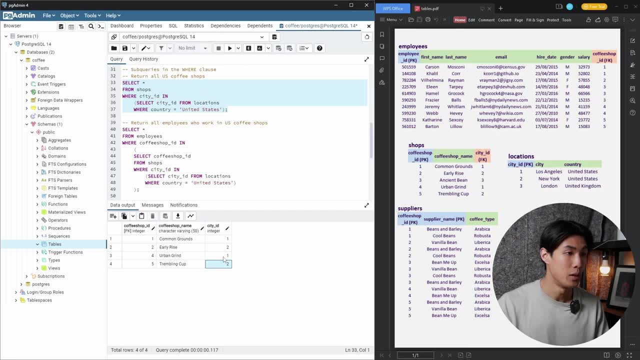 is equal to united states. so let me just run this query here and let's see what this returns. so now we only have city ids one, two, one and two. so if we go back to the locations table- and we're going back into the locations table- that is correct, because city id one is los angeles, which 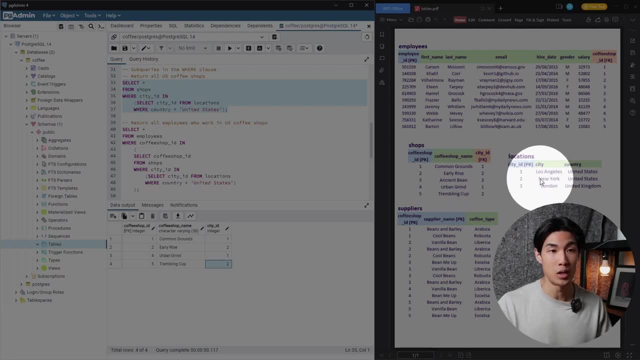 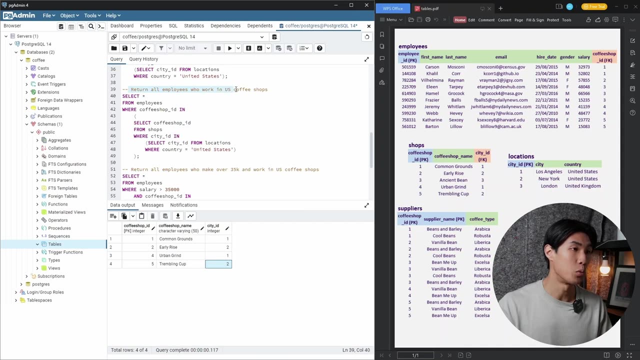 is obviously in the us, and then city id 2 is for the city of new york, which is again in the us. so back into our queries we can return all of the employees who work in us coffee shops. so we have two sub queries running here. actually, the first one we'll select the city ids from. 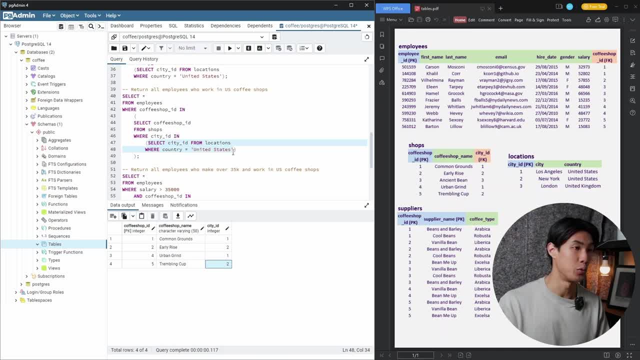 the locations table where the country is equal to united states. and then the second sub query will select the coffee shop id from the shops where the city is. id is in these city ids here. and then i'm just selecting everything from employees where the coffee shop id will be in this coffee shop id here. so that's two sub queries here. so let me just run. 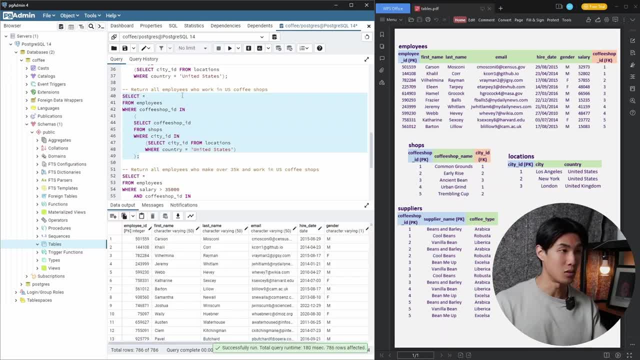 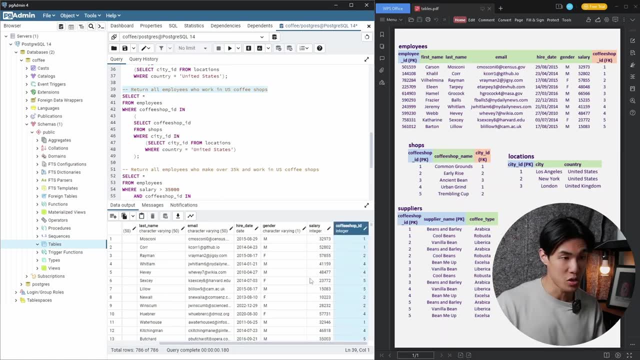 this code here and you can see that now we've selected all of the employees work in us coffee shops and we can check that quickly. so let me go into my table and if i click into the coffee shop id column here you can see that coffee shop id one, two, four, five. so you see basically everything. 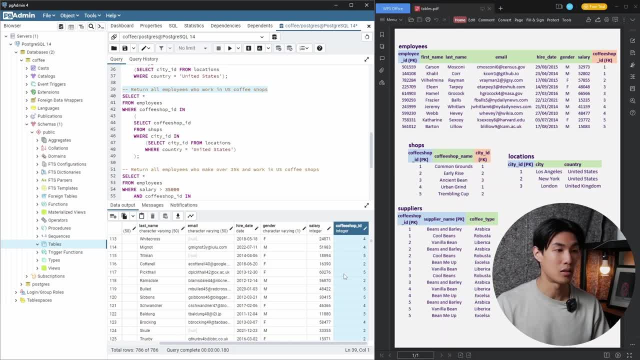 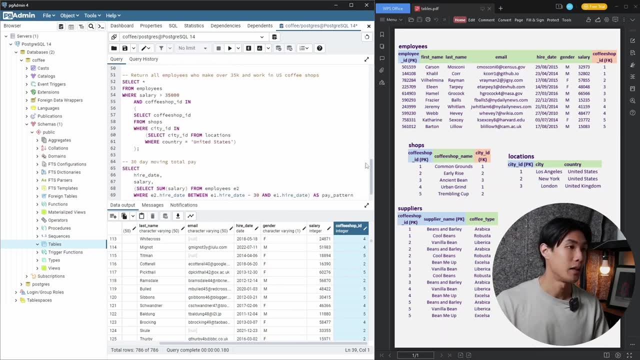 but three appears, because three is the only coffee shop that's not in the us because it's in london, which is in the united kingdom now, next up, how about we return all of the employees who make over 35 000 and work in us coffee shops? so the only difference now is that obviously i included 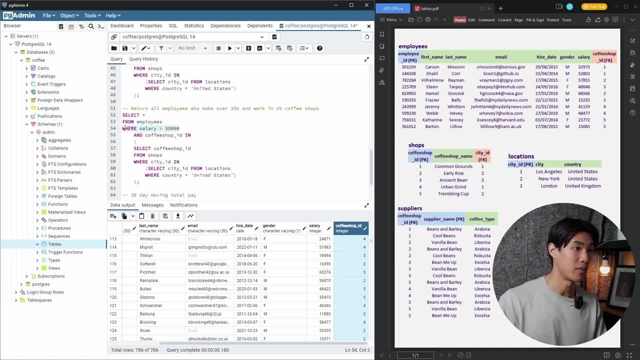 a work clause here, so where the salary is greater than 35 000 and work in us coffee shops. so the only difference now is that obviously i included a 35,000 and the coffee shop ID is in this coffee shop ID here that we defined using two sub. 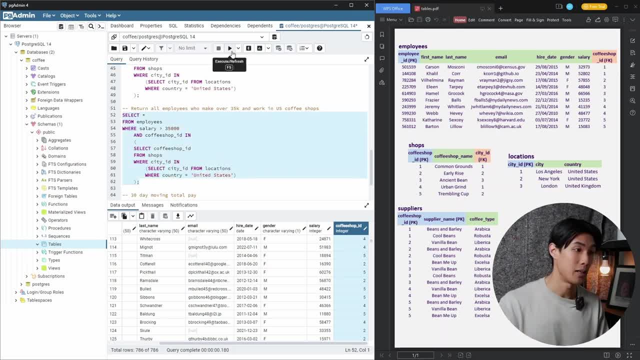 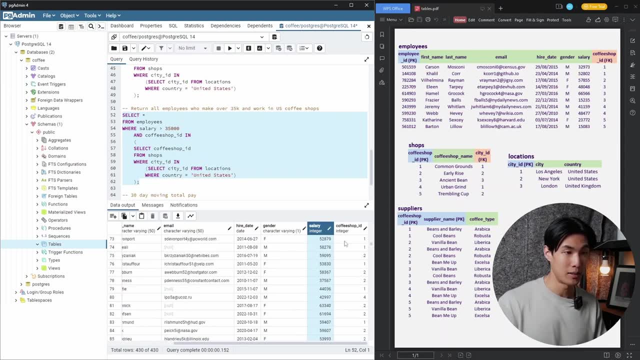 queries. So if I run this now, I am going to have all of the employees who make over 35,000.. So let's look into the salary column. Yep, That looks right. And then in the coffee shop ID column, again you don't see number three appear. 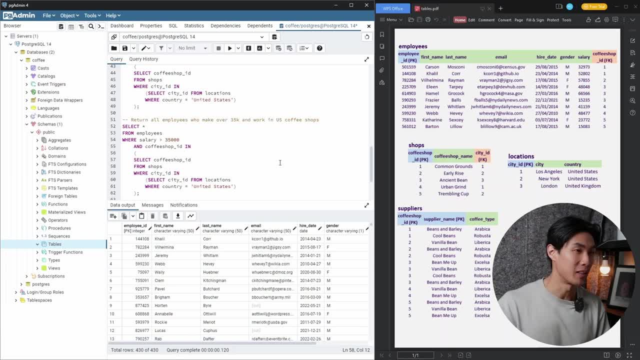 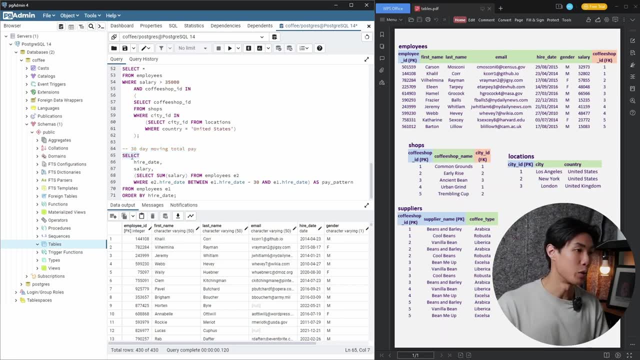 Okay, Last but not least, let's do something quite complicated. So how about we do a 30 day moving total pay? So this time we're selecting the hire date and then the salary columns from employees E1, and then we are going to use the employees table again. 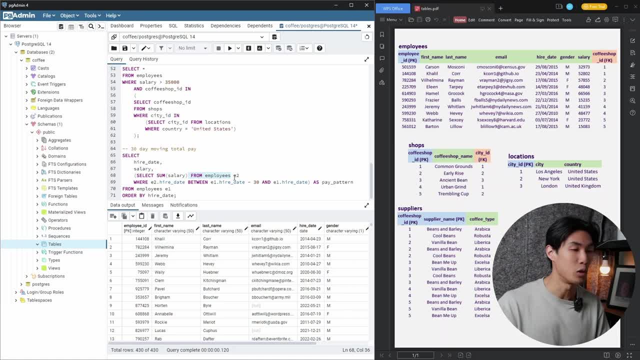 So we're selecting the sum of the salaries from the employees table. I'm going to alias this as E2, where the E2 hire date, So where the hire date within this query here is between the E1 and E2.. Employees table: hire date minus 30, because we want the 30 day moving average. 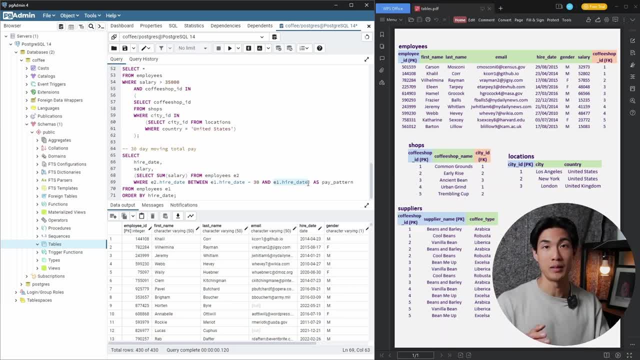 And obviously between the E1 dot hire date, because basically we just want the values before 30 days from the current date to the current date And I am going to say this column is called pay pattern And then I am going to order by the hire date. 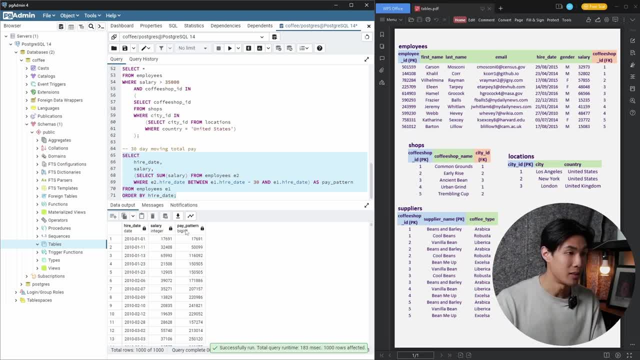 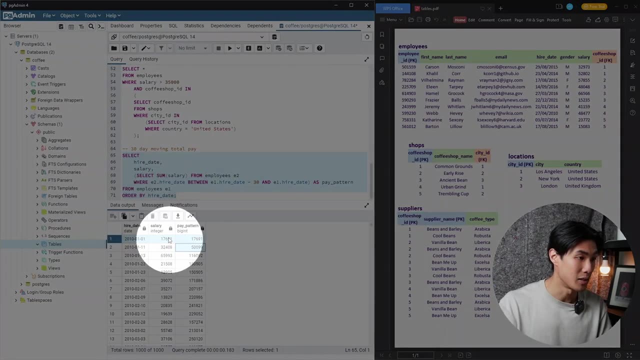 So let me just run this query here And you can see now that if I look down the pay pattern column here, you can see that first of all we have 17,000.. 691.. And then our second observation here is 50,000 and 99,, which is 17,691 plus 32,408.. 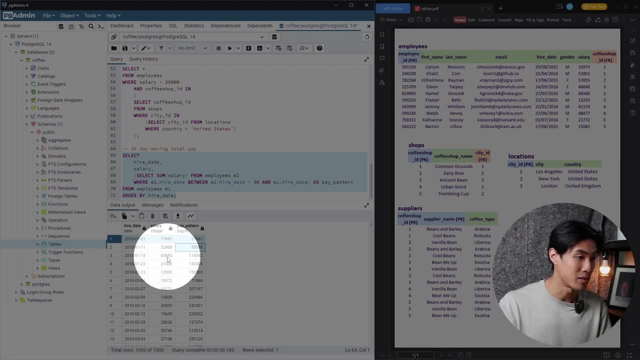 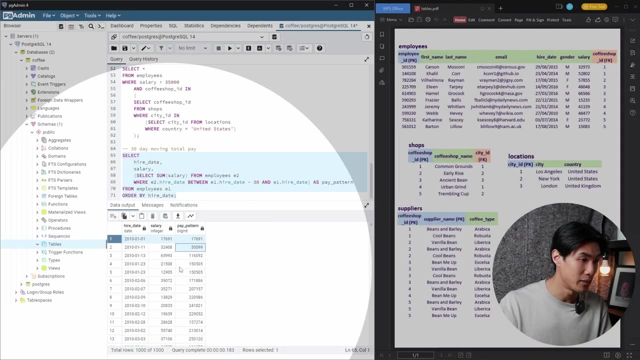 And then 50,000 and 99 plus 65,993 is equal to one 16, Oh nine two. one 16, Oh nine two plus 21,. five Oh eight is equal to 15, one. 50, five Oh five. 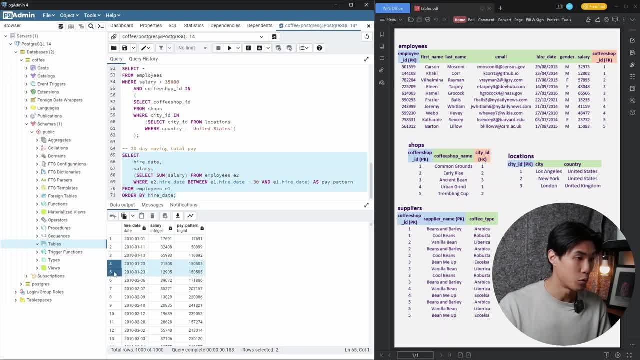 And you see how these are on the same date. So row four And row five, it's the same date, 23rd of January. So the values will be exactly the same. Now for the next row, row six. here you can see that the value now is 171,886.. 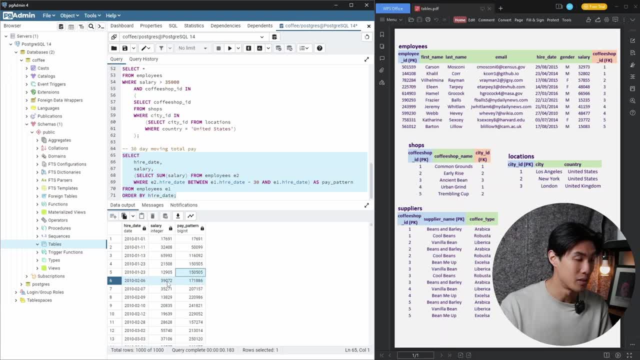 So it's not exactly equal to one five Oh five, plus the 39, Oh seven two. This is because this is already the 6th of February, So this is going to take all of the salaries between the 6th of January and the 6th of. 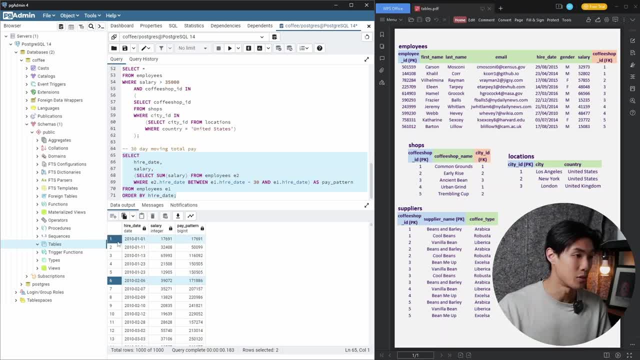 February. So it's going to exclude row number one here. So essentially, this row six adds up all of these values are row two, row three, row four, row five and row six, And this is how we get to 171,886.. 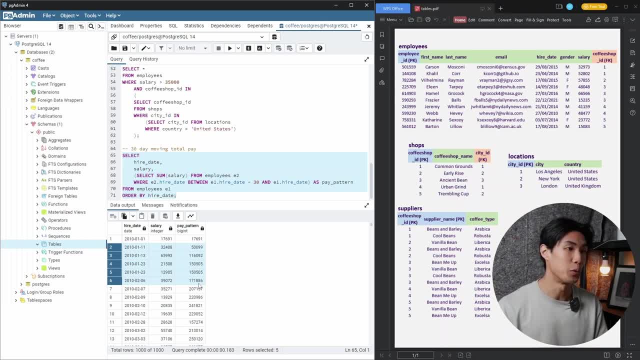 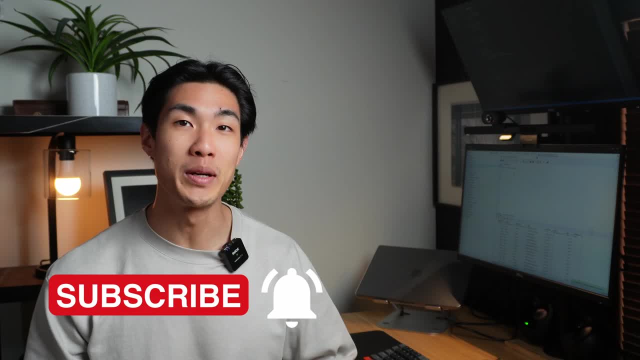 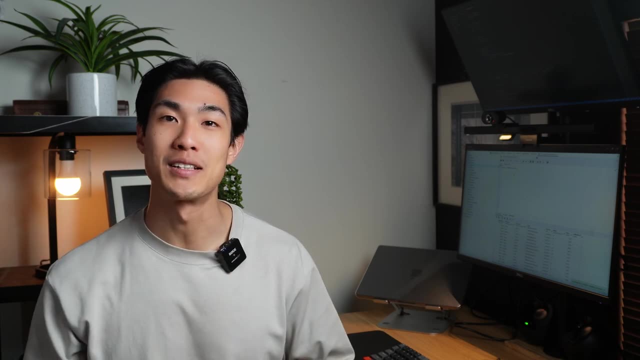 So this is how you do a 30 day moving total pay, And that's it. That is the end of the tutorial. If you liked this video and took away something from it, you may like some of my other videos right here. Thank you so, so much for watching, and I'll see you in the next one. Bye, Bye. 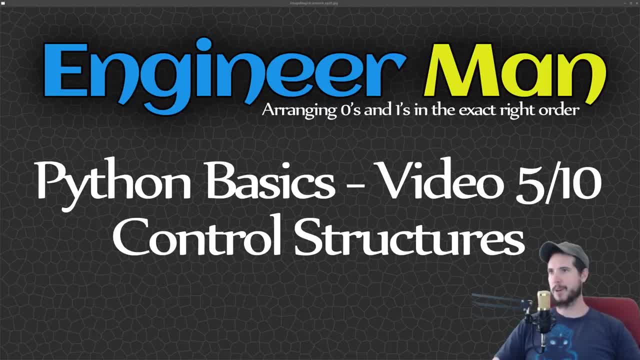 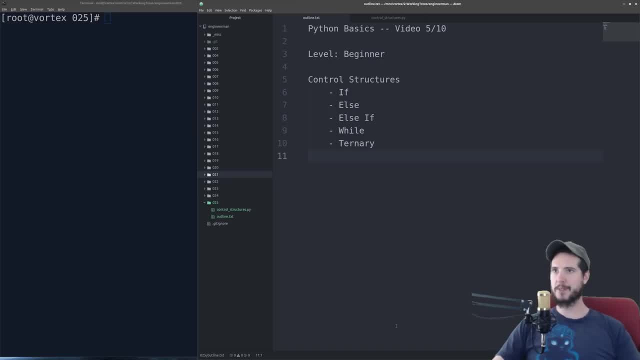 What's going on? engineer team. This is video 5 of 10 in my Python Basics video series. In this video, we're talking about control structures. As with every video in the series, the level's beginner. In this video we'll talk about the if construct, else else if, while and the ternary.